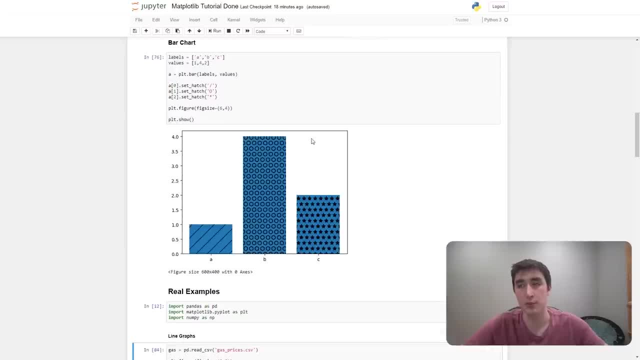 video off with going through all sorts of like real world examples where you can kind of combine your data science skills that you might have using like panda's library. and if you haven't learned anything about the panda's library, i recommend you watch my video on that. so with that, the kind 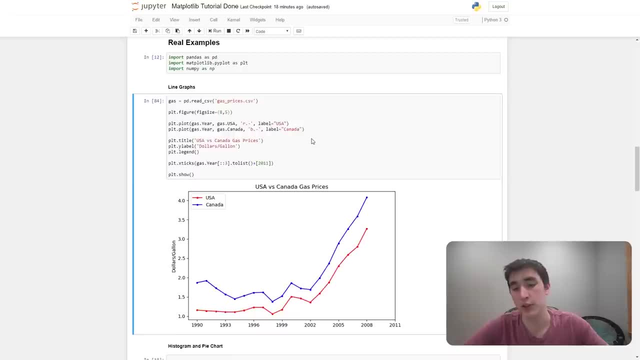 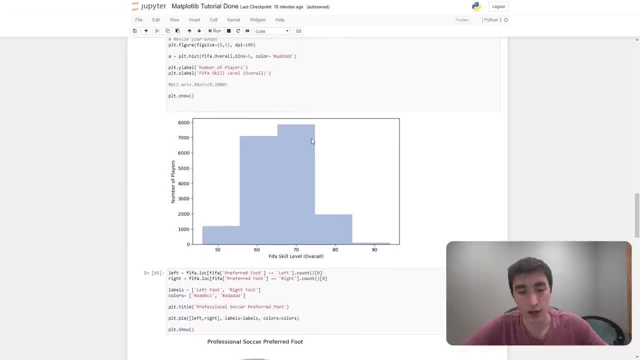 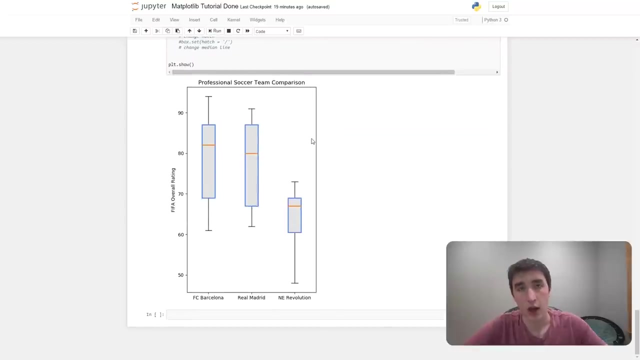 of the real world examples. we'll do stuff such as like plot the usa versus canada gas prices off of a data that we have that i'll link to in a csv. we'll do some histogram stuff. we'll do some pie chart stuff and we will do some box and whiskers chart stuff. i can't get through. 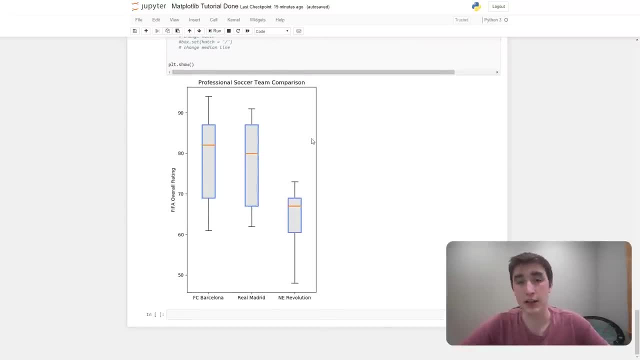 type of graph in this one video. but if there's certain things that i didn't cover and you really want me to cover, let me know in the comments. that would be super duper. uh yeah, that's all i got to start this video. let's just jump into it. all right, let's start out by loading in the libraries that. 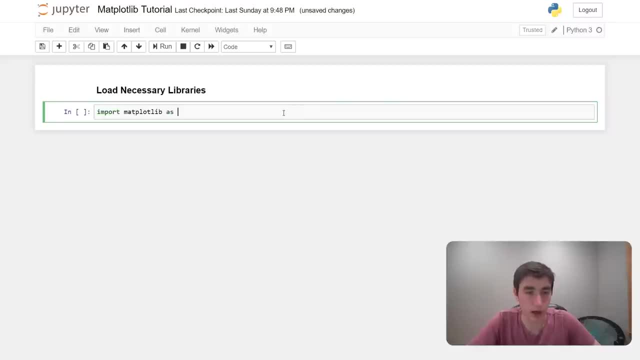 we need for this tutorial. so we're going to import matplotlib as our dot pi plot as plt, we're going to import numpy as np and we're going to the later examples: import pandas as pd and run that. and so if you have all these, uh like already, 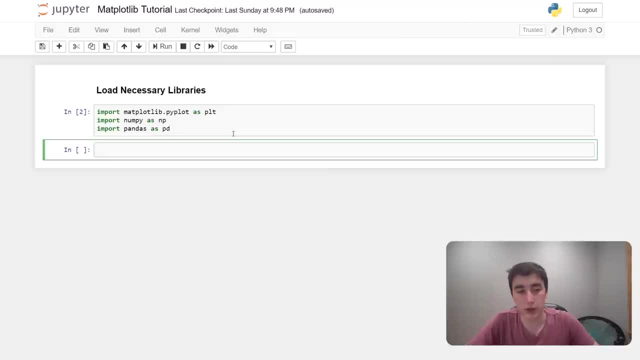 installed, you won't get any errors. if you do get these get an error when you're trying to run one of these, you probably need to install it. so you can either do a pip install matplotlib, pip install numpy, pip install pandas, or you can install a python distribution that already has these packages. 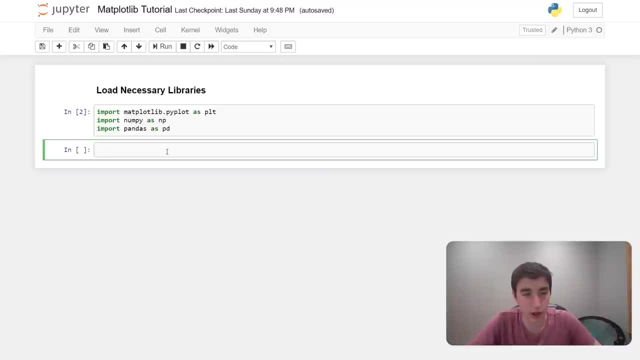 such as anaconda. i'll link to how to do this in the description. okay, so now we have our libraries loaded, let's now build our basic graph. so i always think it's kind of the hardest part about anything with python in general is starting with that blank, blank space. so what i recommend for matplotlib is always start at the documentation. 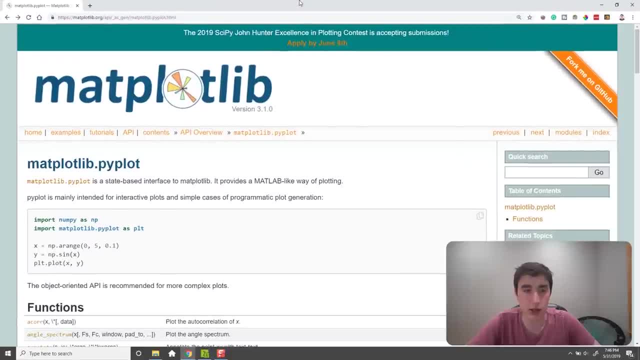 so i have a link for this in the description. but here is the home page of the matplotlibpiplot documentation and what i recommend is, whenever we're trying to do something new, just do a control f and like look for it. so if we look for plot here, that's like we're just trying to get a line graph on the on the screen, uh box. 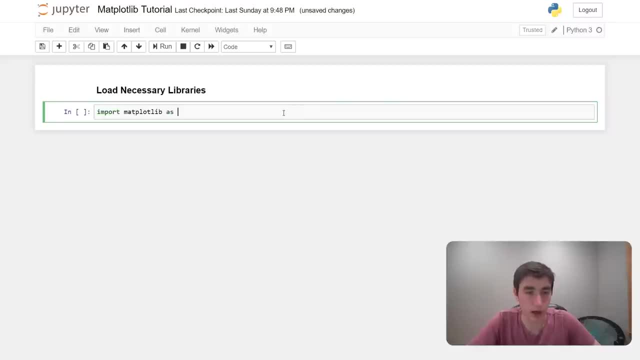 we need for this tutorial. so we're going to import matplotlib as our dot pi plot as plt, we're going to import numpy as np and we're going to the later examples: import pandas as pd and run that. and so if you have all these, uh like already, 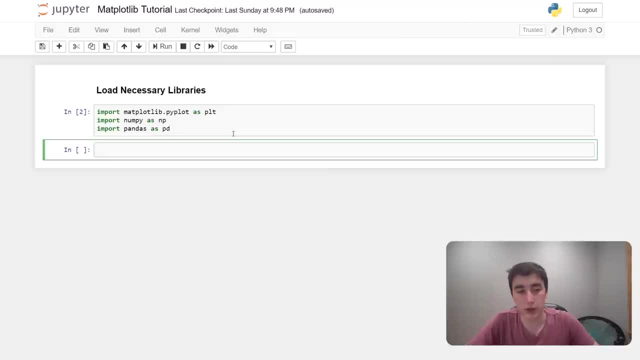 installed, you won't get any errors. if you do get these get an error when you're trying to run one of these, you probably need to install it. so you can either do a pip install matplotlib, pip install numpy, pip install pandas, or you can install a python distribution that already has these packages. 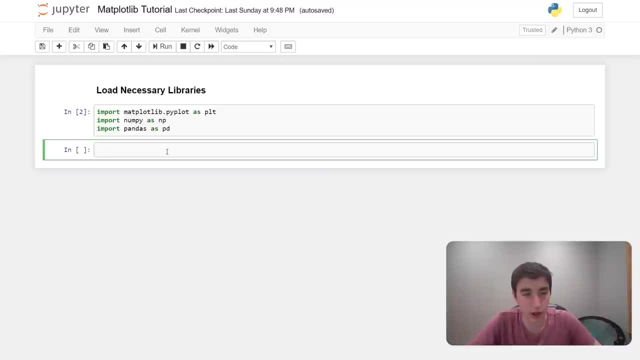 such as anaconda. i'll link to how to do this in the description. okay, so now we have our libraries loaded, let's now build our basic graph. so i always think it's kind of the hardest part about anything with python in general is starting with that blank, blank space. so what i recommend for matplotlib is always start at the documentation. 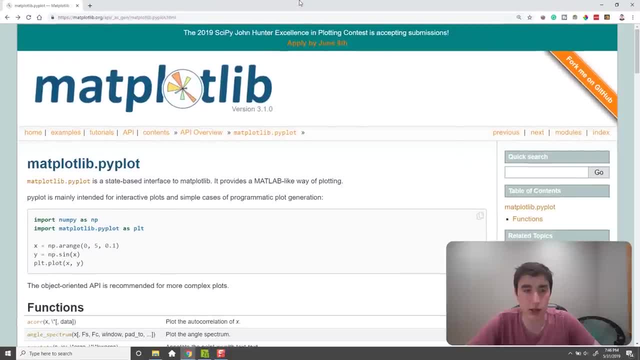 so i have a link for this in the description. but here is the home page of the matplotlibpiplot documentation and what i recommend is, whenever we're trying to do something new, just do a ctrl f and like, look for it. so if we look for plot here, that's like we're just trying to get a line graph on the on the screen- uh, box plots now. 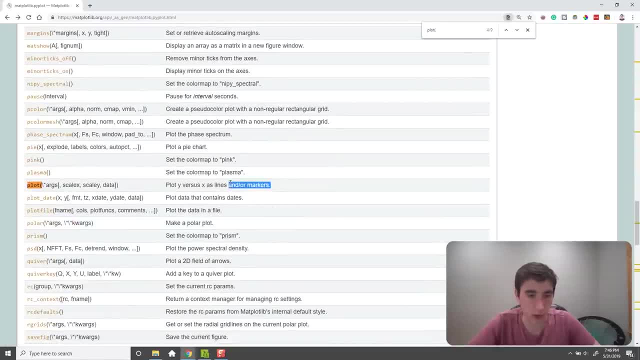 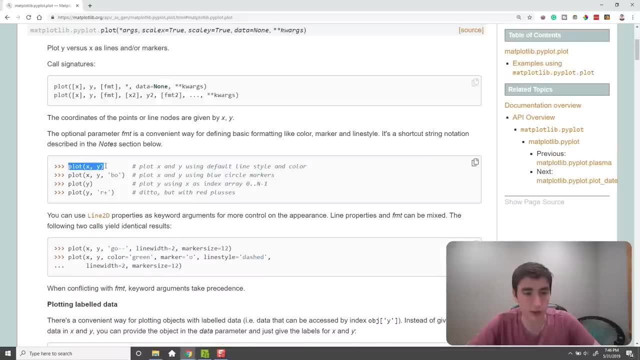 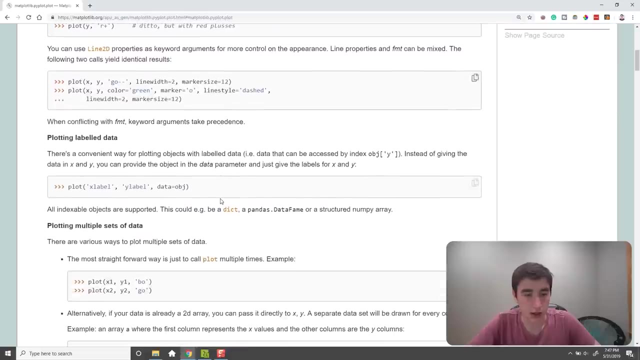 we want, we don't want it. then plot- okay, this looks good. uh, plot y versus x as lines or markers. so this is what we'll start off by doing. as you can see right here in the examples, it gives: gives plot x, comma y. so that's the command we'll have to run to make this work. uh, and just to know, 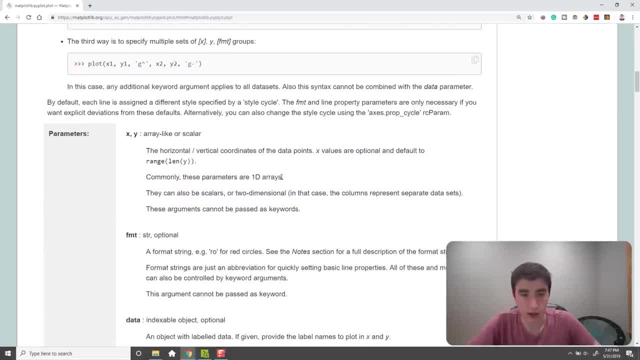 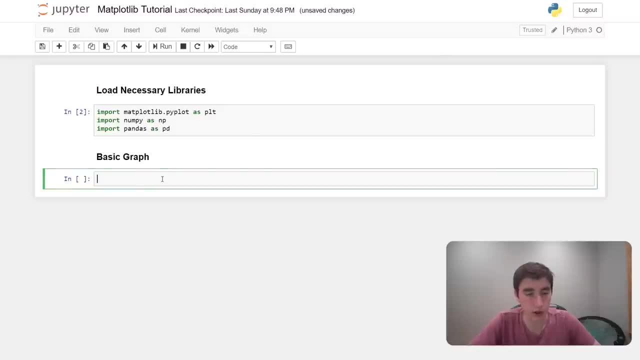 what we're going to need to do is we're going to need to pass in the x and y are. if we go down to parameters, they tell us that commonly these parameters are 1d arrays. so we know we need to pass in 1d array to the plot function. so if we do plot one, two, three, that's going to be our x and 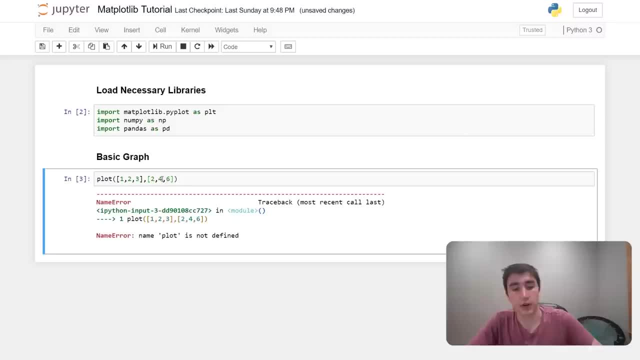 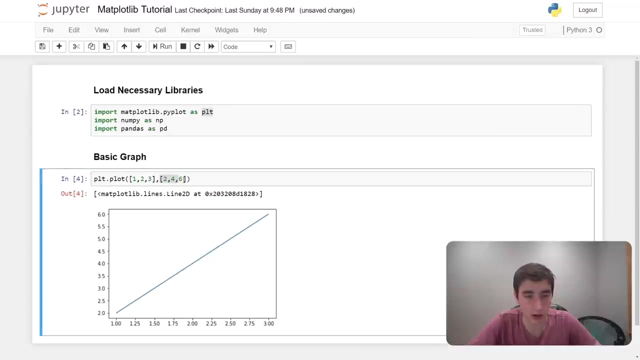 two, four, six will be our y. i can't type and run that. so when we run this function we actually have to do plt, dot, plot, and then this is our x and the second array is our y. so let's see what happens there. yay, we get a graph and, to clean this up, a 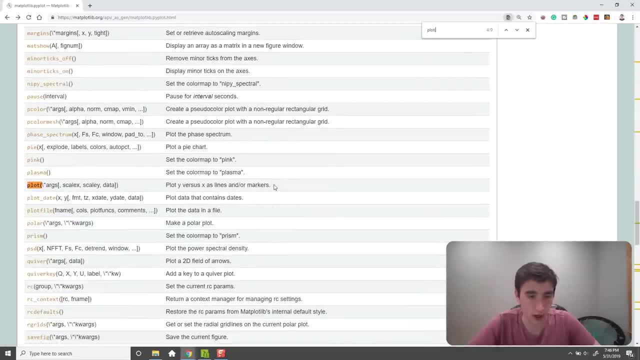 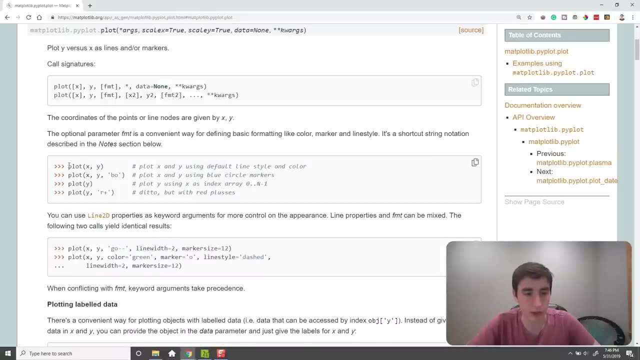 plot is not the one, we don't want it then plot: okay, this looks good. uh, plot y versus x as lines or markers. so this is what we'll start off by doing. as you can see right here in the examples, it gives: gives plot x, comma y. so that's the command we'll have to run to make this work. 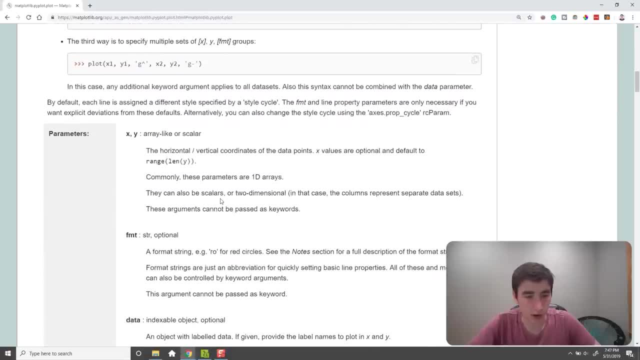 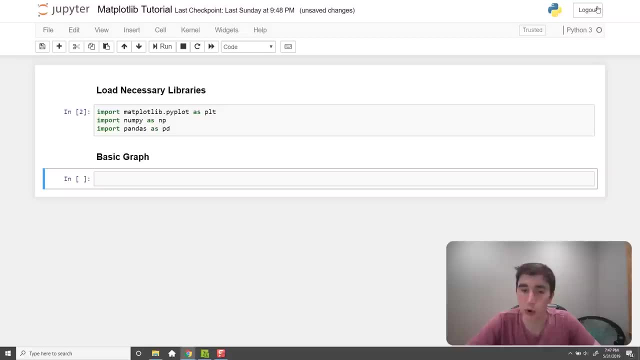 and just to know what x and y are. if we go down to parameters, they tell us that commonly these parameters are 1d arrays. so we know we need to pass in 1d array to the plot function. so if we do plot 1, 2, 3, that's going to be our X and 2, 4, 6. 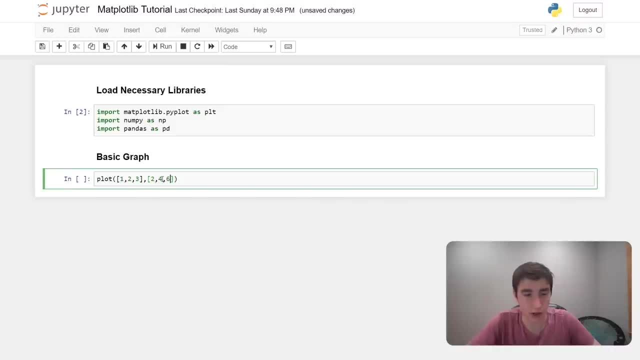 will be our Y. I can't type and run. that plot is not defined, so we imported pyplot as plot. so when we run this function we actually have to do pltplot, and then this is our X and the second array is our Y. so let's see what happens. 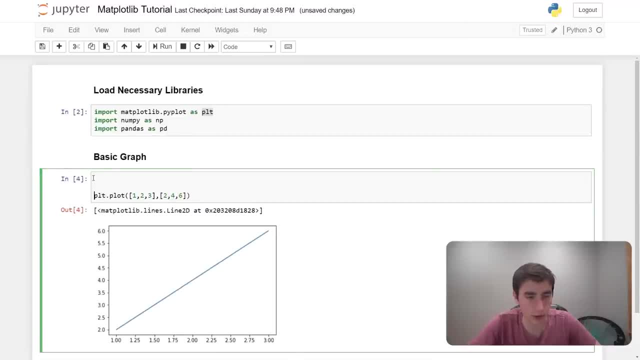 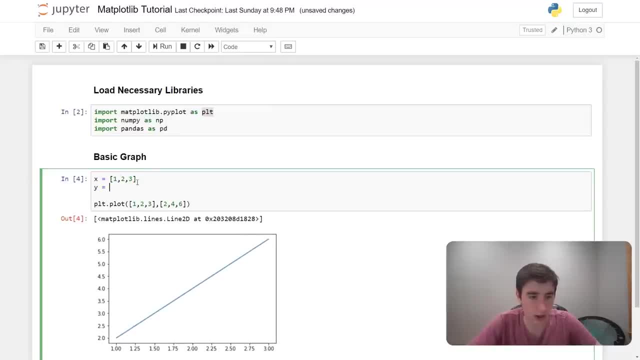 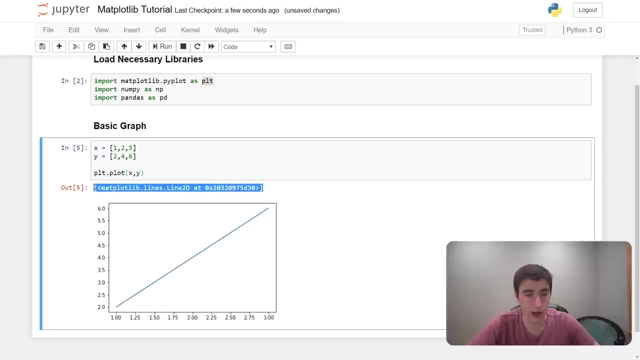 so X is 1, 2, 3 and Y is 2, 4, 6, and we can change now this to X, Y. and one thing that's annoying with the matplotlib- if you're doing this in Jupyter notebook by default- is you have this annoying little line here, so you want to get rid of that. 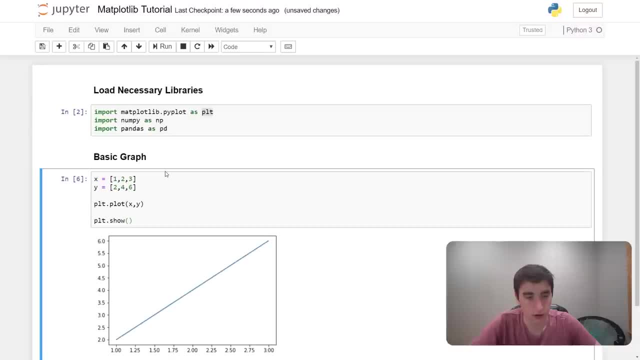 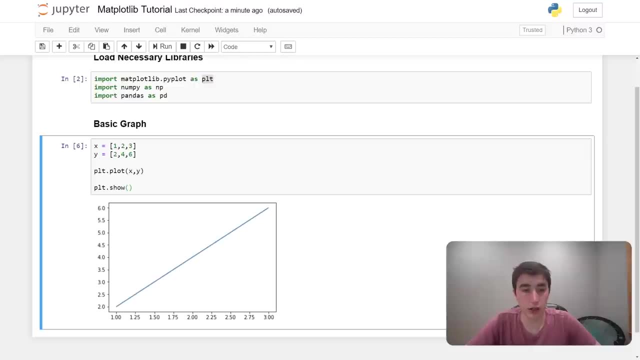 you can just actually call plot dot show, and that's the correct way to actually show this graph. okay, now that we have just a line on the screen, let's start adding a little bit more to our graph. so to do this, let's go back to our documentation and 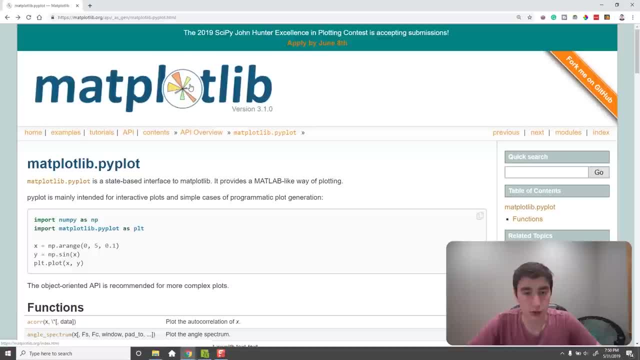 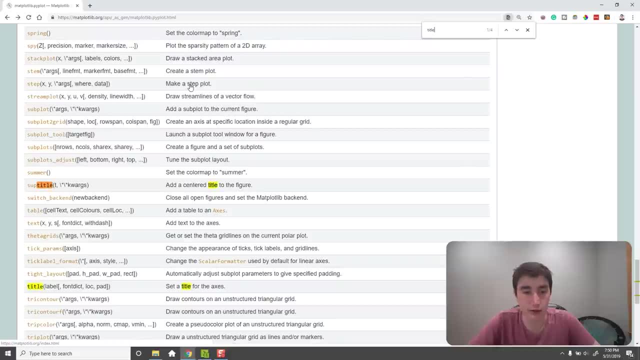 go back to just the pie plot. so I think this is a good spot to start, because you always can kind of just control left and find something you're looking for. so let's say we wanted to add a title to our graph. if I type in title, it points. 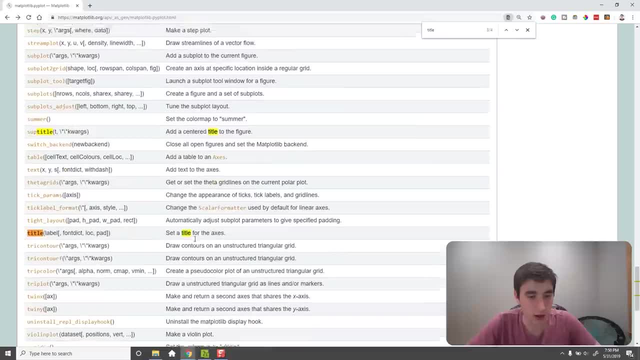 me right to a couple different places that I probably want to look at, and right here is what we're looking at and that's where we're going to add our graph, so I'm going to go to the plot and choose the size of the graph that we're. 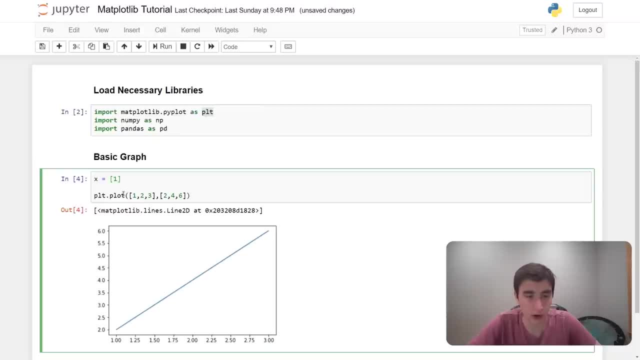 little bit. i recommend um moving our variables into, or moving our arrays into variables. so x is one, two, three and y is two, four, six, and we can change that now this to x, y. and one thing that's annoying with the matplotlib, if you're doing this in: 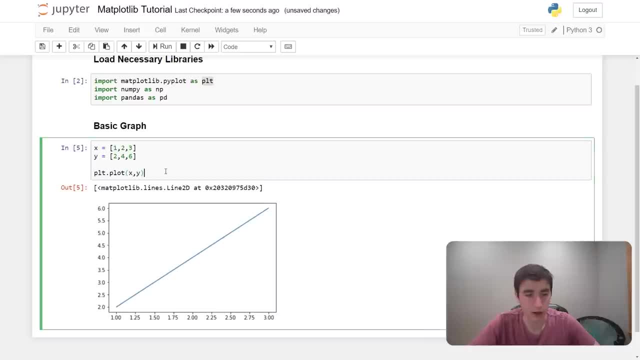 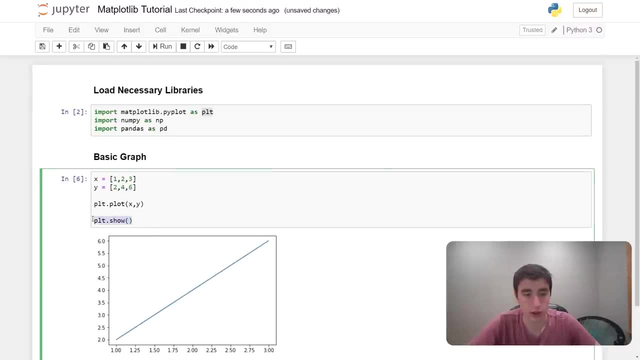 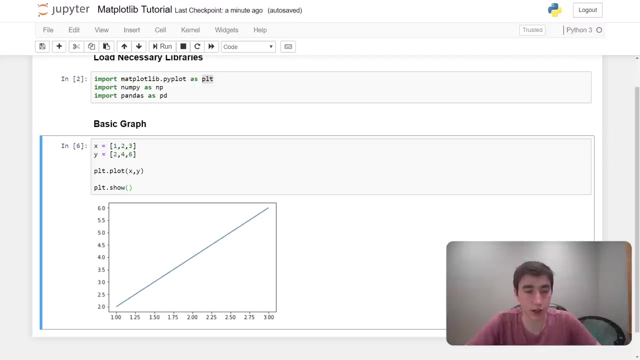 jupyter notebook by default is: you have this annoying little line here, so you want to get rid of that? you can just actually call plot dot show, and that's the correct way to actually show this graph. okay, now that we have just a line on the screen, let's uh start adding a little. 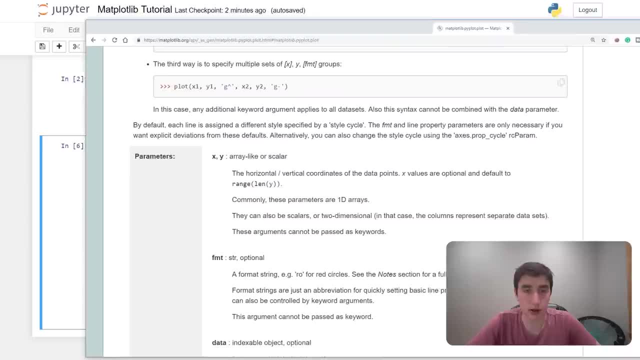 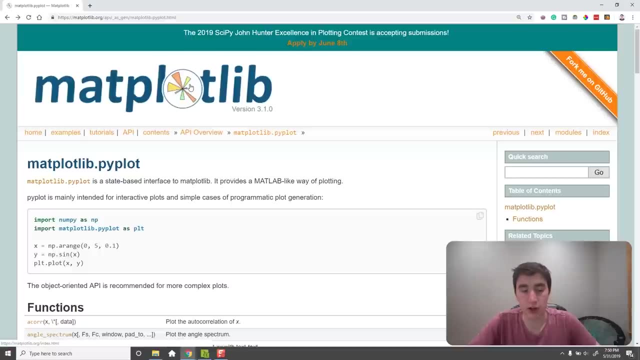 bit more to our graph. so to do this, let's go back to our documentation and go back to just the pi plot. so i think this is a good spot to start, because you always can kind of just control f and find something you're looking for. so let's say we wanted to add a title. 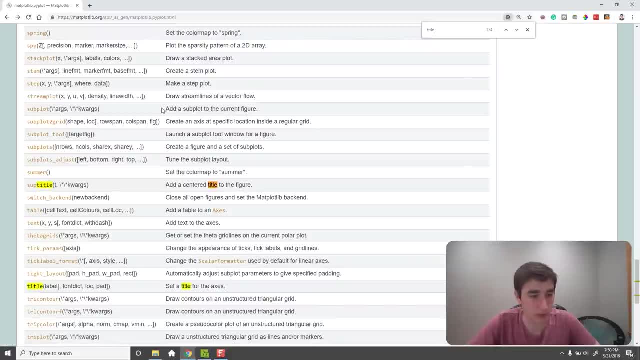 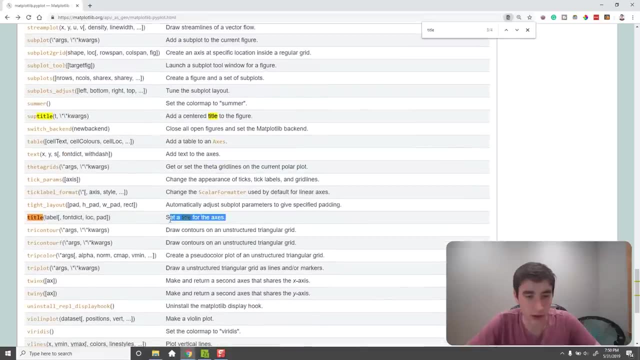 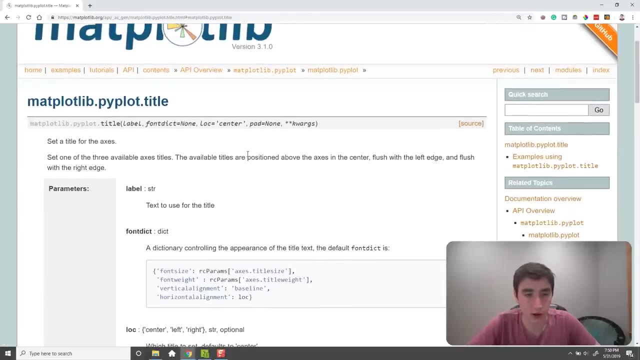 to our graph. if i type in title, it points me right to a couple different places that i probably want to look at, and right here is what we're looking for. so set a title for the axes, click that, and this tells me all sorts of stuff about how i call this, so it looks like i can just. 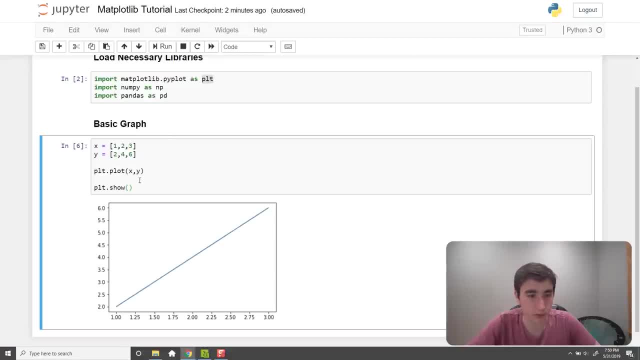 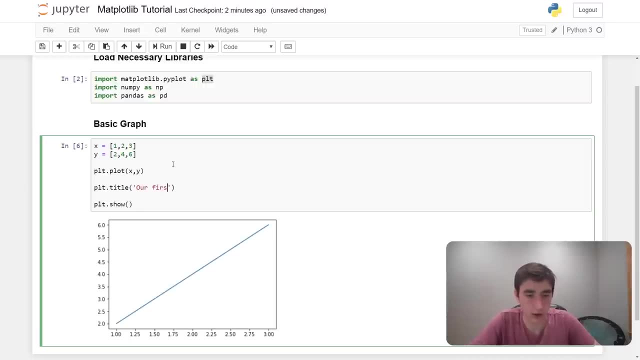 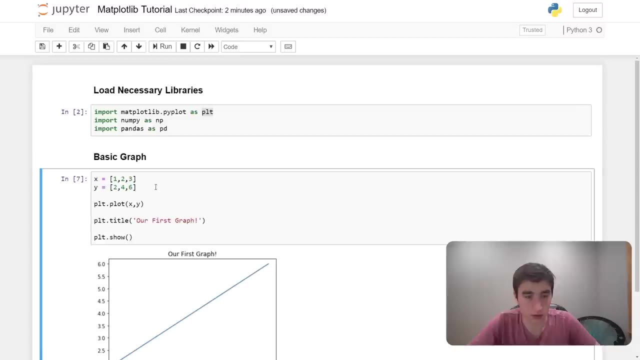 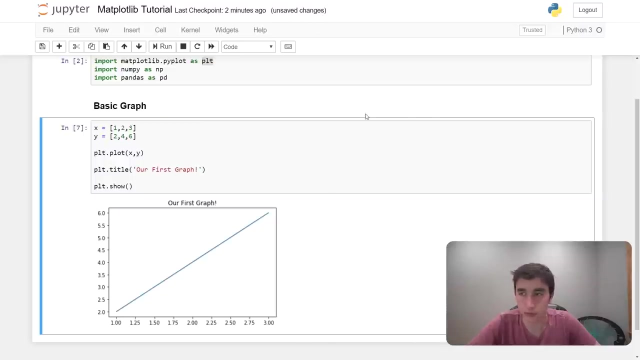 do piplottitle. so i can do plot dot title and let's just do our first graph and run that. as you can see, our title is now there, and same thing for a lot of the different parameters. so, going back to the documentation, if i want an after comment for the documentation, if i want, let's say, an after comment, i just do piplottitle. so if you linked id. 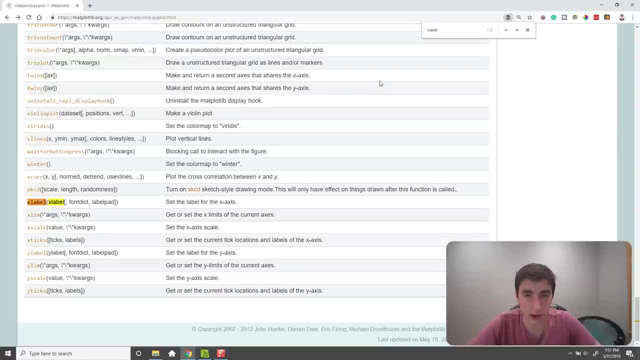 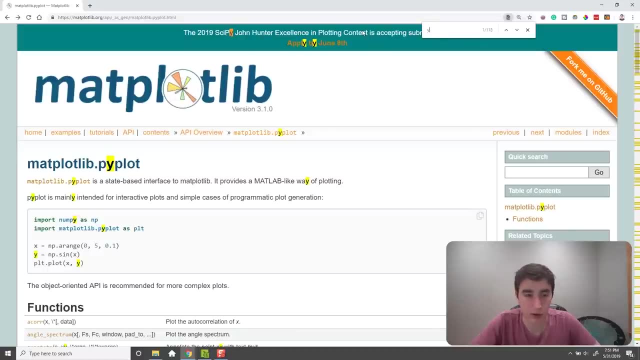 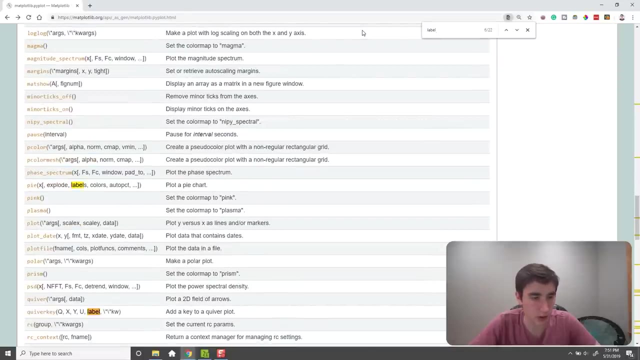 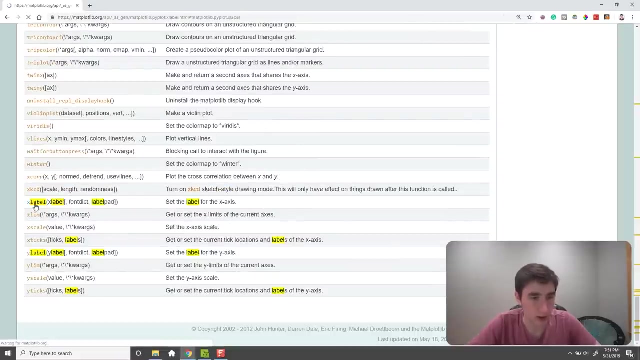 x label and a y label. i just type in right, i guess i knew that. but let's just say y label, nothing comes up y, or just even label c label label a contour plot. that's not us. the fig label is no pi, no title, no x label, y label. that's how we get there, so you can keep. 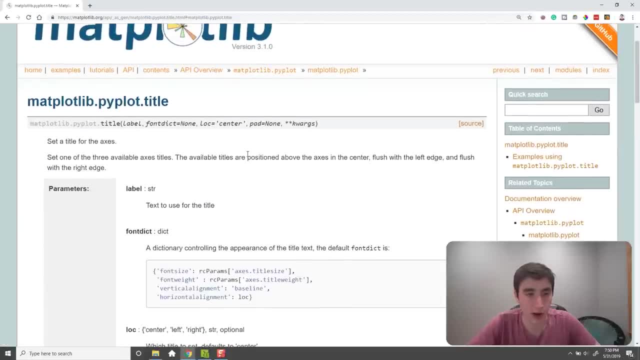 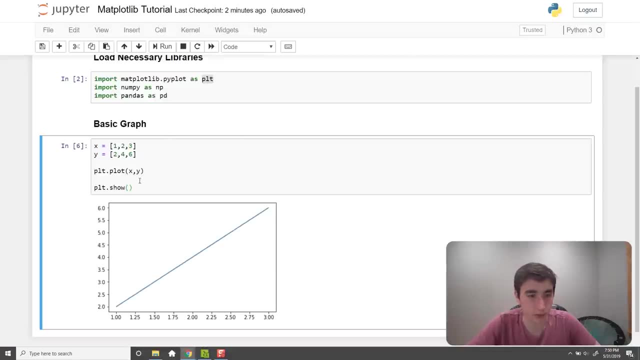 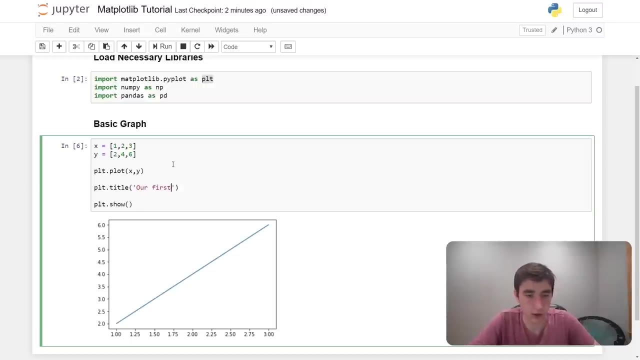 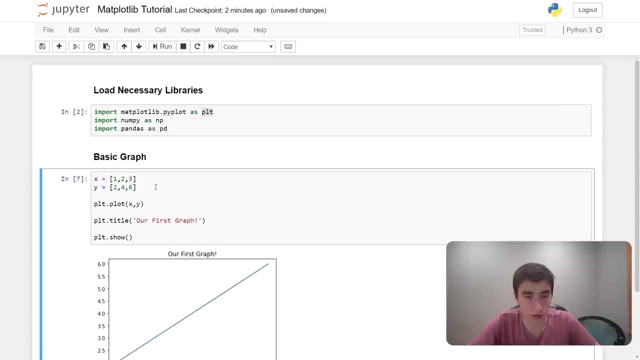 looking for. so set a title for the axes, click that and this tells me all sorts of stuff about how I call this. so it looks like I need to pie plot title. so I can do plot title and let's just do our first graph and run that. as you can see, our title is now there, and same thing for a lot of. 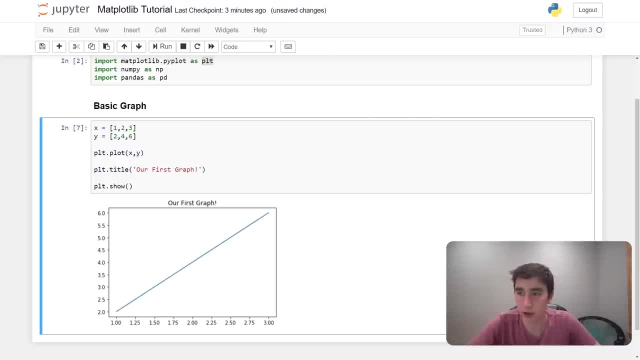 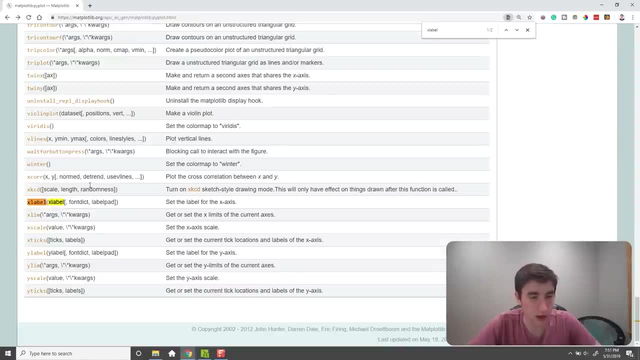 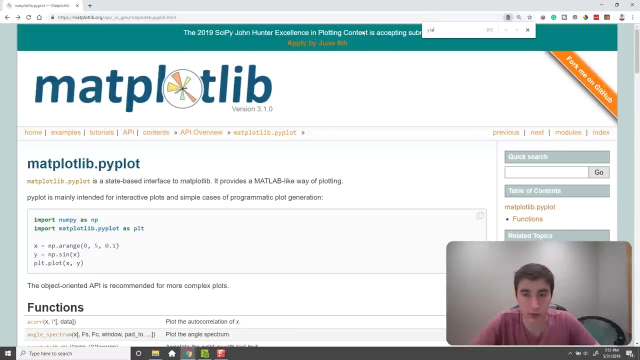 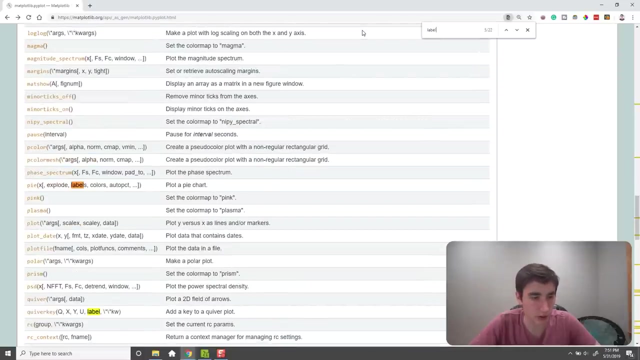 the different parameters. so, going back to the documentation, if I want an X label on a Y label, I just type in: alright, I guess I knew that. but let's just say why label nothing comes up, why. or just even label C, label label a contour plot. that's not us. the Fig Label is no Pi, no title, no X label. 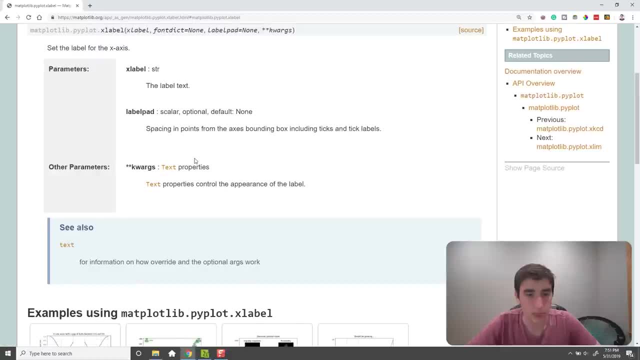 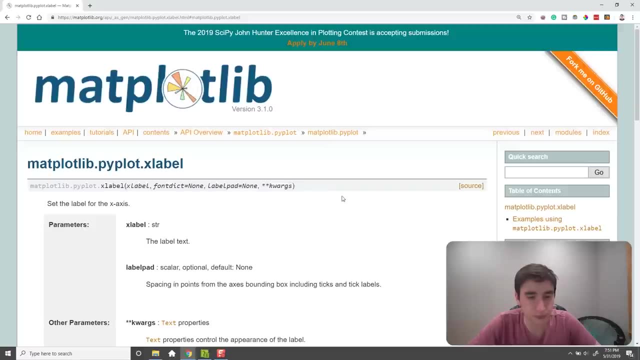 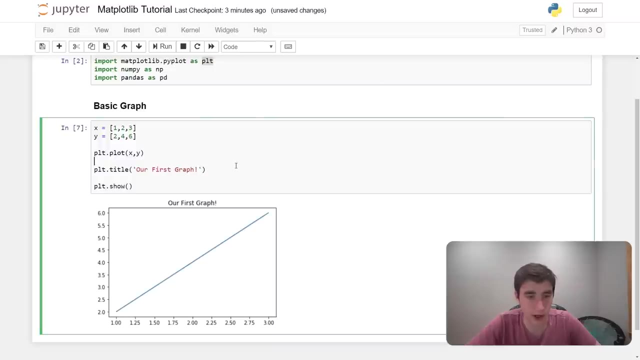 why they'll. that's how we get there, so you can keep doing this and really easily find what you're looking for. I think it's a good place to go if you kind of just if you forget things, because I always forget things in that plot lab. okay, so adding a label to X and Y: plotX'ed label. 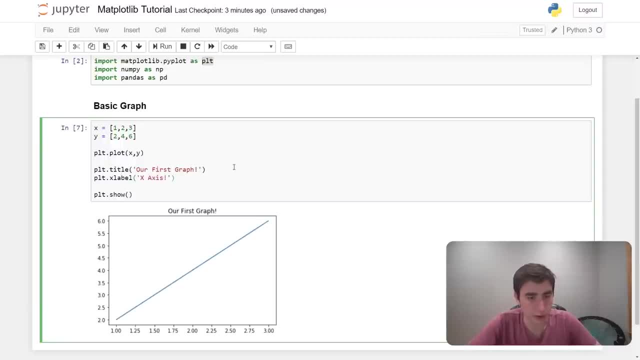 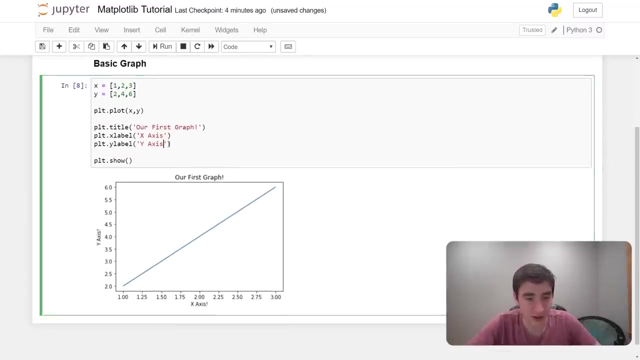 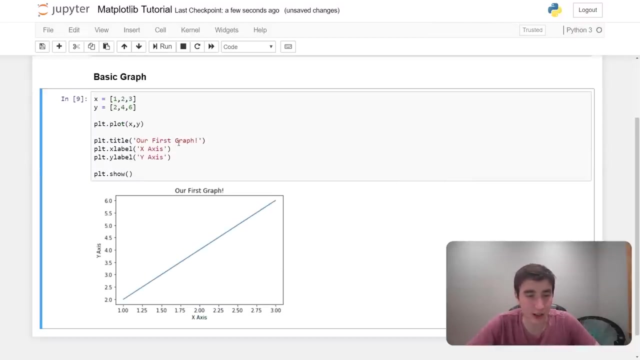 X, X and I'm- I guess I'm- getting really enthusiastic because I keep adding exclamation points to all my stuff: y-axis- yay, see what happens. yeah, and I want to just get rid of these explanations. I don't need them, okay, so now we have a graph and we have a title and we have y-axis, x-axis in a real 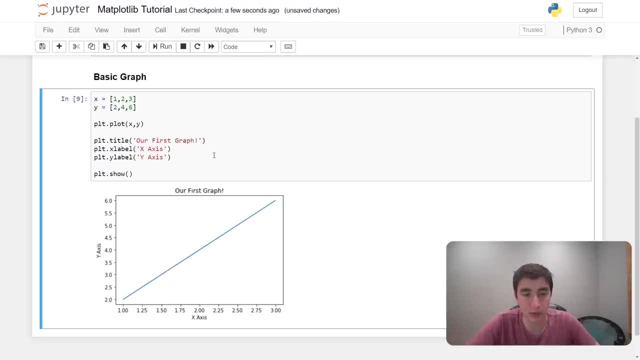 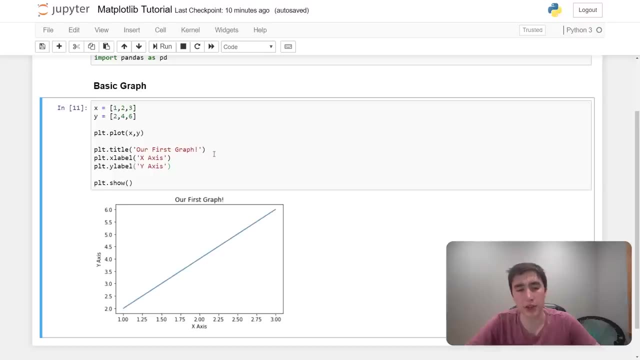 graph, we would label these properly, but for the sake of this example, we're just kind of getting a feel for how we add these. alright, so now that we have our title and labels, one thing we might want to do to them is resize them. so if we 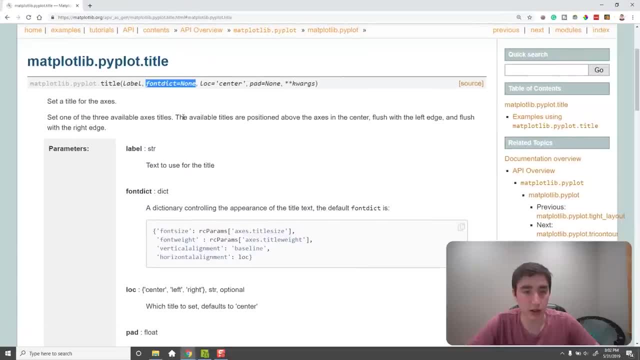 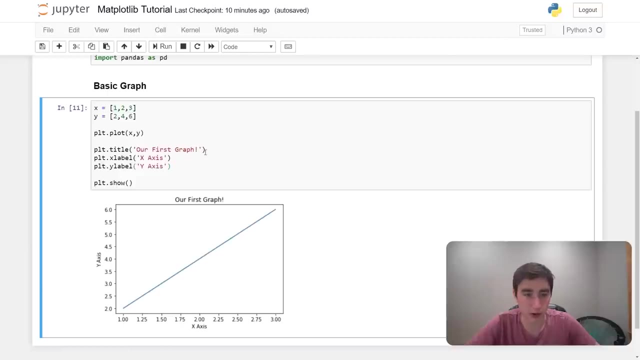 look at the, the documentation for title. one thing you'll notice is that you can use, you can pass in this font dictionary and it gives you a little bit of details about the font dictionary here. but basically there's all sorts of options that we can do and like play around with our font. so let's say I wanted to change. 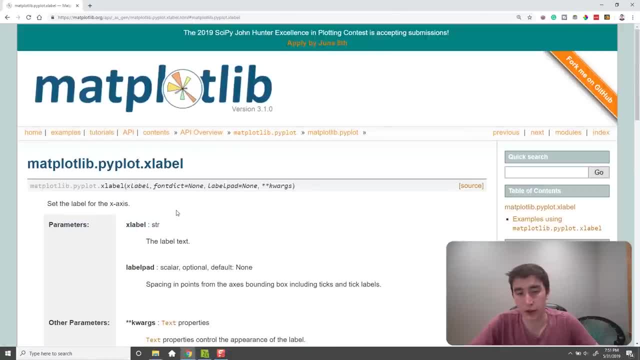 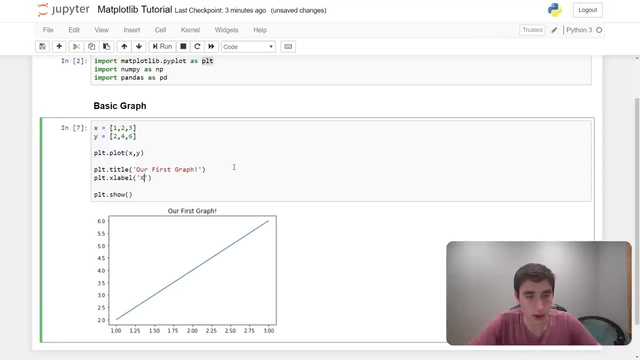 doing this and really easily find what you're looking for. i think it's a good place to go, if you kind of, just if you forget things, because i always forget things from that plot lib. okay, so adding a label to x and y, plot x label, x axes and i'm i guess i'm getting really 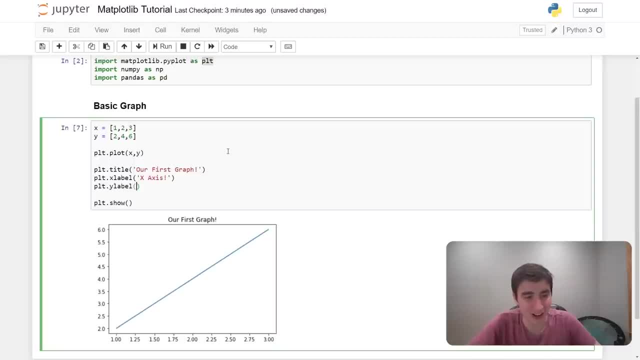 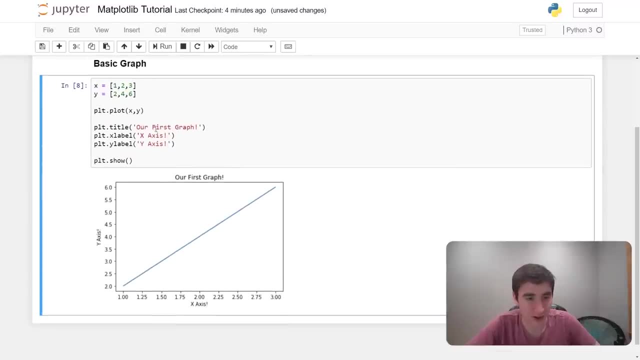 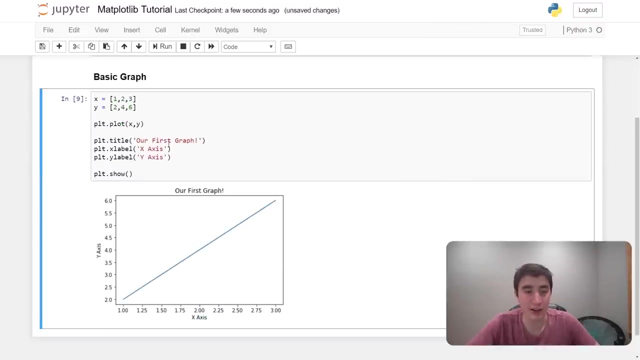 enthusiastic because i keep adding exclamation points to all my stuff. y axes- yay, let's see what happens. Yeah, and I'm going to just get rid of these explanations. I don't need them, Okay, so now we have a graph and we have a title, and we have y-axis, x-axis. 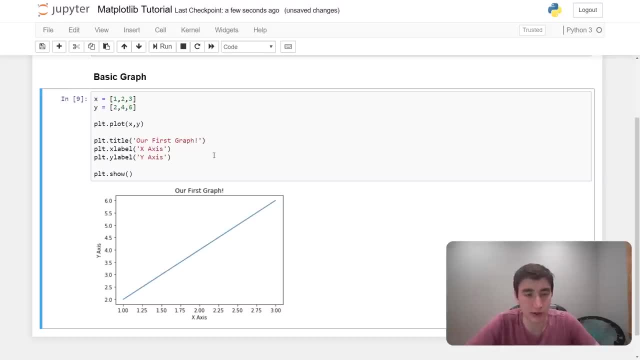 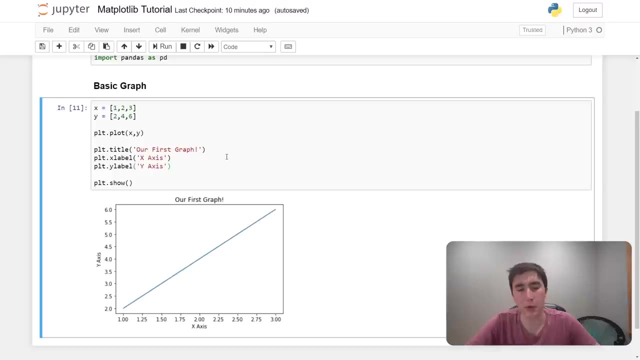 In a real graph we would label these properly, but for the sake of this example, we're just kind of getting a feel for how we add these. All right. so now that we have our title and labels, one thing we might want to do to them is resize them. 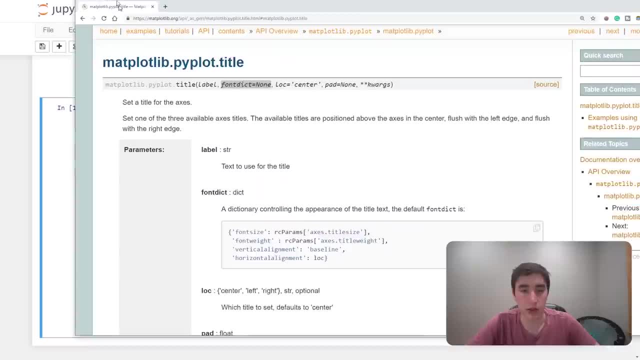 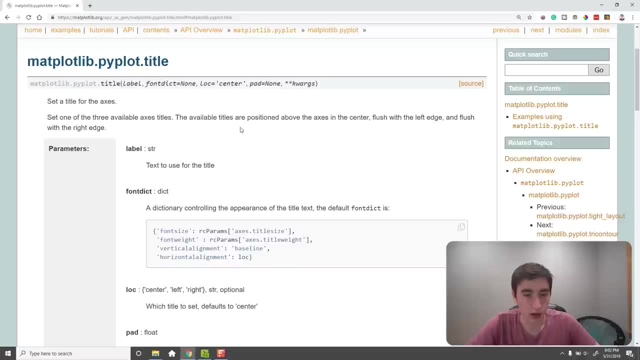 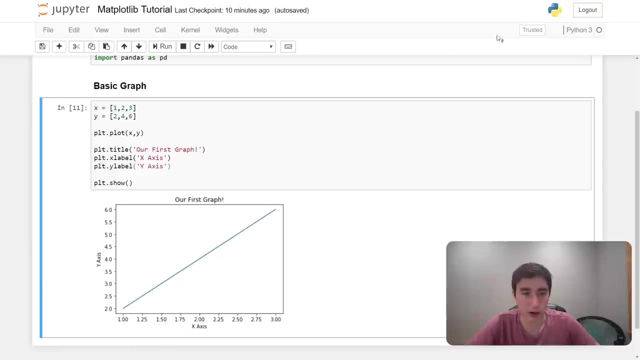 So if we look at the documentation for title, one thing you'll notice is that you can pass in this font dictionary and it gives you a little bit of details about the font dictionary here. But basically there's all sorts of options that we can do and play around with our font. 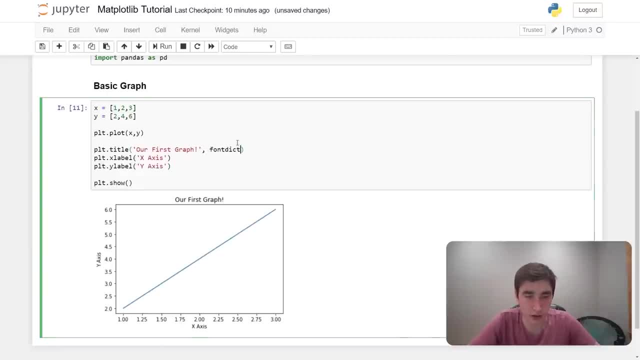 So let's say I wanted to change the font of our title. I can do font dict equals and I can pass in font name. And let's see, Let's say, my good old, trusty, reliable Comic Sans MS will be our new font. 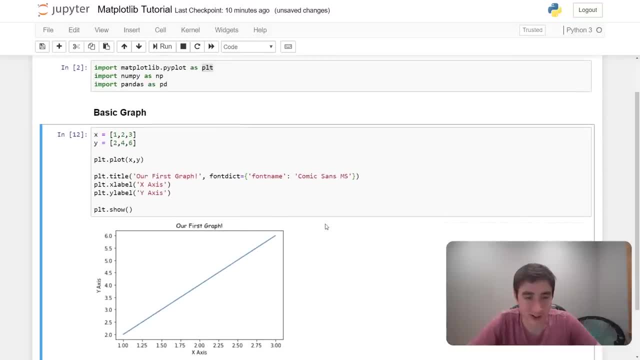 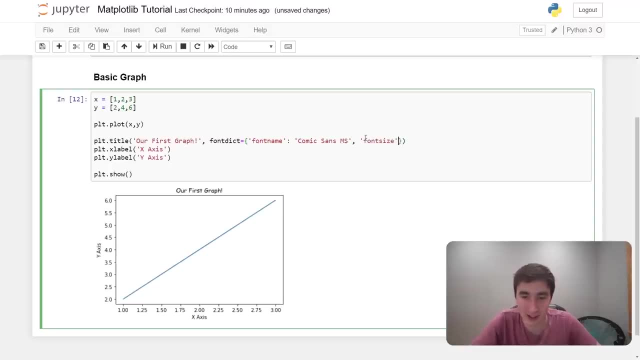 And if you look at that, we got a nice new font on our graph. And if you can't see it, well, then in that case I'll change the font size to be something like 20.. Now you should definitely be able to tell that I've changed the font type. 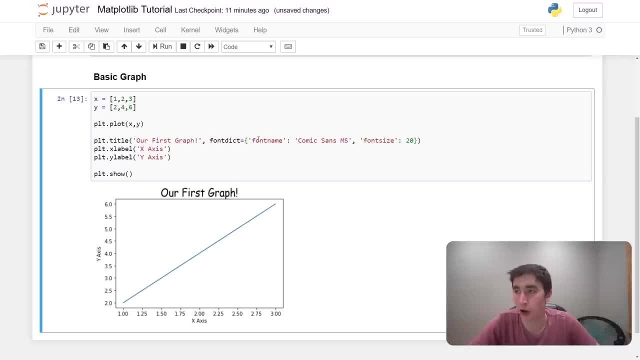 And in the description I listed I put a link to all of the known Matplotlib fonts that you can use, And if you look through the documentation you kind of find some different options. you can do with this, And you can also do the same thing with the labels. 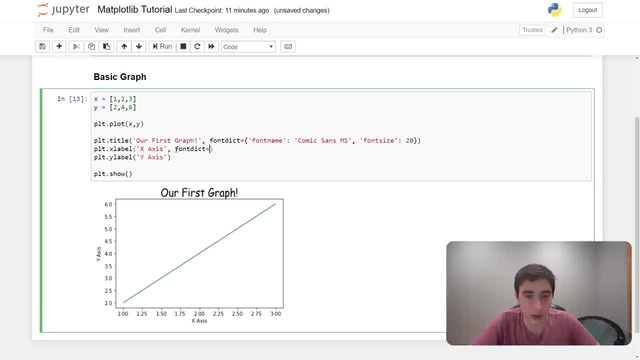 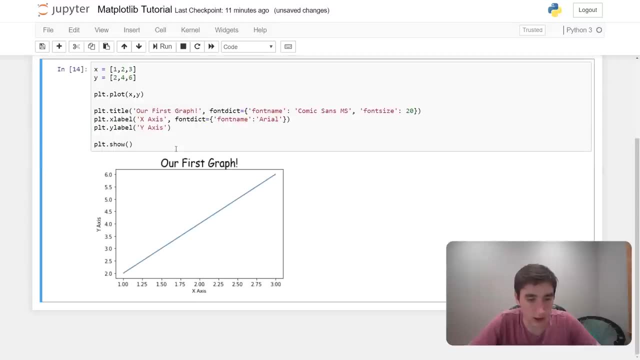 I could do like font dict equals. Let's say, I wanted to make this font REL And that, honestly, might be the default, But if I did it like Comic Sans as well, you can tell that the X-axis now has changed. 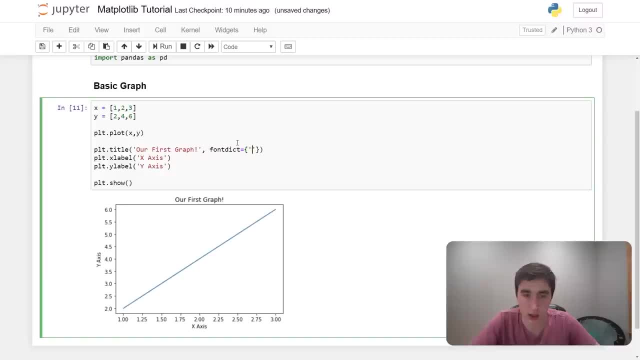 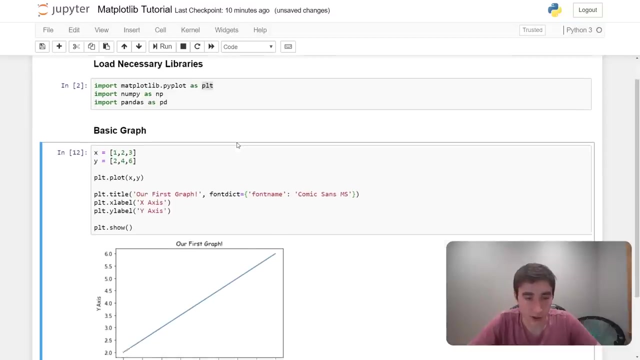 the font, my title, I do you find it equals and I can pass in font name. and let's say, on my good old, trusty, reliable comics sans MS will be our new font, and if you look at that, we got a nice new font on our graph. and if you can't see it, well then, 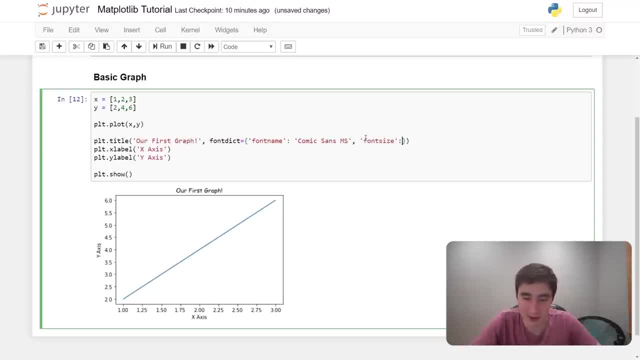 in that case I'll change the font size to be something like 20, and if you can't see it well, then in that case I'll change the font size to be something like 20. Now you should definitely be able to tell that I've changed the font type. 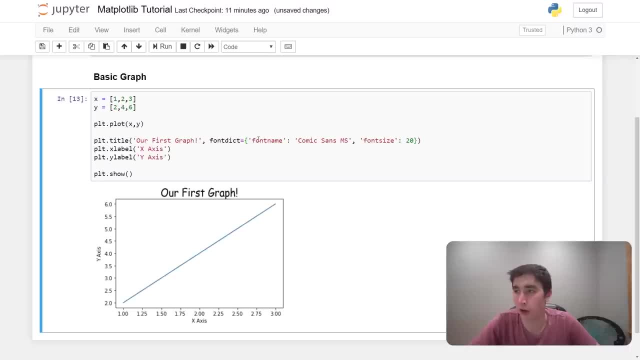 And in the description I put a link to all the known Matplotlib fonts that you can use, And if you look through the documentation you kind of find some different options. you can do with this, And you can also do the same thing with the labels. 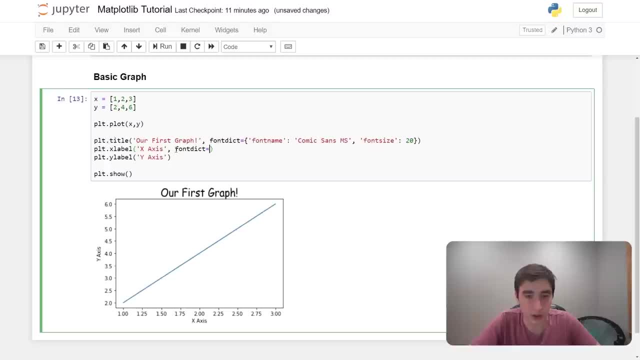 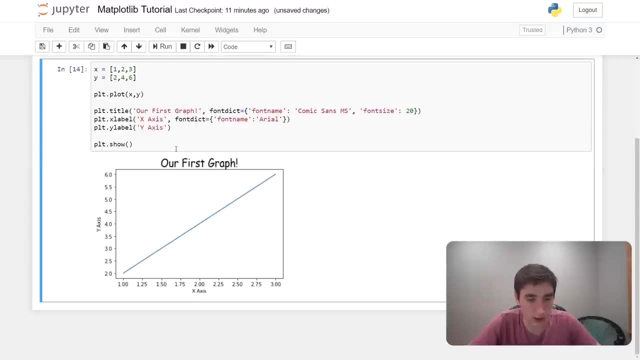 I could do like font dict equals. let's say, I wanted to make this font REL And that, honestly, might be the default. But if I did it like Comic Sans as well, you can tell that the X-axis now has changed. But I'm going to just leave that at this B for now. 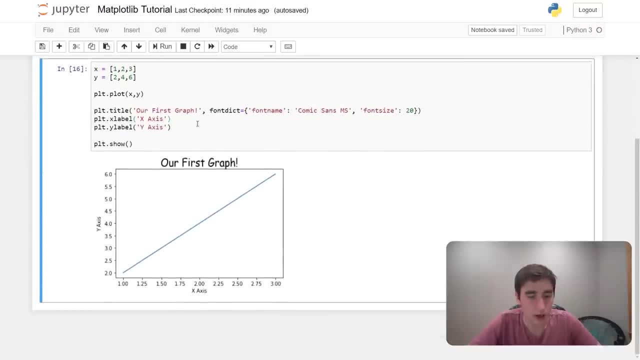 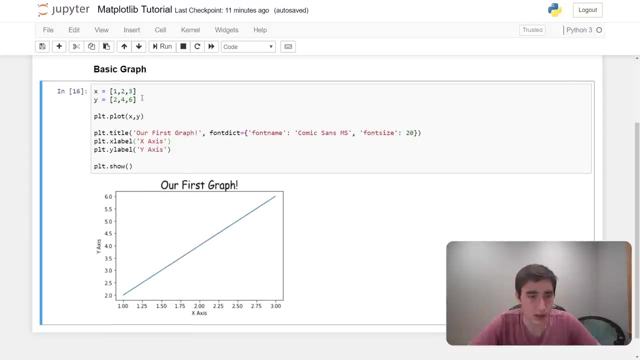 Okay, so we did labels, All right. so now one thing. One thing that's bothering me is the tick marks. Let's say, I just want to do integer numbers And I'm going to add a couple more values to our graph. 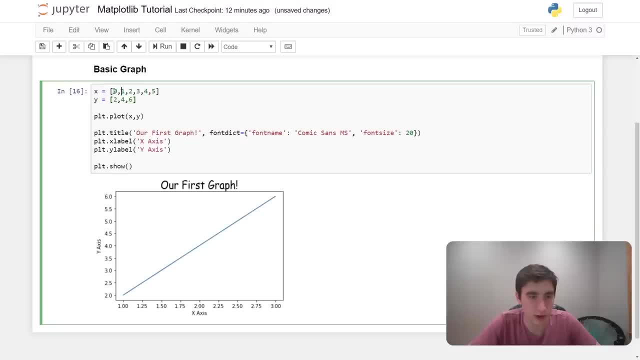 So I'm going to go to 5. And we'll start at 0.. And Y is always going to be 2 times X, So it's going to look like that. Oh wow, it magically did it for us in that case. 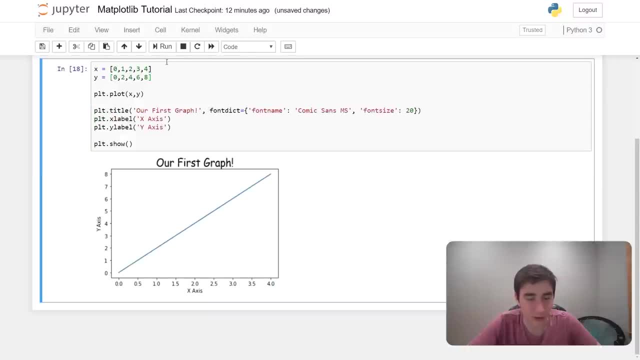 I don't want it to magically do it for us. Okay, Let's say, Let's say we went to 4, and we wanted just the integer values. We didn't want any of the decimal values. So how do we change our ticks? 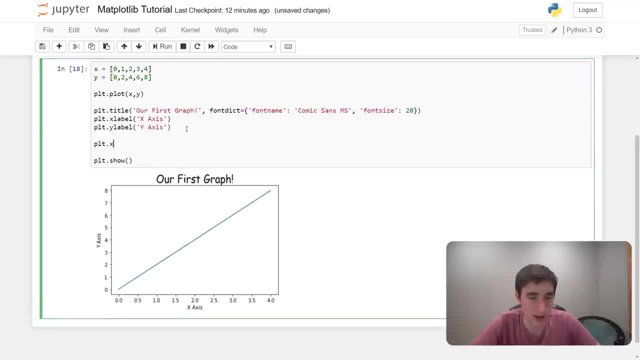 So we can do that by doing plotXTicks, And our X ticks will do 0,, 0,, 1,, 2,, 3.. And I also just found, remember this command by using the documentation, And our Y ticks will be how about 0 to 10 every 2.. 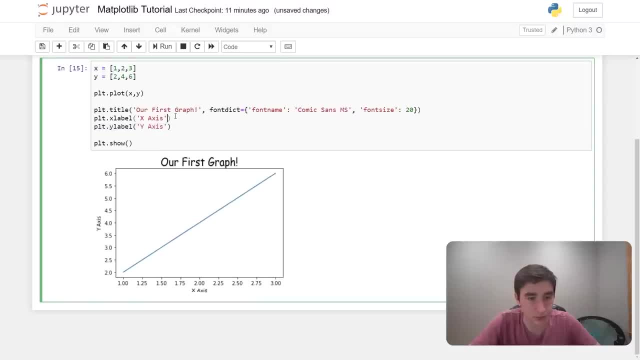 But I'm going to just leave that at this B for now. Okay, So we did labels, All right. So now one thing that's bothering me is the tick marks. Let's say, I just want to do integer numbers And I'm going to add a couple more values to our graph. 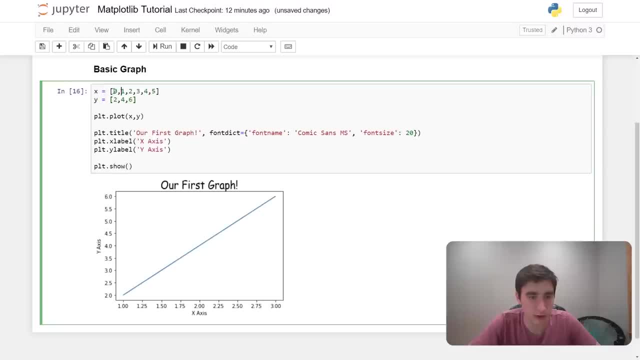 So I'm going to go to 5. And we'll start at 0.. And Y is always going to be 2 times X, so it's going to look like that. Oh wow, It magically did it for us in that case. 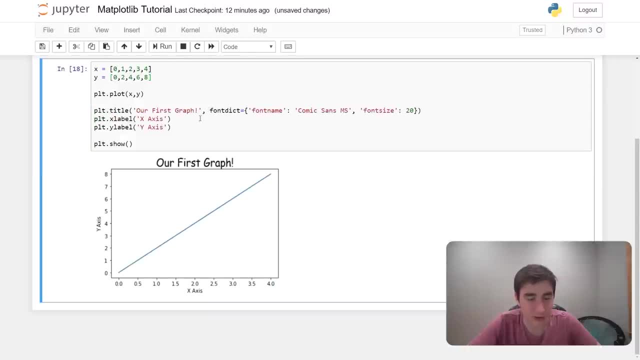 I don't want it to magically do it for us. Okay, Let's say we went to 4. And we wanted just the integer values. We didn't want any of the decimal values. So how do we change our ticks? So we can do that by doing plotxticks. 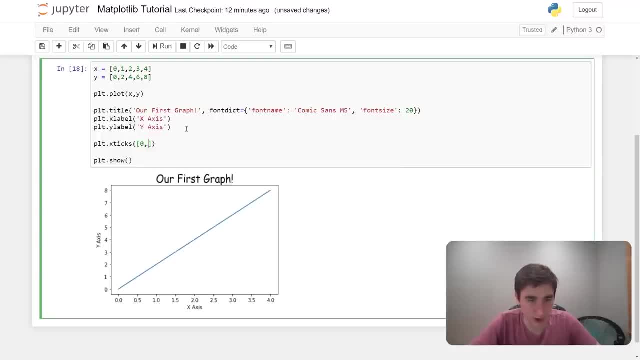 And our xticks will do 0.. 0,, 1,, 2,, 3.. And I also just found remember this command by using the documentation, And our yticks will be how about 0,, 2,, 10 every 2.. 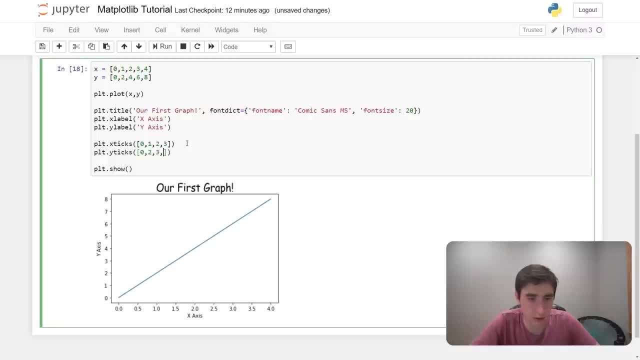 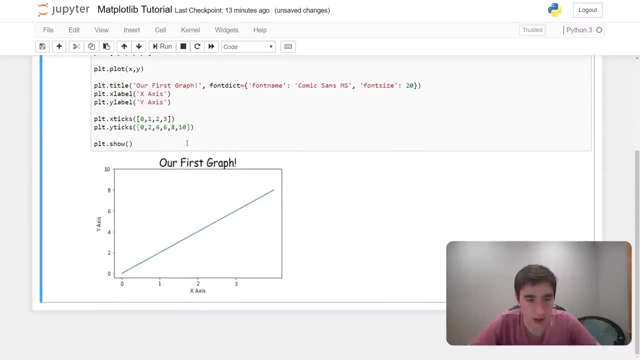 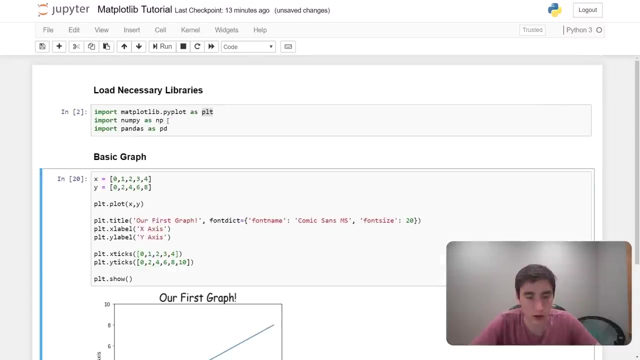 So 0,, 2,, 4, 6.. Oh my gosh, 10.. As you can see that now we have the tick marks working properly, And maybe I wanted to add Add 4 as well, So now we labeled our ticks differently. 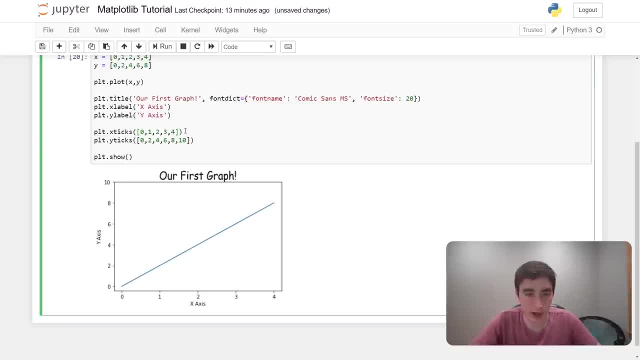 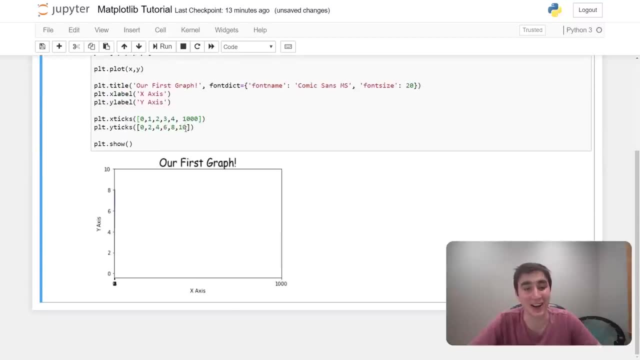 And one thing that's cool to know is that the graph will automatically resize based on how we set this. So if I set 1 tick to 1,000, well, now our graph kind of looks like not too good, But it's nice that you can easily do that. 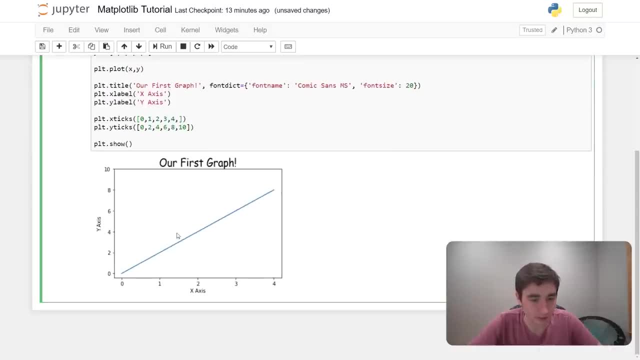 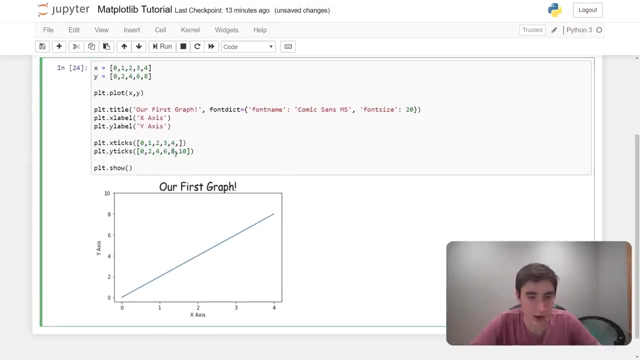 4 is better, But you can do the same thing with y. Let's say, when did I make the last one? 100.. As you can see, it changes up the sizing of the graph. One thing that's also cool, though, is, even if I did evenly space these out, if I did like 7 here and then 7.5,. 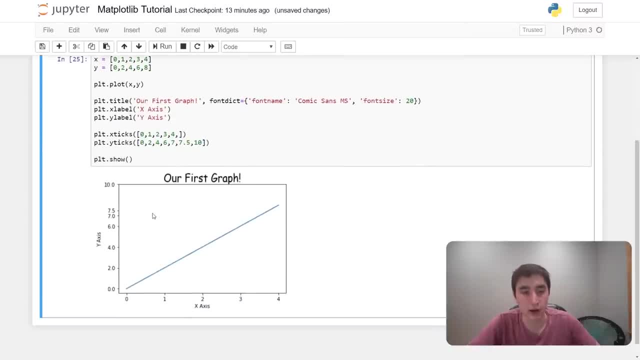 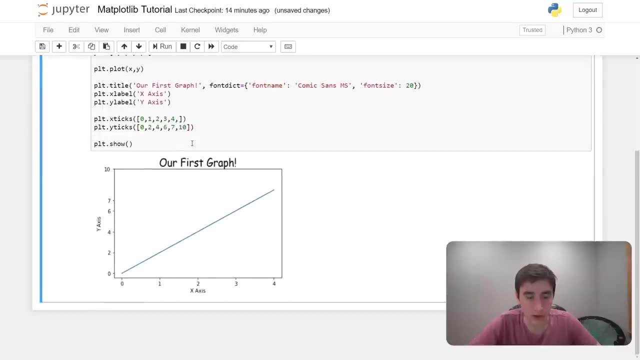 as you can see it properly puts those at the right spot in the graph. I'll leave it like this. I'll leave it a little bit weird, But yeah, that looks good to me. Okay, so we have our first graph. 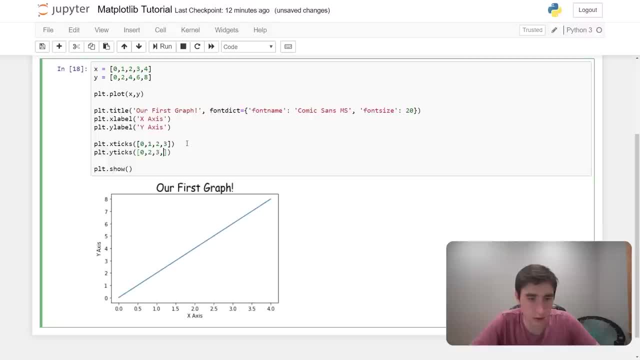 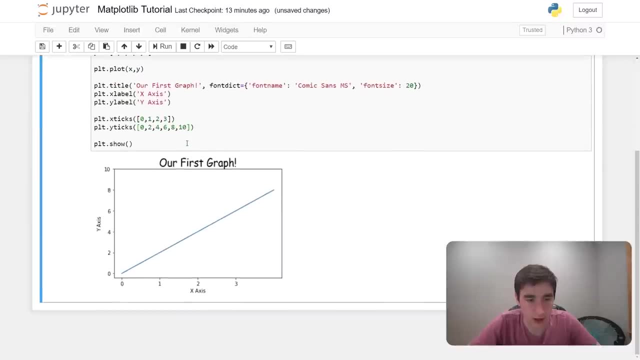 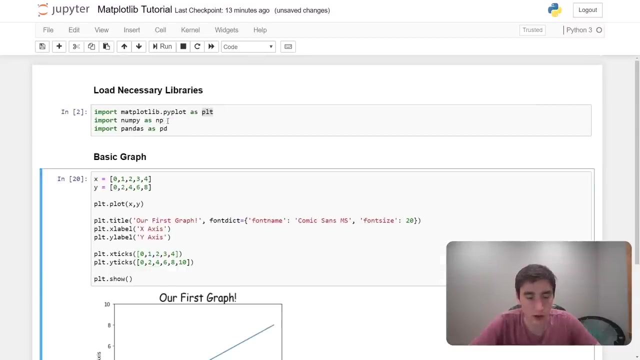 So it's 0,, 2,, 4,, 6.. Oh my gosh, 10.. As you can see that now we have the tick marks working properly, And maybe I wanted to add 4 as well, So now we labeled our ticks differently. 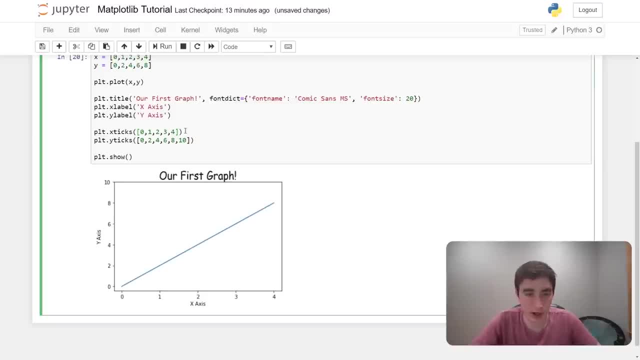 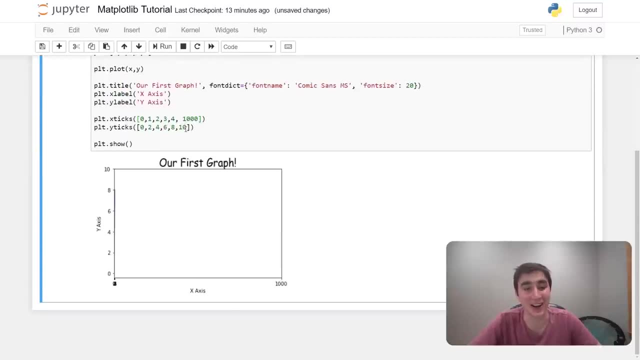 And one thing that's cool to know is that the graph will automatically resize based on how we set this. So if I set 1, tick to 1,000.. Well, now our graph kind of looks like not too good, But it's nice that you can easily do that. 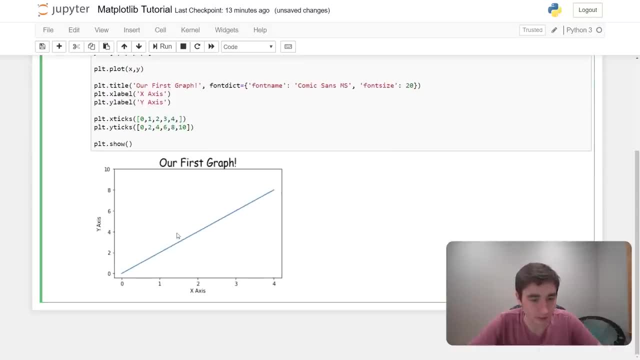 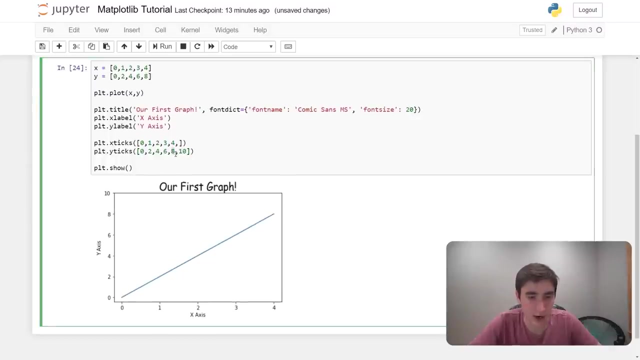 4 is better, But- And you can do the same thing with Y- Let's say I wanted to make the last one 100.. As you can see, it changes up the sizing of the graph. One thing that's also cool, though, is even if I didn't evenly space these out. 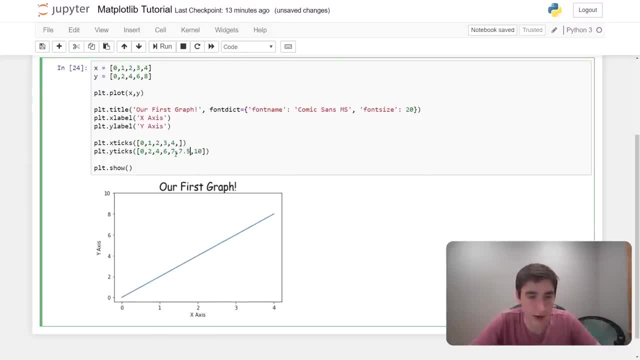 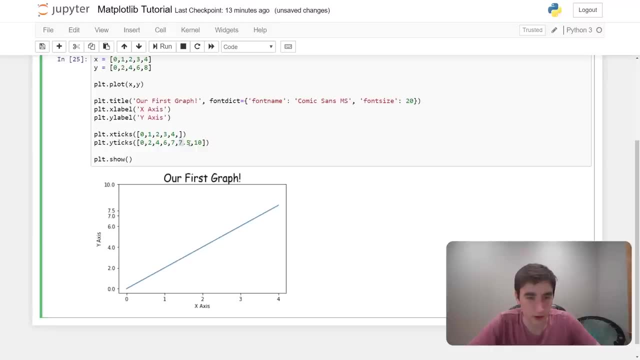 if I did like 7 here and then 7.5.. As you can see, it properly puts those at the right spot in the graph. I'll leave it like this. I'll leave it a little bit weird, But yeah, that looks good to me. 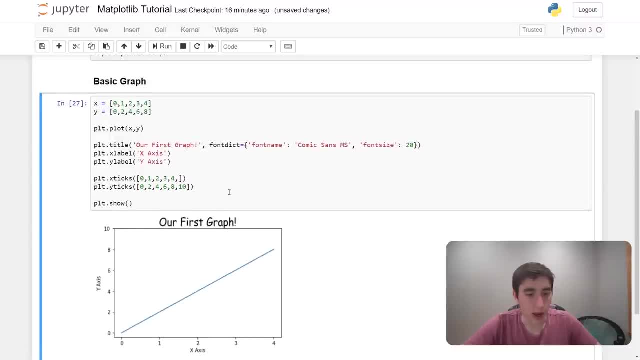 Okay, so we have our first graph. Let's add a legend and make this line a little bit more exciting color-wise. So if we wanted to add a legend, we can do, And I'm going to actually Because I like showing how the documentation is helpful. 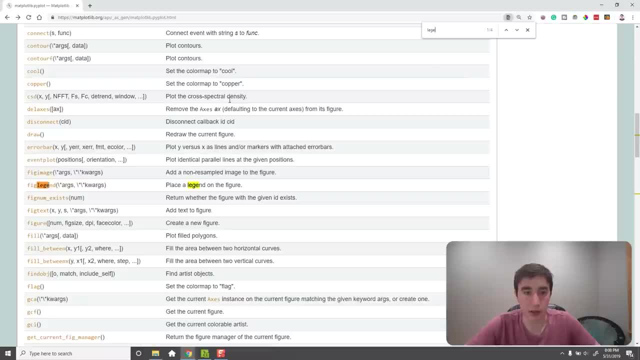 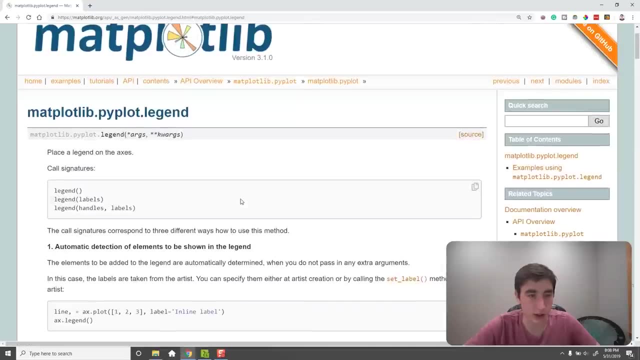 If I look at this, I'm going to do this. I'm going to do this. If I looked up legend- fig legend, that might work. Just this legend: Place a legend on the axes. By looking up legend, I've figured out that the call is just legend. 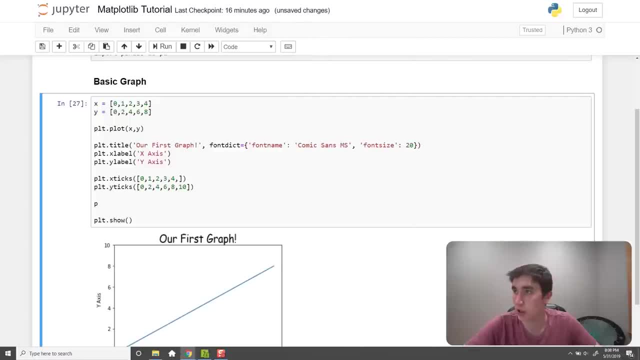 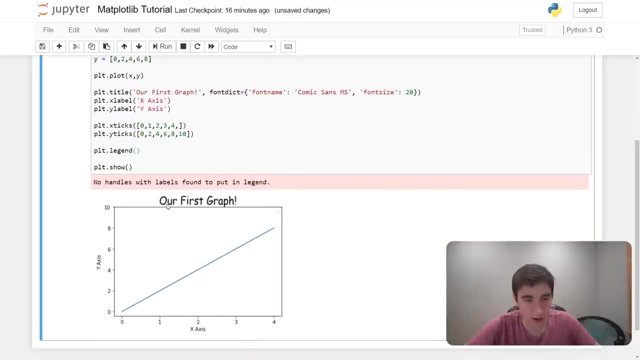 And it gives me some examples. So I always like to refer to this documentation. Okay, so pltlegend, And what happens when I do that? No handles with labels found to put in legend. So it's complaining because we don't have anything to label. 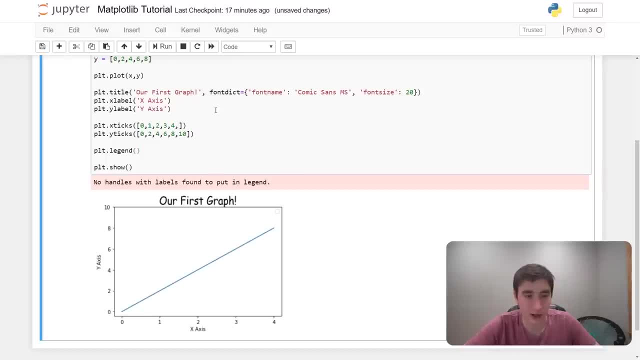 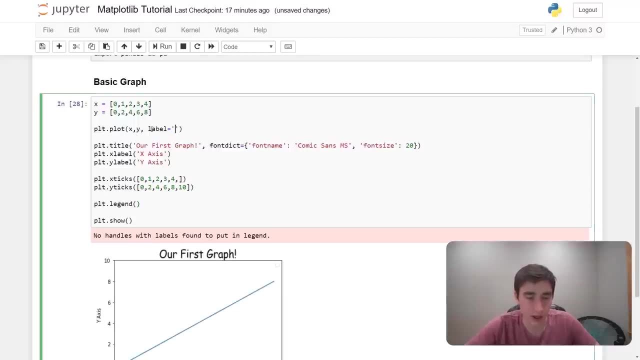 What it says? What it's saying is: how do we label this line? And the way we do that is by passing in a label to our plot function. So in this case, our x and y. we plotted x to be Or y to be 2 times x. 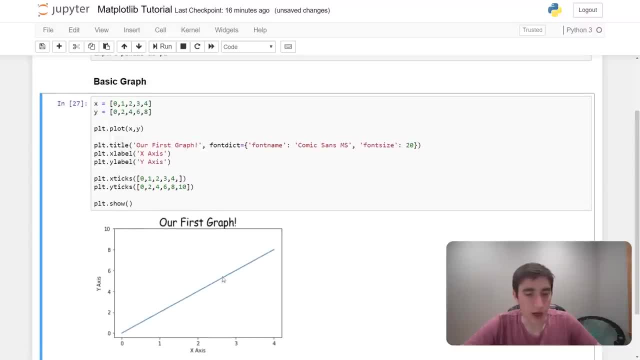 Let's add a legend and make this, Let's make this line a little bit more exciting color-wise. So if we wanted to add a legend, we can do, and I'm going to actually because I like showing how the documentation is helpful. 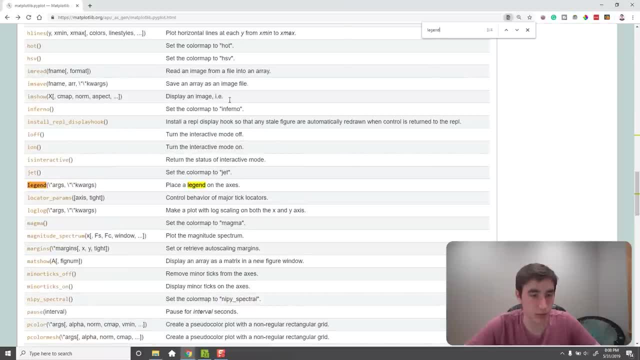 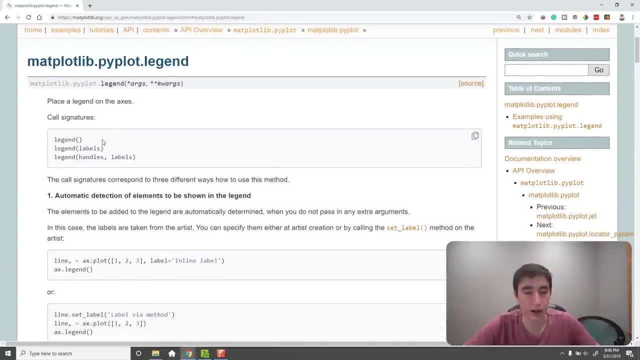 If I looked up legend- fig legend- that might work. Just this legend- Place a legend on the axes, Like by looking up legend, I figured out that the call is just legend And it gives me some examples. So I always like to refer to this documentation. 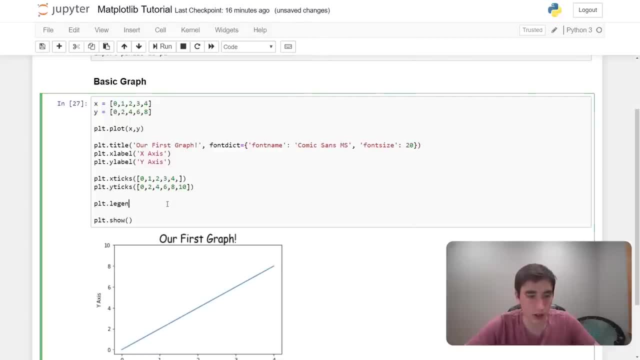 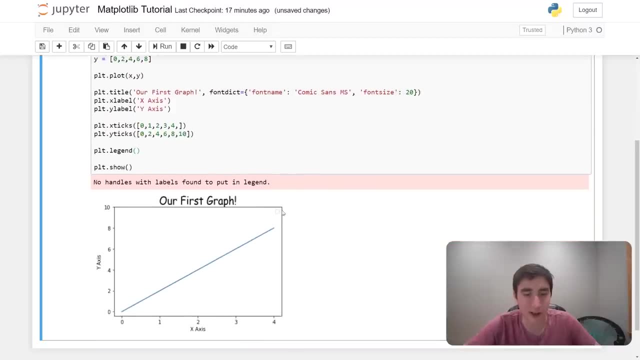 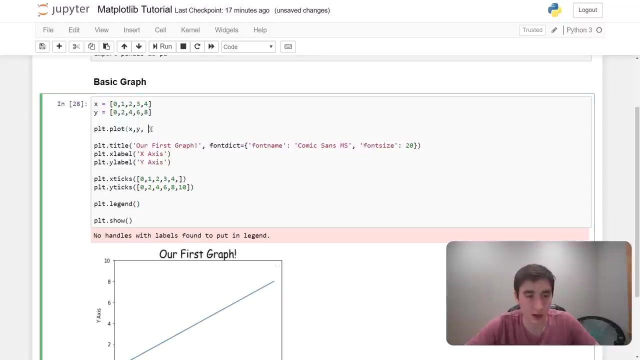 Okay, so pltlegend. And what happens when I do that? No handles with labels found to put in legend. So it's complaining because we don't have anything to label. What it's saying is: how do we label this line? And the way we do that is by passing in a label to our plot function. 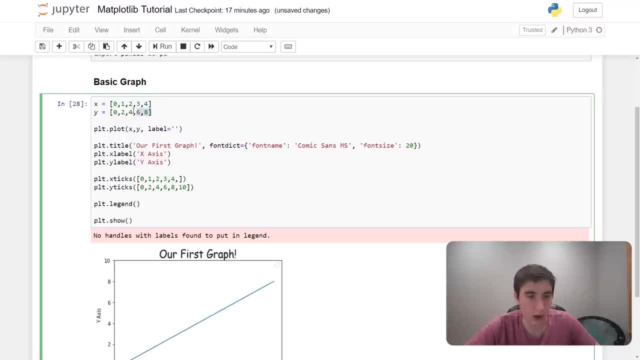 So in this case, our x and y. we plotted y to be 2 times x, So I'm going to call the label here Here 2x, And, as you can see, we get 2x right there. Okay, let's say now that we wanted to change up the color of this line, maybe make it thicker, do some other things to it. 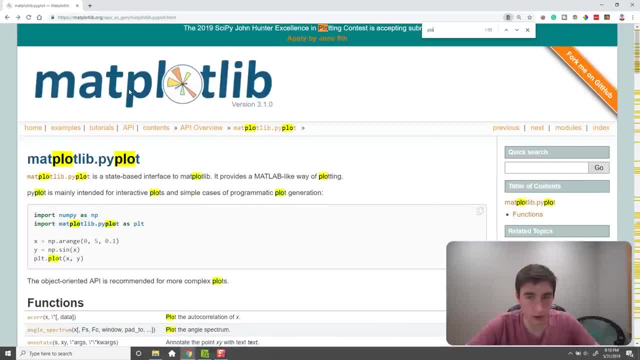 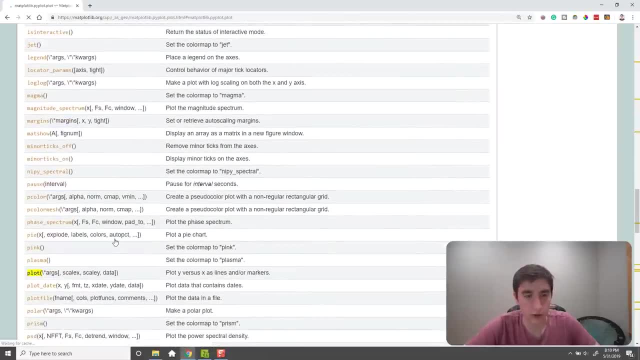 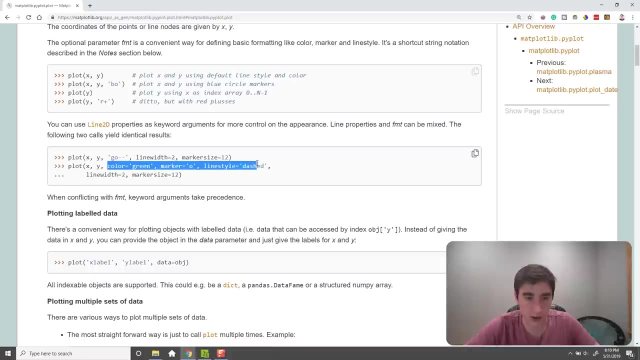 If we go to plot Where's plot, We'll see all sorts of properties that we can do in plot. So what I'm seeing right here is you can pass in all of these different parameters to our plot And it probably lists off what we can put, maybe not. 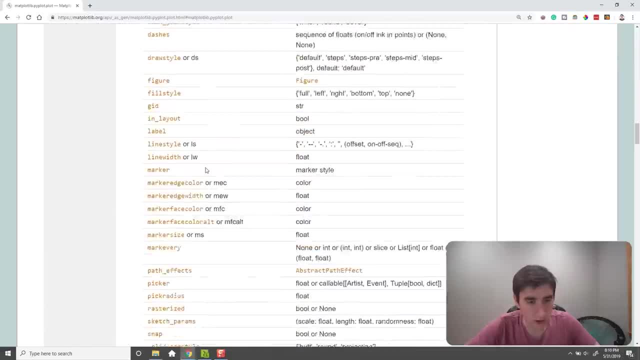 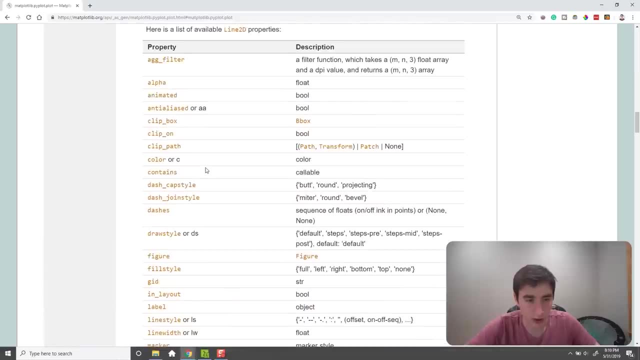 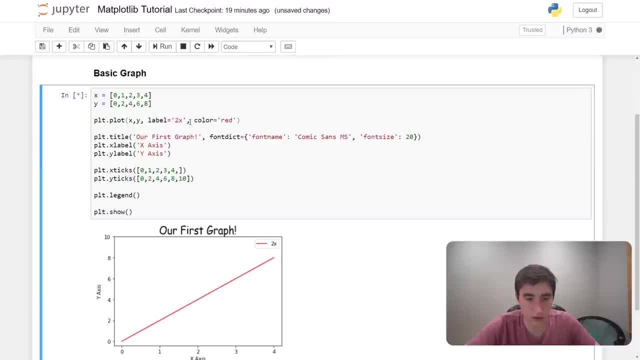 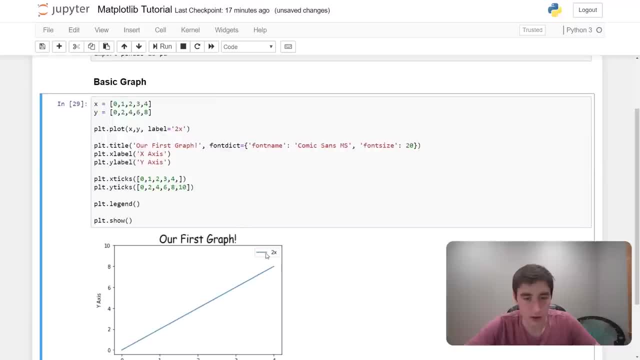 So I'm going to call the label here 2x And, as you can see, we get 2x right there. Okay, let's say now that we wanted to change up the color of this line, Maybe make it thicker, Do some other things to it. 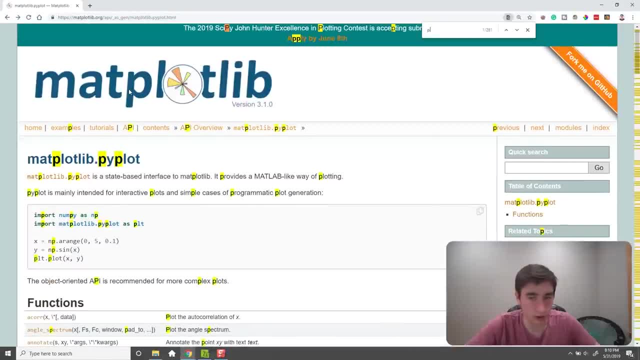 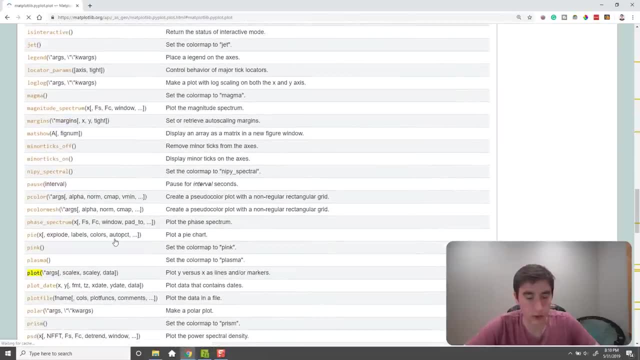 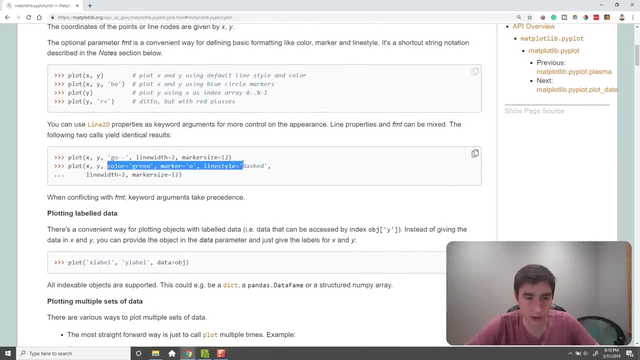 If we go to plot- Where is plot? We'll see all sorts of properties that we can do in plot. So what I'm seeing right here is you can pass in all of these different parameters to our plot And it probably lists off what we can put. 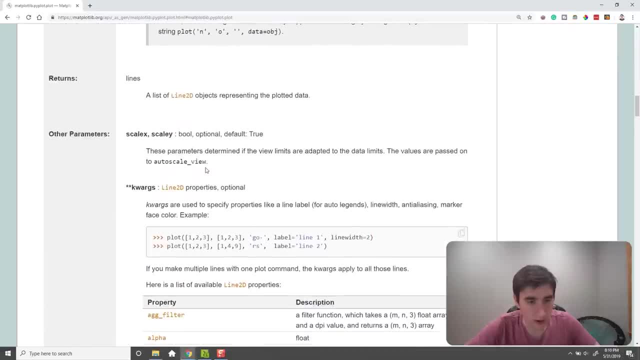 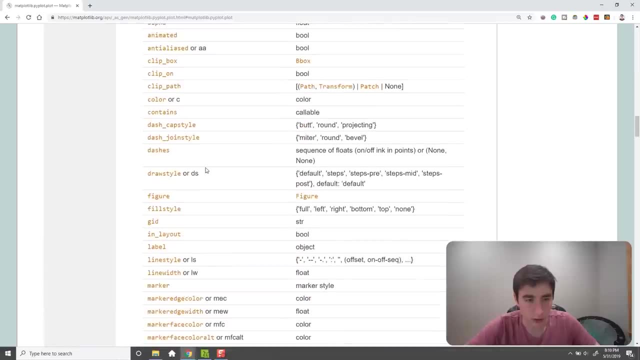 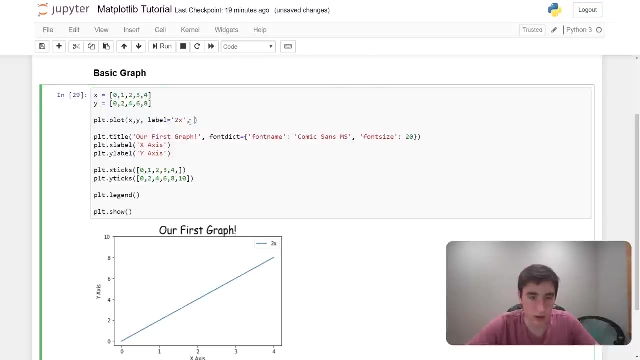 Maybe not. It's not super specific, But if you look hard enough, yeah, you can see all of these properties that you can pass into the plot function. So one thing we could pass in is color. So if I passed in color equals red, it will work. 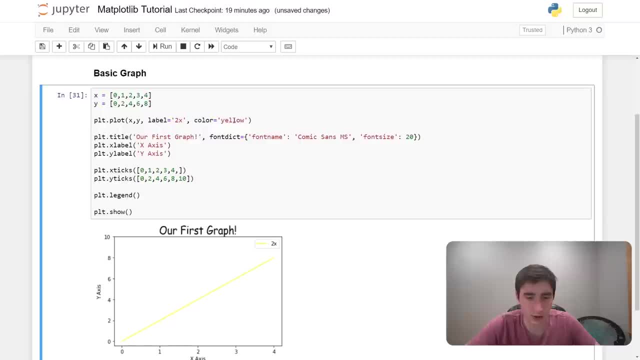 And it will know, I think, the common colors. So if I did yellow, If I did like yellow, which is not a color it's going to yell at me, It might even work with Y Yeah cool. 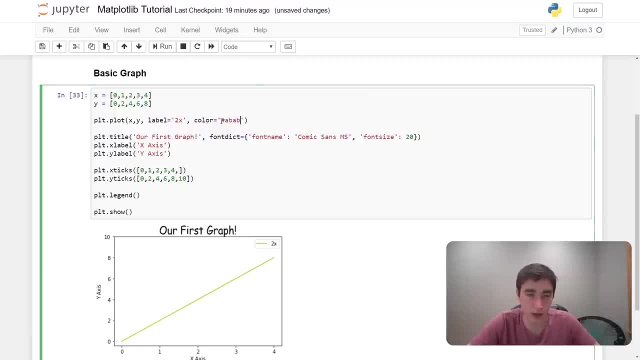 And we also can pass in hexadecimal colors, So I could do like ABABAB And we get like a grayish color. This is helpful because you can use like a color picker tool and pick pretty much any color we want here. 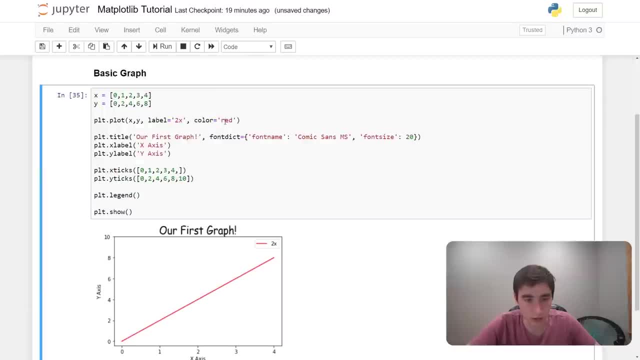 But we'll stay with red for now. The other parameters I could pass into that. Let's see what else we had I could do. I think line size equals, let's say, 12.. Oh, that is not a parameter. 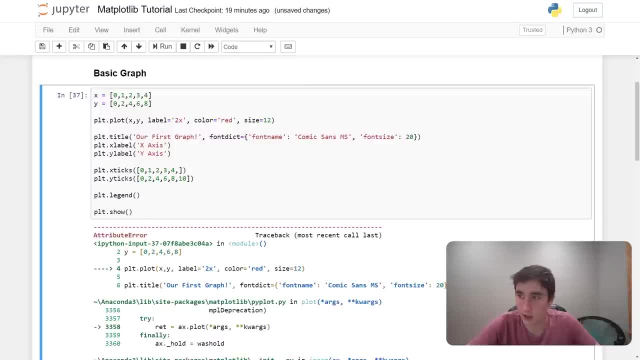 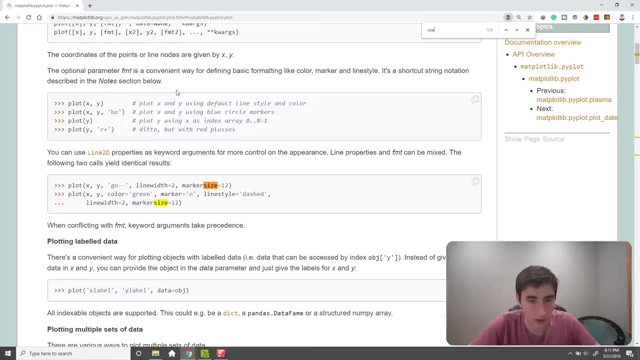 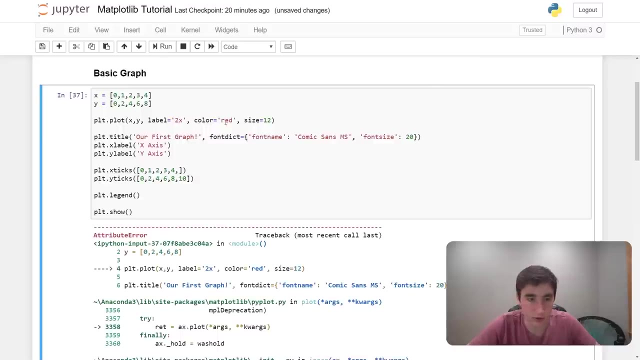 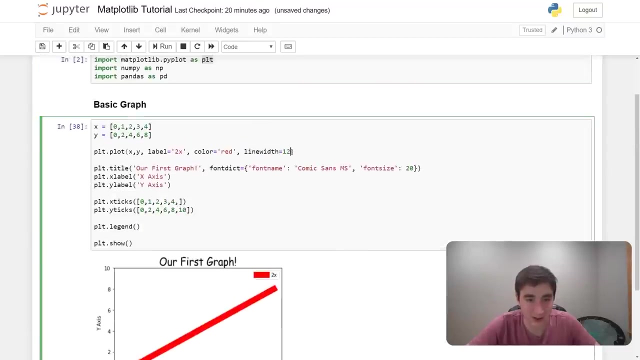 Ah, not a parameter either. Go back to my documentation: Size, Marker size. Maybe that's it, Marker size. Oh, I also see line width here. So line width equals 2.. Oh my gosh, Line width equals 12. makes this big line. 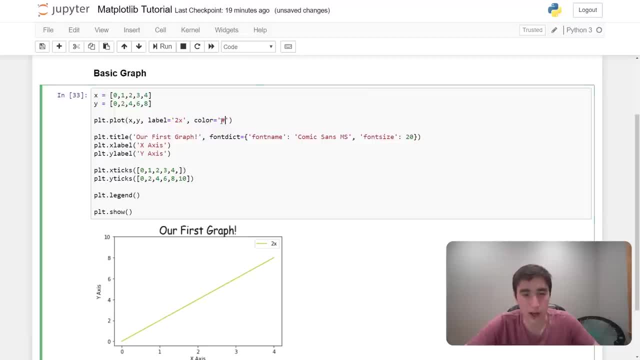 It might even work with y, Yeah cool, And we also can pass in hexadecimal colors. So I can do like a b a, b a b, And we got like a grayish color. This is helpful because you can use like a color picker tool and pick pretty much any color we want here. 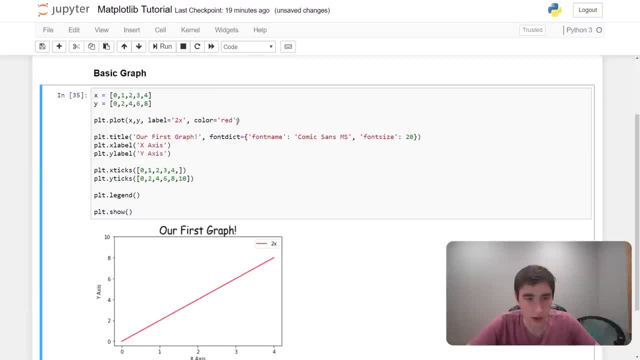 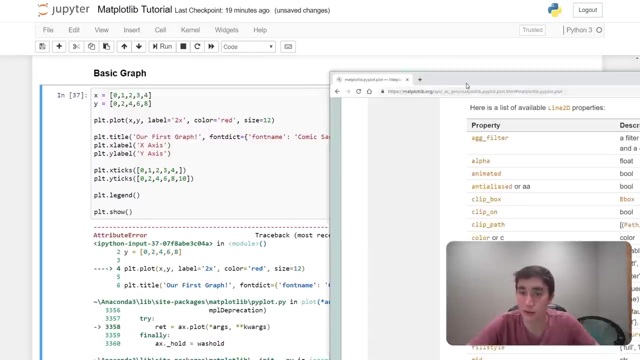 but we'll stay with red for now. the other parameters I could pass into that. let's see what else we had. I could do. I think line size equal, let's say 12. oh, that is not a parameter. not a parameter either. go back to my documentation size. 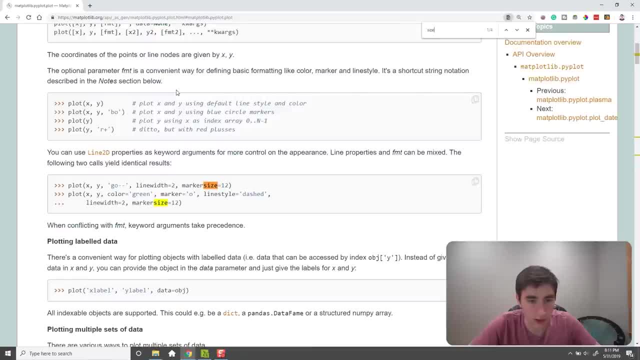 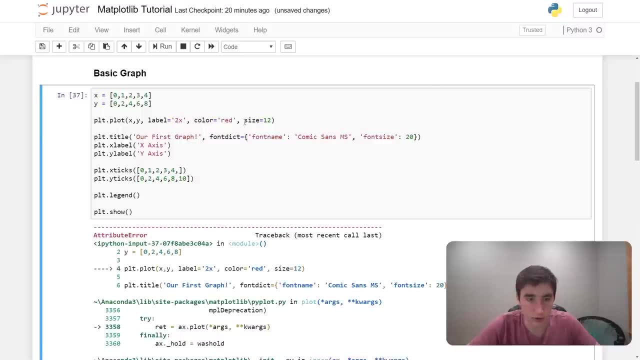 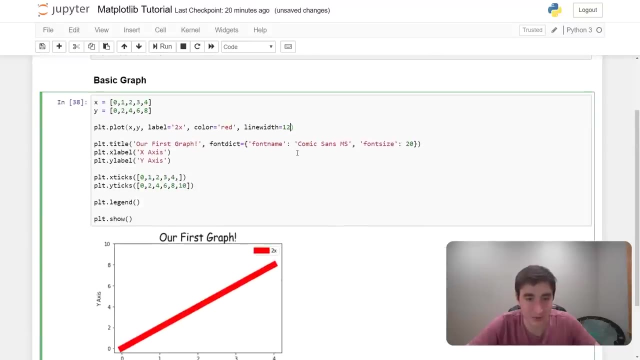 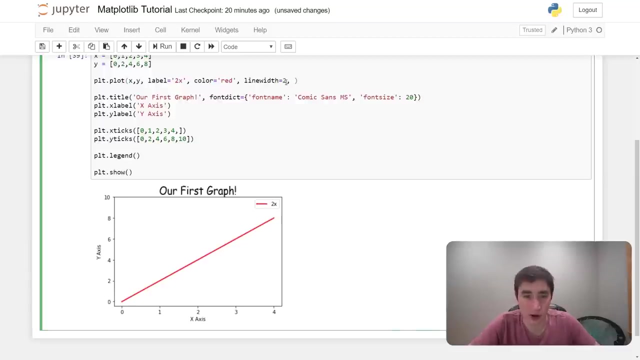 marker size. maybe that's it. marker size. oh, I also see line width here. so line width equals two. oh my gosh, line width equals 12. makes this big line maybe two. it's a bit bigger than I think what we had. we can also do, we can label. 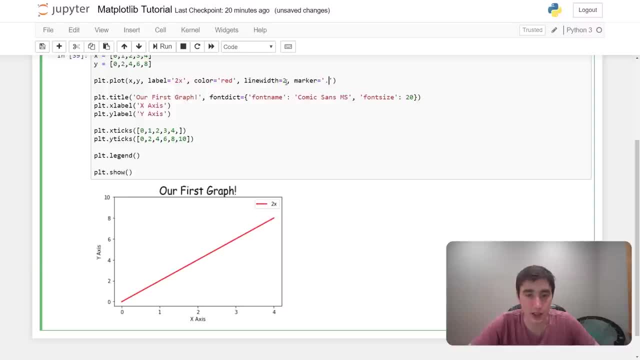 a marker. so let's say, I wanted to add dots into this. as you can see, you can't really see it too too well, but maybe if I made the marker size a little bit bigger and I'm just kind of passing this in so you can kind of see what you can do, oh, that didn't work. let's say 10. yeah, as you can. 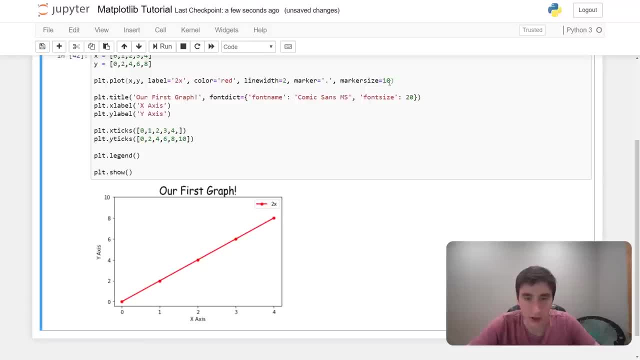 see now you see big dots on our graph. I can also do marker edge color. there's all sorts of properties. I'm just like continually passing these in. but now you see a different Marker Edge color and I think I did that wrong, but I was able to. 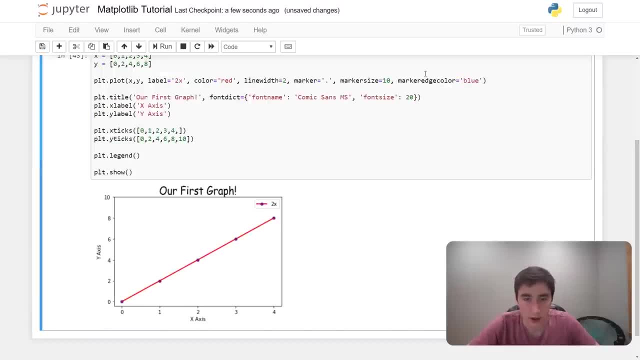 different type of dot and whatnot. So this is pretty cool that we can have all of this customization. It sometimes takes a little while to get what we want, but it's usually. it's just nice to have this power. And one final thing I'll pass in is line style. 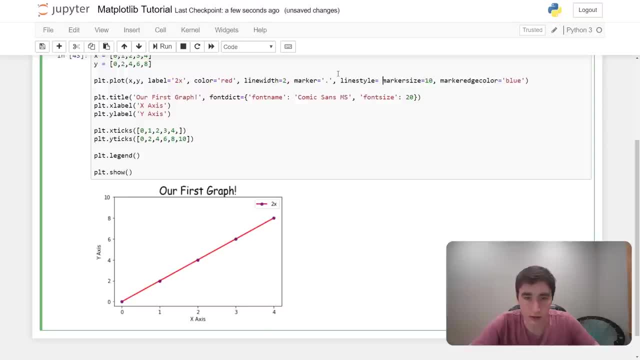 So there's all sorts of line styles we can pass in and you can read all into the different ways you can do this in the documentation. One thing that's pretty cool is that instead of listing all of these keyword arguments, sometimes we just want to make: 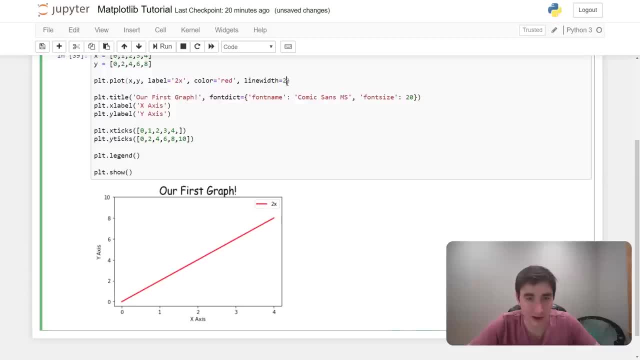 Maybe 2.. It's a bit bigger than I think what we had. We can also do. We can label a marker. So let's say I wanted to add dots into this. As you can see, you can't really see it too, too well. 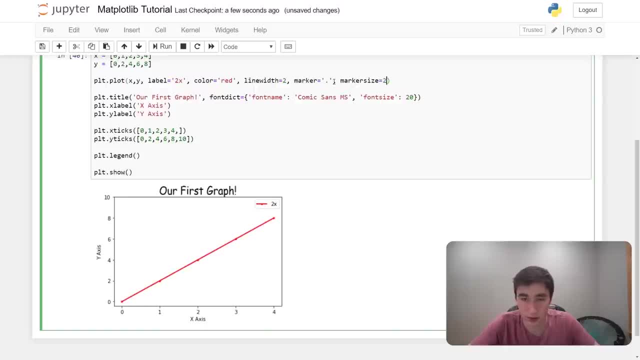 But maybe if I made the marker size a little bit bigger, And I'm just kind of passing these in so you can kind of see what you can do. Oh, that didn't work, Let's say 10.. Yeah, as you can see now you see big dots on our graph. 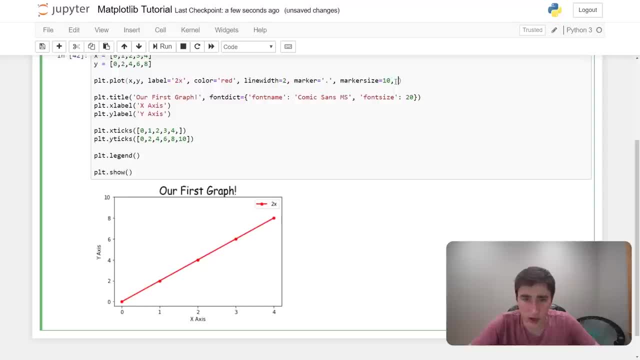 I can also do marker, edge color. There's all sorts of properties. I'm just like continually passing these in, But now you see a different type of dot and whatnot. So this is pretty cool that we can have all of this customization. 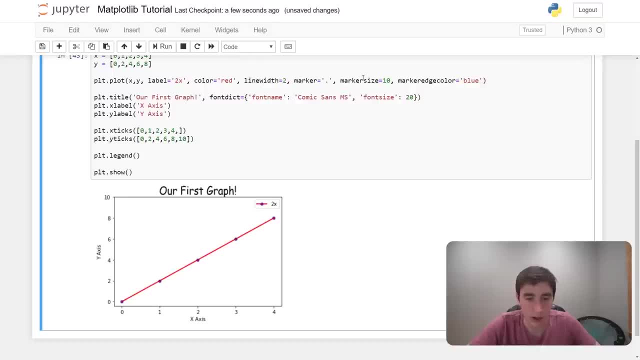 It sometimes takes a little while to get what we want, But it's usually. It's just nice to have this power. And one final thing I'll pass in is line style. So there's all sorts of line styles we can pass in. 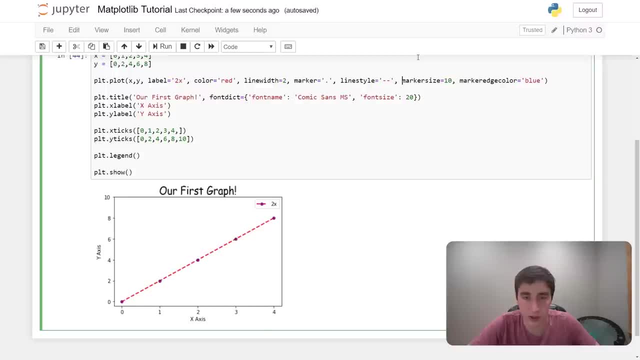 And you can read all into the different ways you can do this in the documentation. One thing that's pretty cool is that instead of listing all of these keyword arguments, sometimes we just want to make a different type of line quickly. So there's actually a shorthand that you can use to kind of do pretty much the same thing. 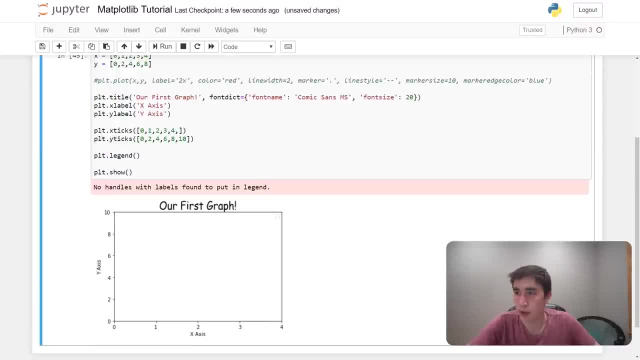 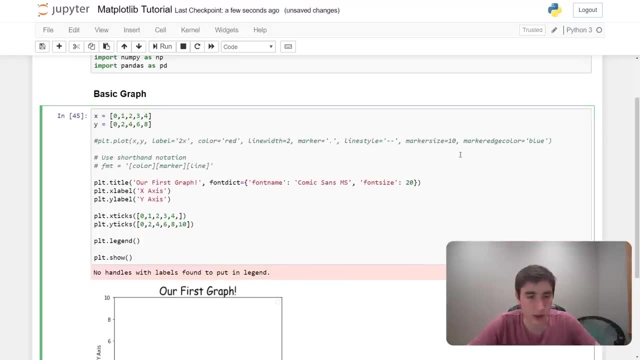 So, if I comment this out real quick, we have no graph. What you can do is there's a shorthand notation that allows you to kind of have a pretty good amount of customization quickly. So the shorthand notation is color marker, line, Marker line, style, I guess. 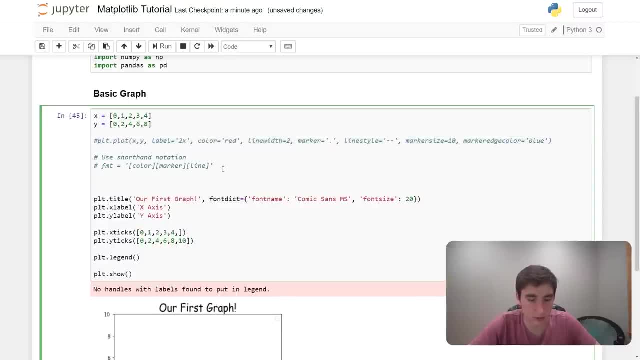 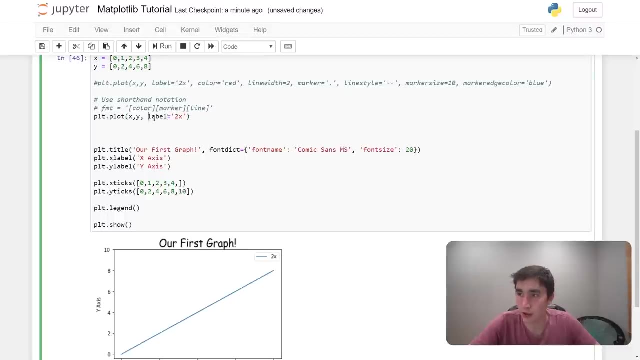 So if we go and copy this line from above, let's say we just passed in this. Now what we can do is, before we add our label, we can pass in the shorthand notation. So I can do color. We'll say red. 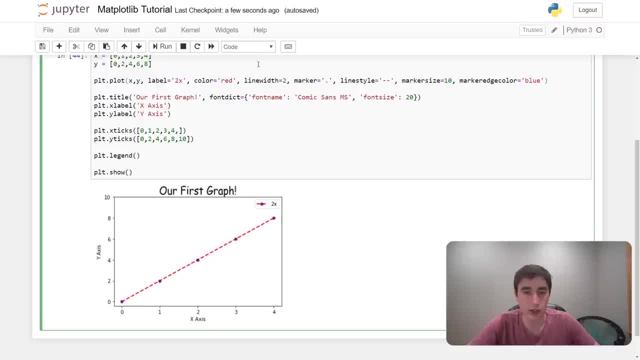 a different type of line quickly. So there's actually a shorthand that you can use to kind of do pretty much the same thing. So if I comment this out real quick, we have no graph. What you can do is there's a shorthand notation. 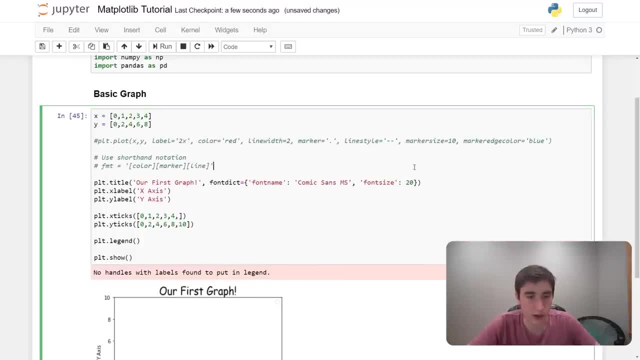 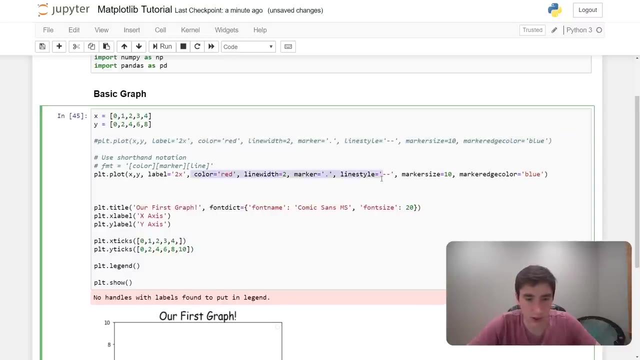 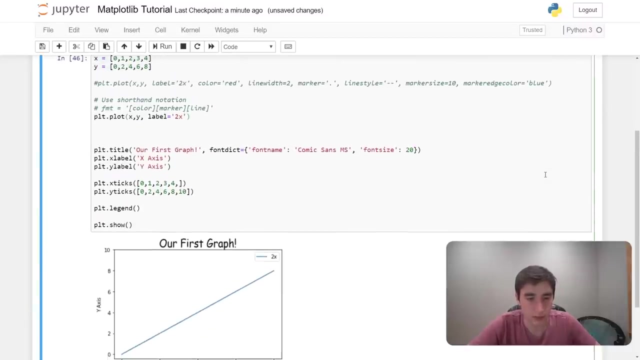 that allows you to kind of have pretty good amount of customization quickly. So the shorthand notation is color marker line style, I guess. So if we go and copy this line from above, let's say we just passed in this. Now what we can do is, before we add our label, 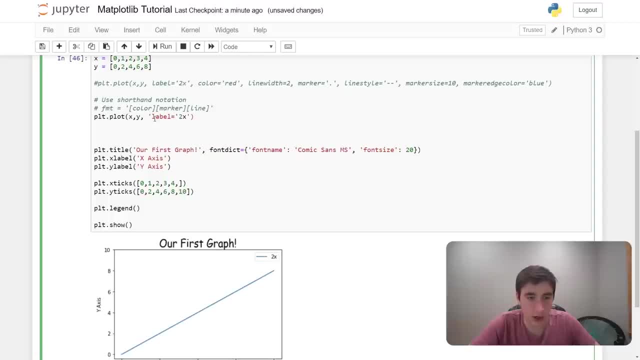 we can pass in the shorthand notation So I can do color. we'll say red and I think it just accepts letters. You can look into the documentation, see exactly what it does. Marker, we'll do a dot and then line, we'll do a dash. 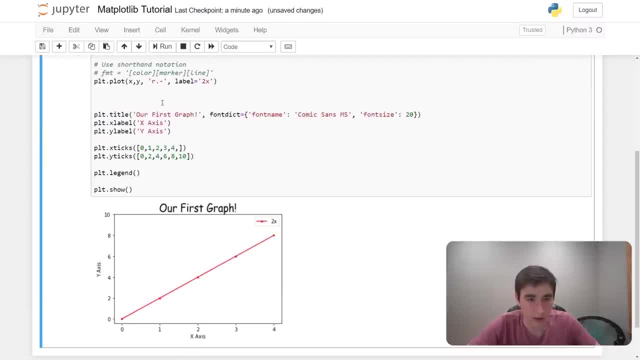 So watch what happens when I do this. It gives us a nice line with dots in it. If I do two dashes gives us a dotted line. If I do like a different type of marker, I can pass in like a carrot, like that. 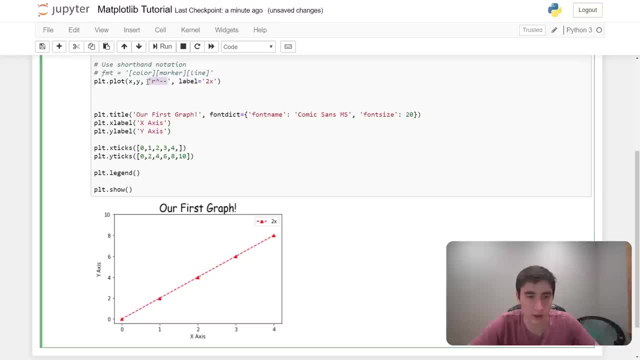 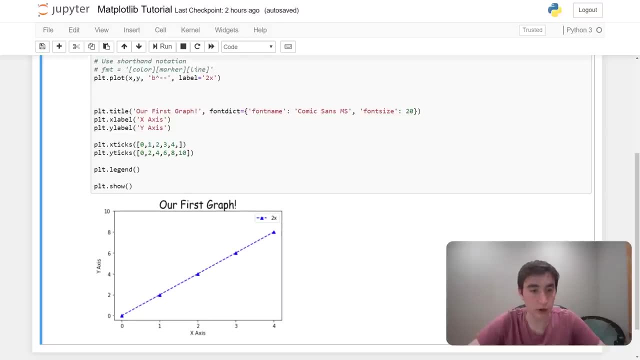 Gives us a line with carrots in it. It's kind of cool that you can do this shorthand notation and get different types of lines very easily. Just to follow up on the whole shorthand notation, I'm pulling in the docs for the plot function. 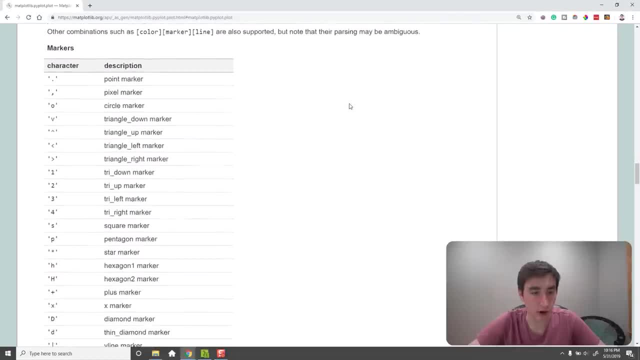 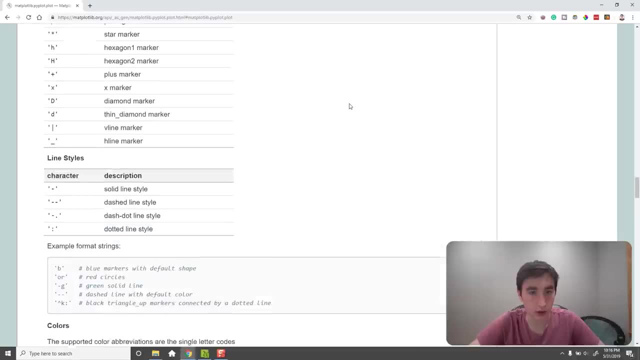 I'm pulling in the docs for the plot function. I'm pulling in the docs for the plot function. It shows all the different markers you can use and the different line styles supported and the different colors supported. So check out the plot documentation to see all that. 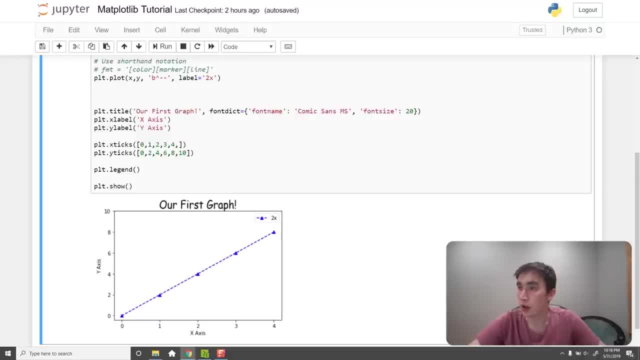 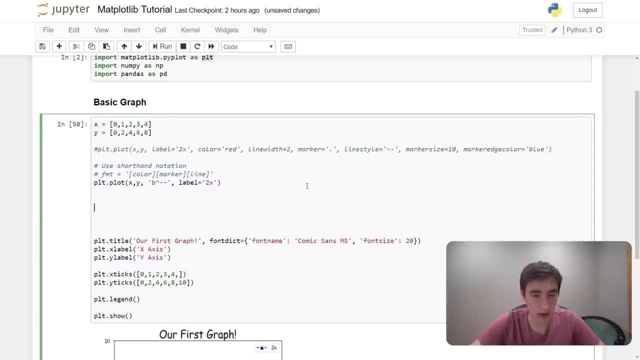 All right, let's move on to our next thing, and that will be, I guess let's just add another line real quick to our graph. So we have our first line, Let's add line number two, And this one will make a little bit more interesting. 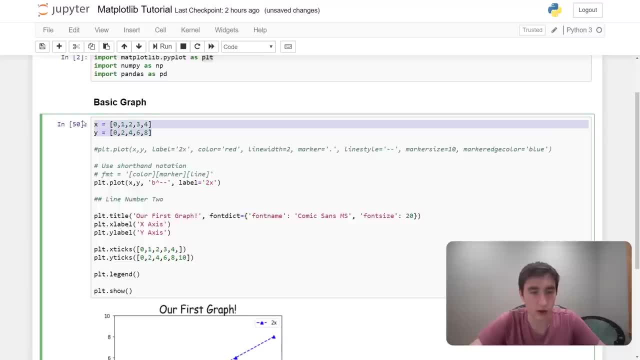 And the thing is like here we had a very straightforward like you have X and you have your Y. but this is not always easy to do, especially if you have like a function like sign, where you want to plot it at like a bunch of values. 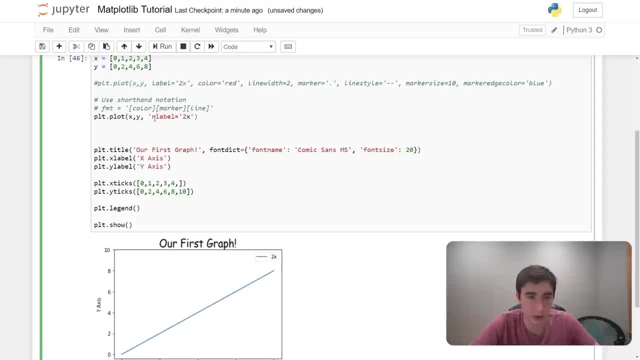 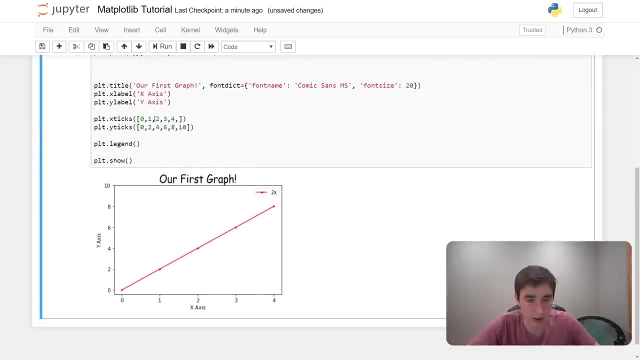 And I think it just accepts letters. So if I click into the documentation and see exactly what it does, marker will do a dot and then line will do a dash. So watch what happens when I do this. It gives us a nice line with dots in it. 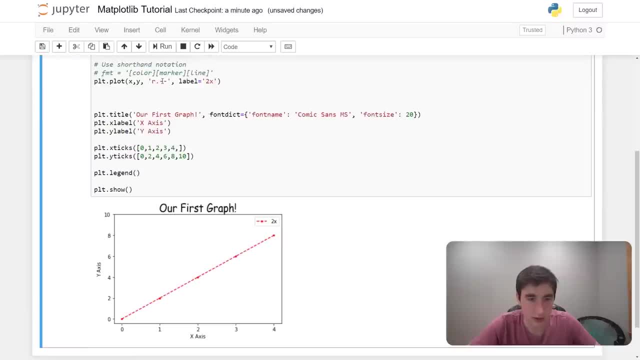 If I do two dashes it gives us a dotted line. If I do like a different type of marker, I can pass in like a caret, like that. It gives us a line with carets in it. It's kind of cool that you can do this. shorthand notation. 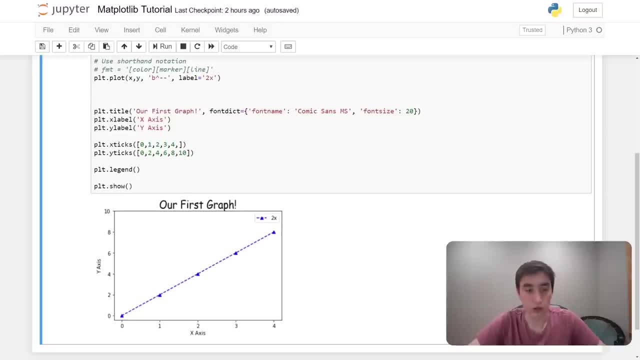 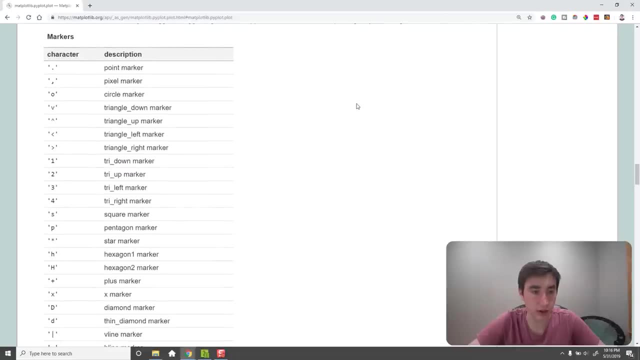 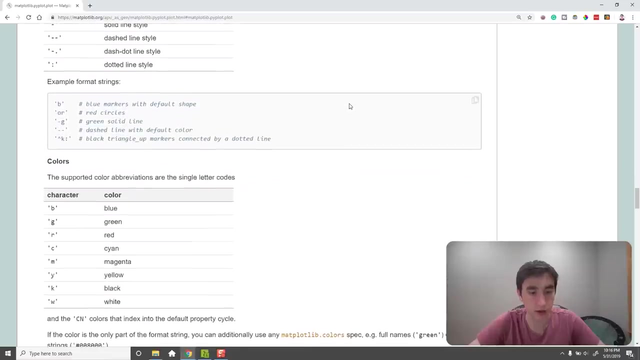 and get different types of lines Very easily. Just to follow up on the whole shorthand notation, I'm pulling in the docs for the plot function. It shows all the different markers you can use and the different line styles supported and the different colors supported. 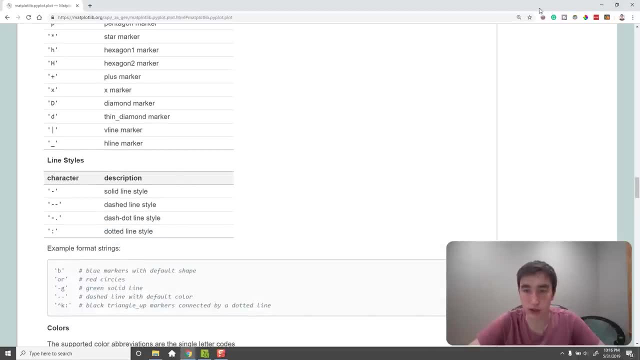 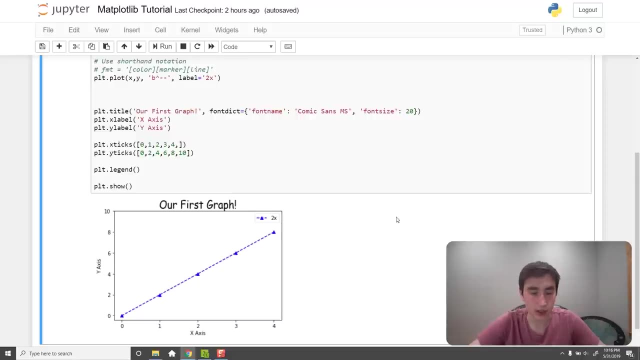 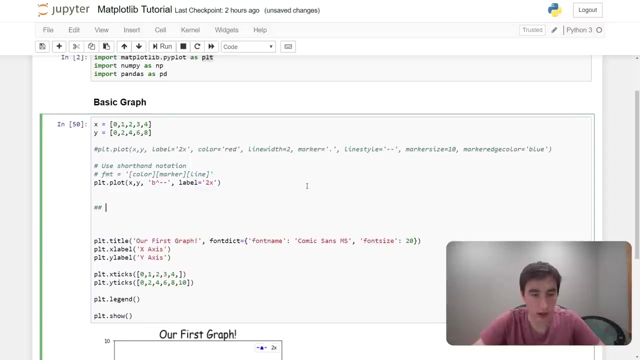 So check out the plot documentation to see all that. All right, let's move on to our next thing, And that will be, I guess. let's just add another line real quick. so we have our first line. Let's add line number two. 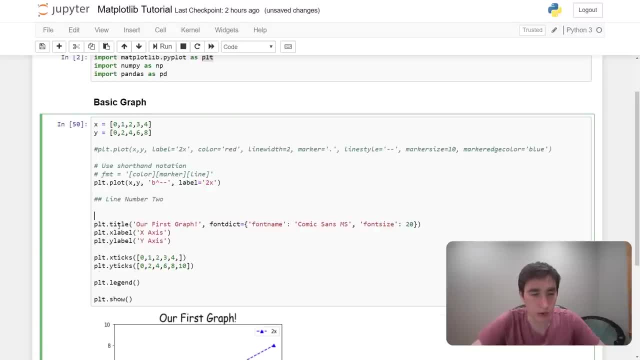 And this one will make a little bit more interesting. And the thing is like here we had a very straightforward like you have X and you have your Y. But this is not always easy to do, especially if you have like a function like sign. 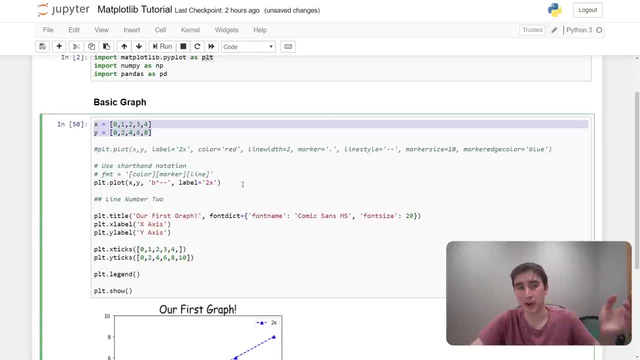 where you want to plot it at like a bunch of values, but those values are all, like you know, crazy decimals. So I want to show you how you can handle something like that. So this is where we use numpy. So I'm going to call this X2.. 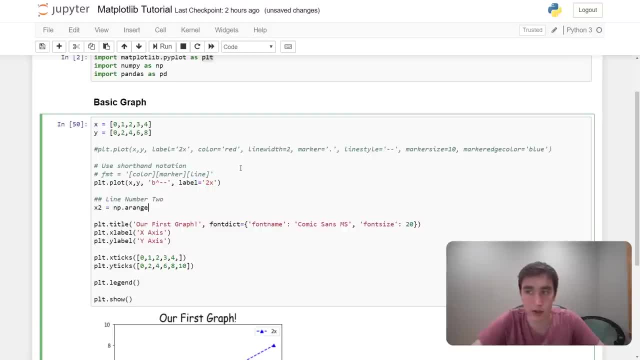 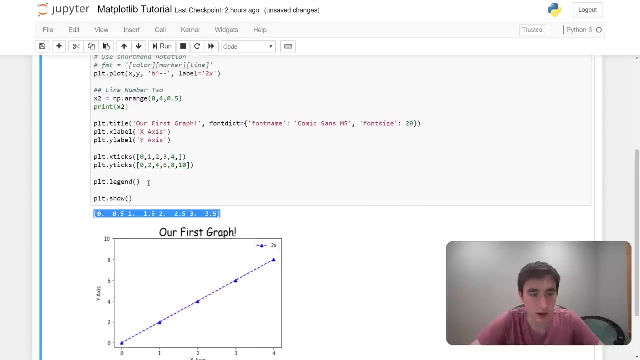 I'm going to say that X2 equals nparange 0 to 4 and we'll go by 0.5 as our tick. So if I print out X2 real quick, you see that this gives us a numpy array with 0, 0.5,. 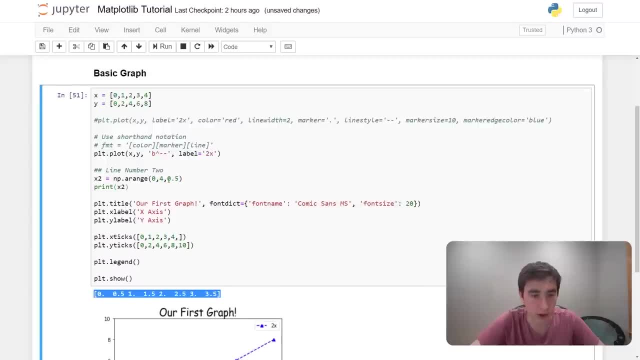 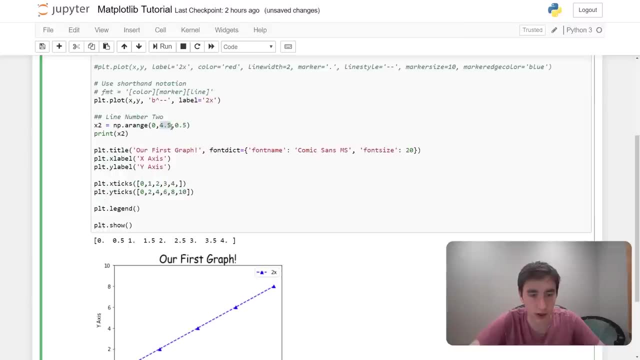 1, 1.5,, 2, 2.5,, 3,, 3.5.. I'll actually make it go to 4.5, so it goes to the same spot as our other graph, because this is exclusive here. 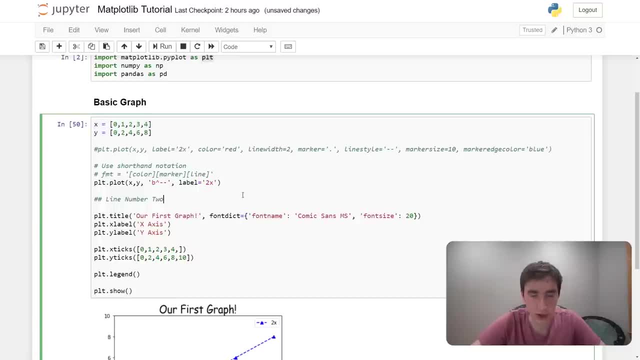 but those values are all, like you know, crazy decimals, So I'm gonna show you how you can handle something like that. So this is where we use NumPy, So I'm gonna call this X2.. I'm gonna say that X2 equals N. 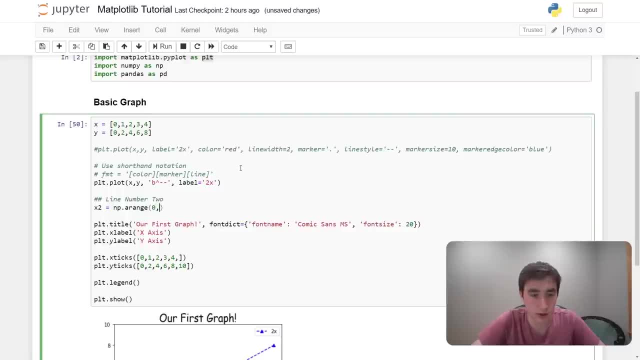 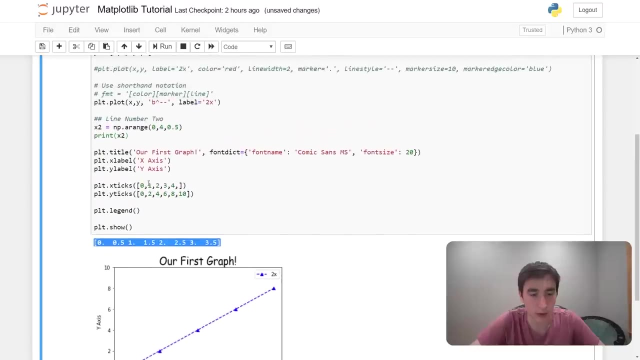 Nparange 0 to 4, and we'll go by 0.5 as our tick. So if I print out X2 real quick, you see that this gives us a NumPy array with 0,, 0.5,, 1, 1.5,, 2,, 2.5,, 3,, 3.5.. 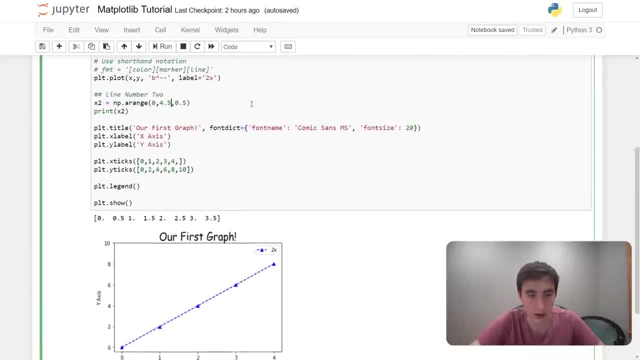 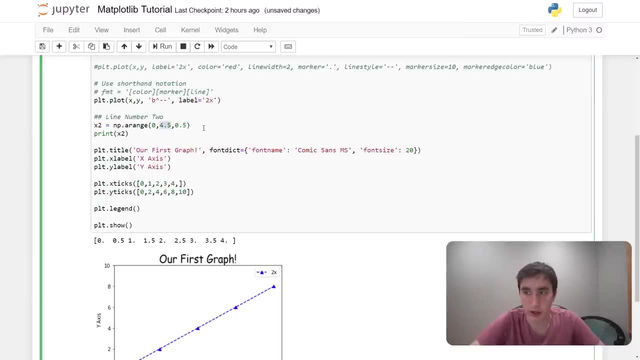 I'll actually make it go to 4.5.. So it goes to the same spot as our other graph, cause this is exclusive here, So we have that, So that's gonna be our Xs, And so what I can do here is I can go ahead and plot that. 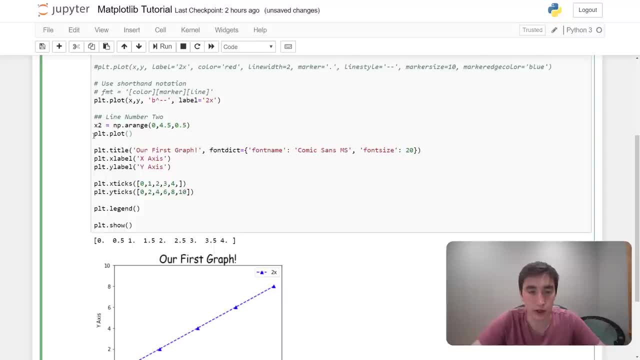 And I'm gonna plot the square function for it. So I'm gonna pass an X2, and then, instead of passing in a Y, I'm just gonna do X2, and I'm gonna do squared What happens here? So now you see, we get X2 squared. 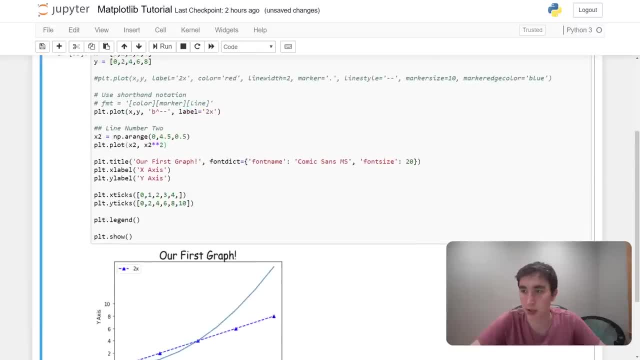 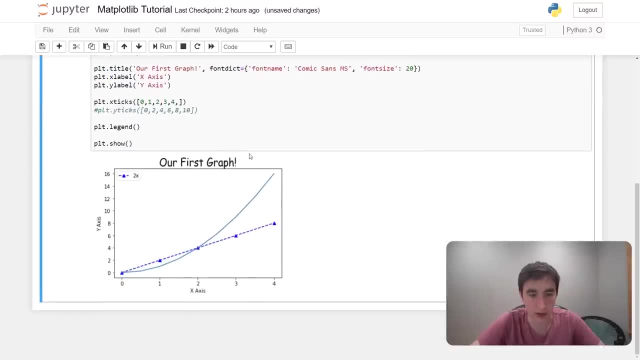 It goes a little bit higher than our original axis was set. So I'm gonna change up the ticks or maybe I'll just kind of comment this out and see what happens for our tick marks. Yeah, I'm fine with just leaving the default that it gave us. 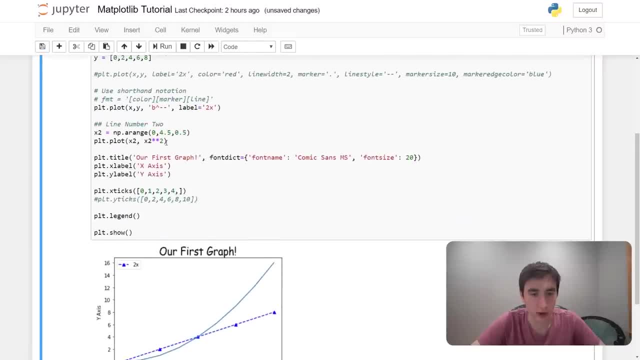 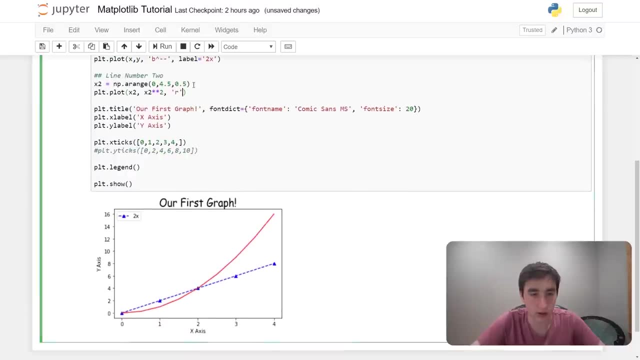 Looks good to me, And now we have two blue colors, So let's make this a different color. Maybe you make it red. We wanna give it a label as well, So I'm gonna do red. I'm gonna say the label is equal to X squared. 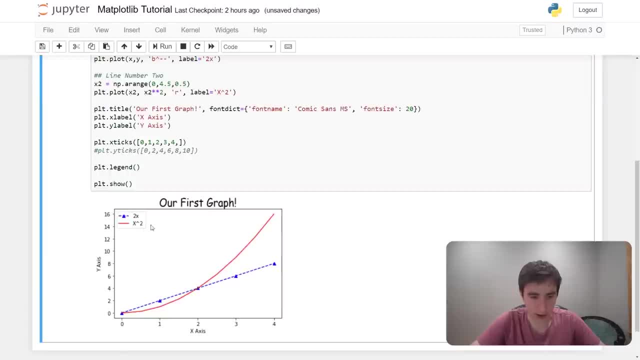 And one thing that's cool is that it automatically moved this legend to the top left because the positioning was better. now that this goes up to the top right, All right, so we have two lines up there And from the original image I showed. 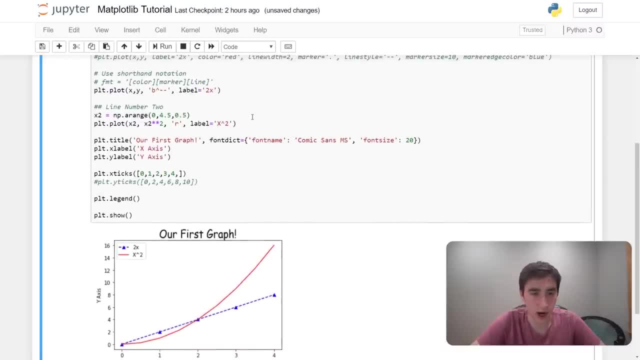 there's some stuff that's still different. One thing that's kind of cool that you could do is, let's say, you had a graph that stopped, but you wanted to kind of show the projection of it in the future. So what I did to show it? 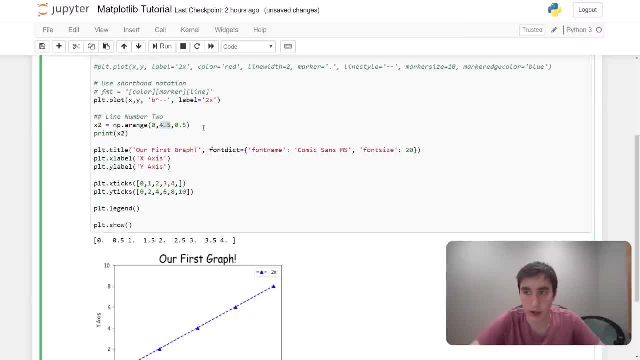 So we have that, So that's going to be our Xs, And so what I can do here is I can go ahead and plot that And I'm going to plot the square function for it. So I'm going to pass an X2.. 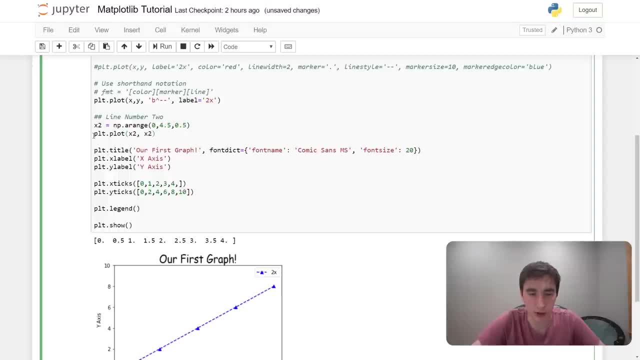 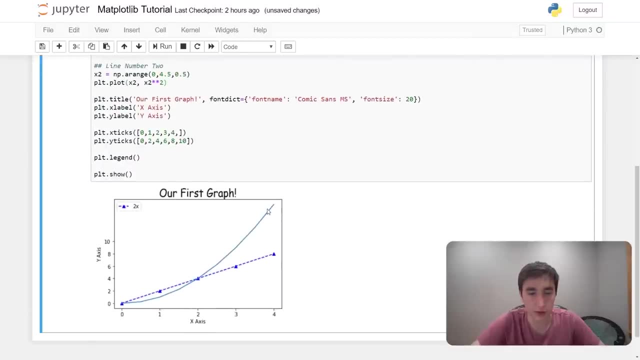 And then, instead of passing in a Y, I'm just going to do X2.. And then I'm going to do squared What happens here? So now you see, we get X2 squared. It goes a little bit higher than our original axis was set. 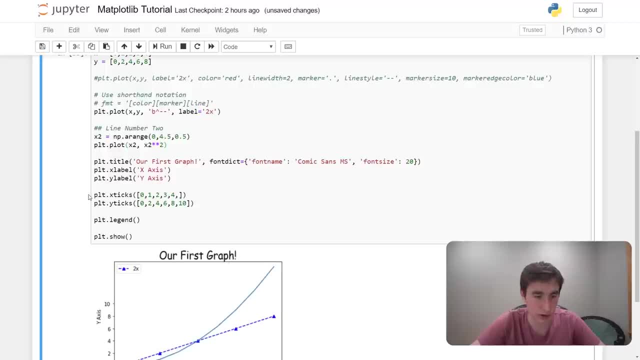 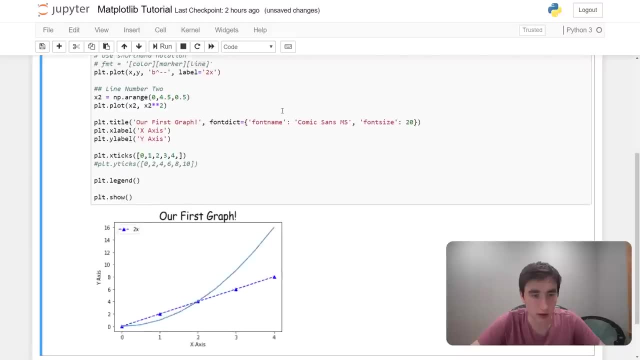 so I'm going to change up the ticks, Or maybe I'll just kind of comment this out and see what happens for our tick marks. Yeah, I'm fine with just leaving the default that it gave us. It looks good to me And now we have two blue colors. 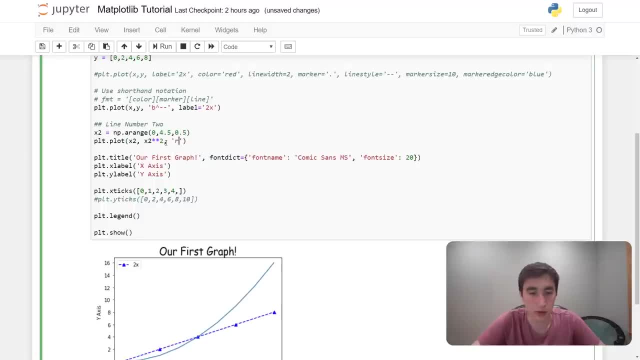 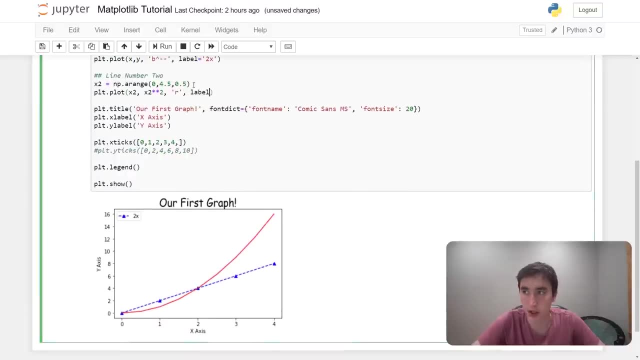 so let's make this a different color. Maybe we can make it red. We want to give it a label as well, So I'm going to do red And I'm going to say: the label is equal to X squared. And one thing that's cool is that it automatically moved this legend. 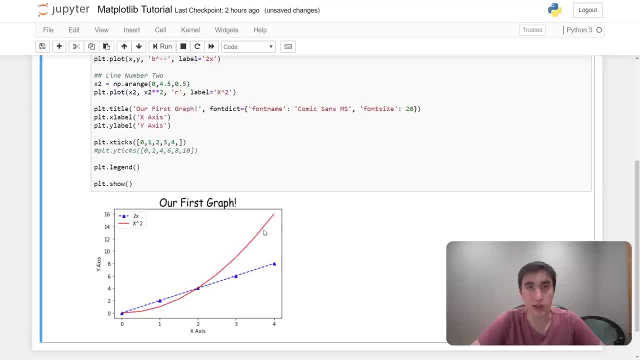 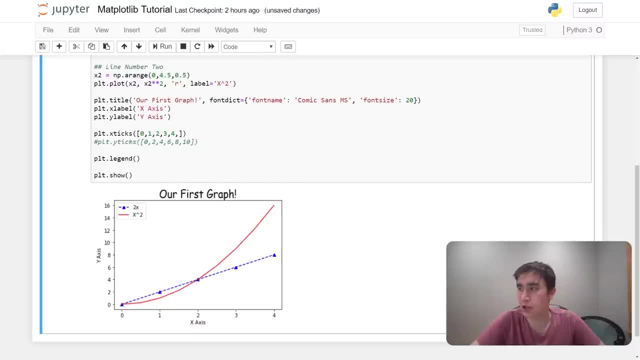 to the top left because the positioning was better now that this goes up to the top right. So we have two lines up there And from the original image I showed there's some stuff that's still different. One thing that's kind of cool that you could do. 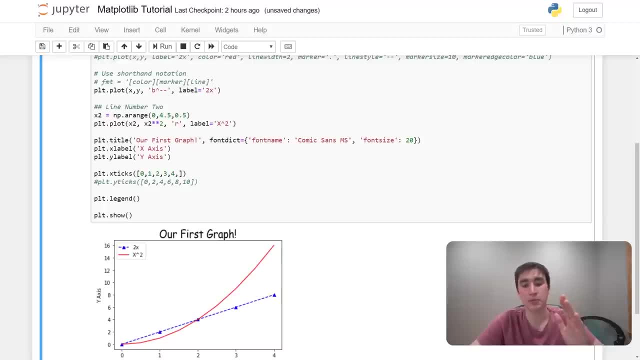 is, let's say, you had a graph that stopped, but you wanted to kind of show the projection of it in the future. So what I did to show that type of a phenomenon is: I did like X2, take the first four values here. 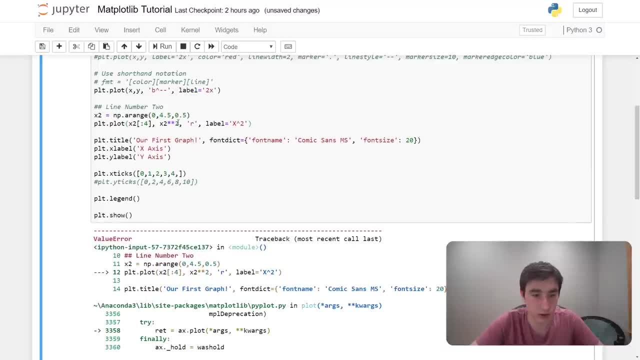 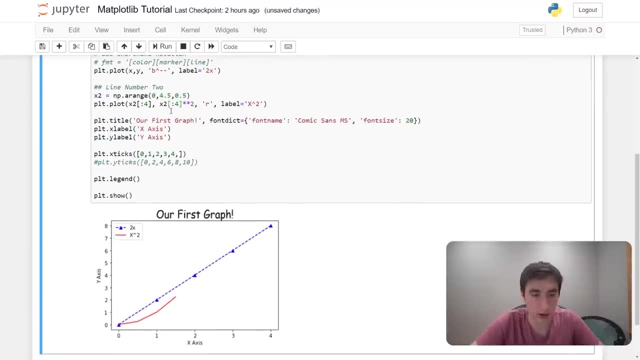 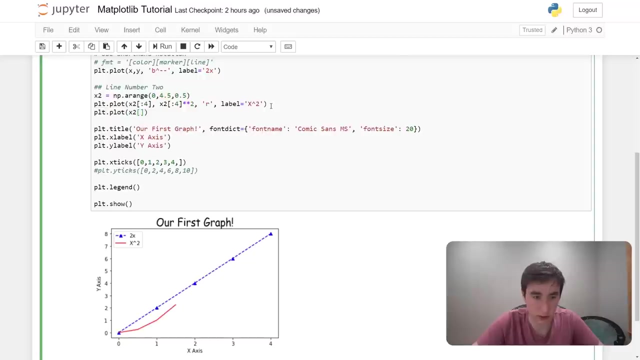 and we'll plot that. What did I do? Oh, shoot First four. Is that what I want? I think that will work. Take the first four and plot that, And then for the last values, so from, let's say, five or three. 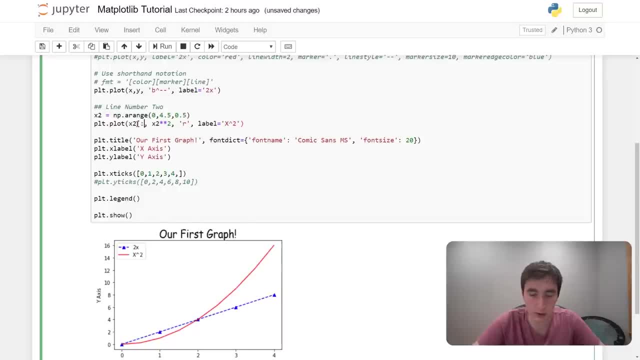 show that type of a phenomenon is. I did, like X two, take the first four values here and we'll plot that. Ah, what did I do? Oh, shoot First four. Is that what I want? I think that will work. 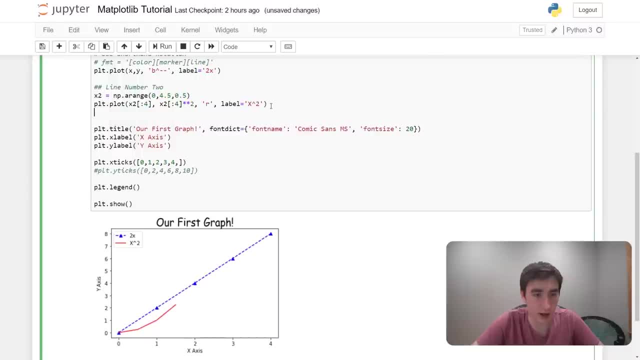 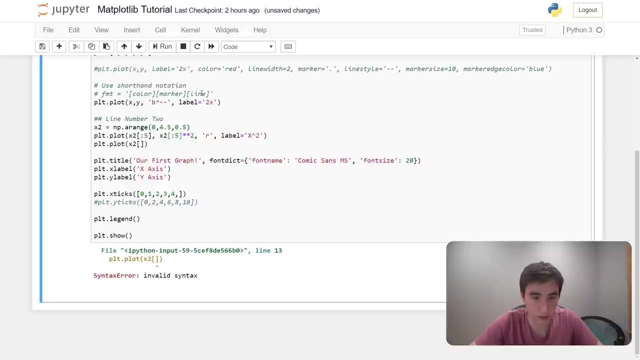 Take the first four and plot that, And then for the last value, I'm going to take the last values, So from let's say, five or three, or let's make this a little bigger, Make this six or five. Bear with me here. 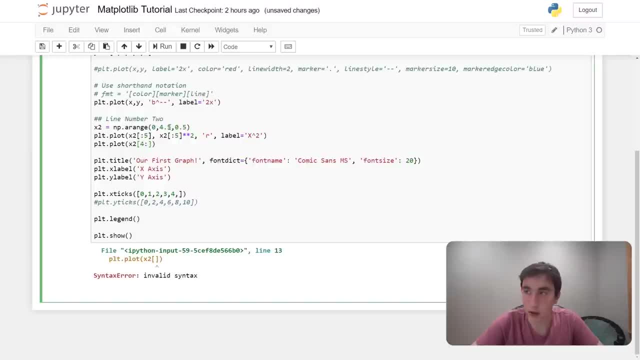 From four onward, we'll make it six. We'll make it a dashed line And I had a little bit of overlap because I think it'll look better. You'll see in a sec. Four dash: We'll make this. still the same function. 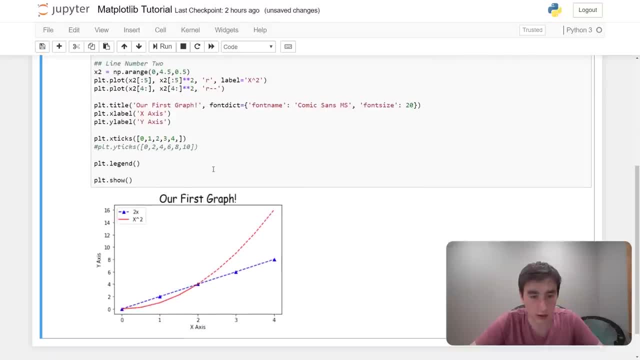 but this time we're going to make it a dashed line. So there you see- and I'm going to actually make this a little bit different- There you see, like maybe something ended here and then you make it a dashed line, dashed the rest of the way. you could do something like that using the format I just showed. 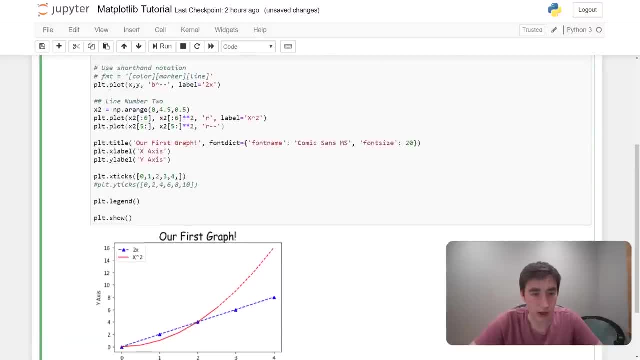 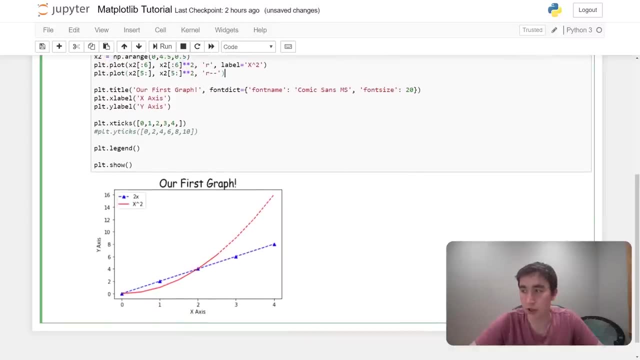 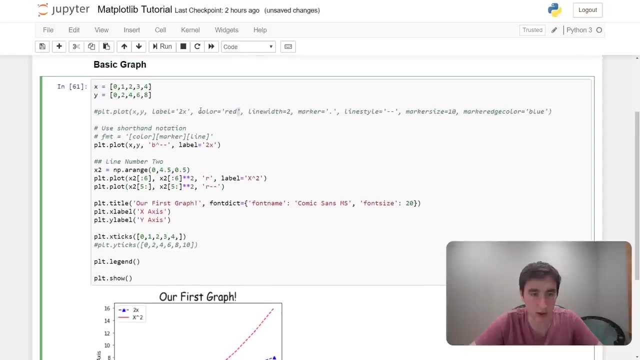 all right, what else do we have? probably clean this code up a little bit. another thing that I showed in the original graph that I showed when I was introducing this video was a resize. so let's say we wanted to resize our graph. well, we should do that probably near the top of our graph. so I'm 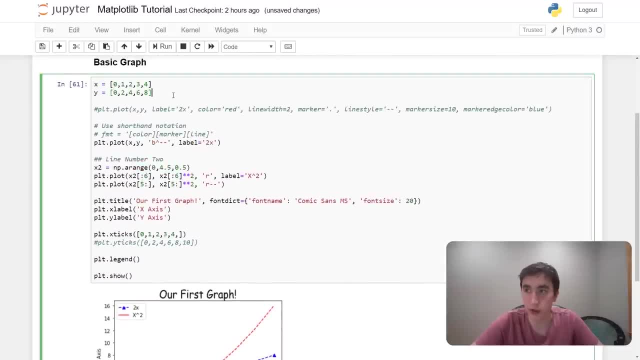 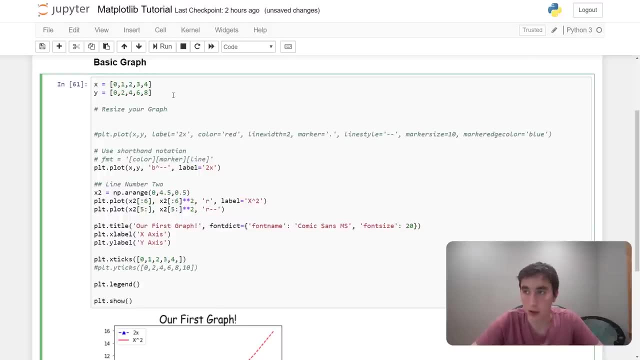 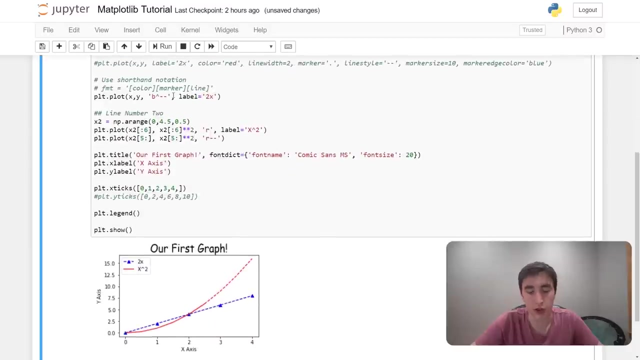 going to go ahead and do resize your graph. I'm going to go ahead and do plot bigger passing fig size and we're gonna say let's make the dimensions 5x3. it's kind of an arbitrary five by three that will give you kind of the ratio of your X to your y, but to specify how many pixels it is, youendi. 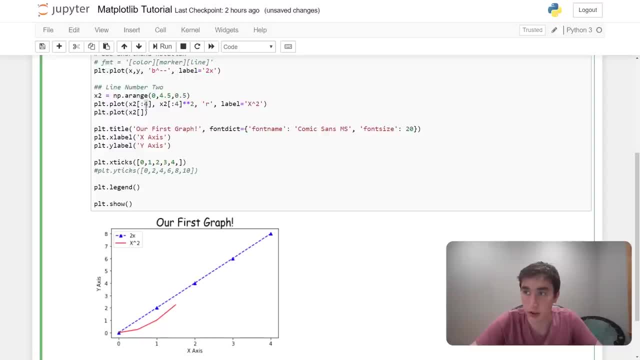 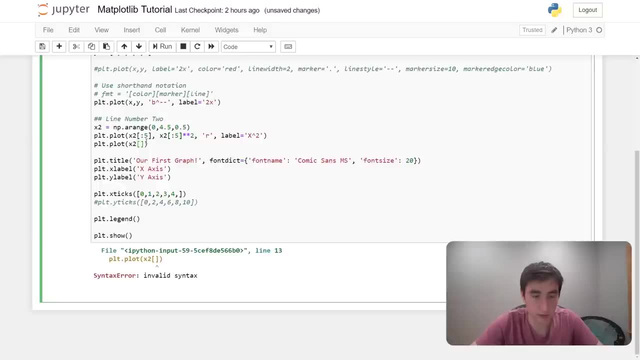 Let's make this a little bigger, Make this six or five. Bear with me here. From four onward we'll make it a dashed line And I had a little bit of overlap because I think it'll look better. You'll see in a sec. 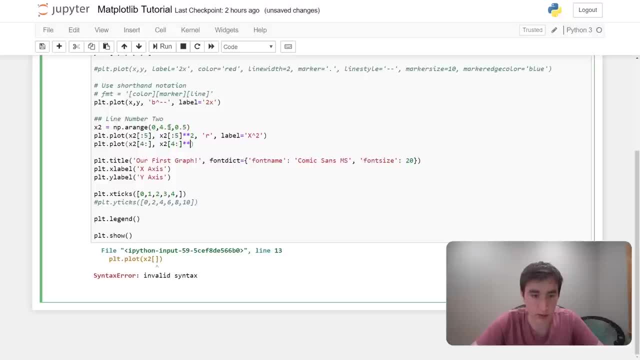 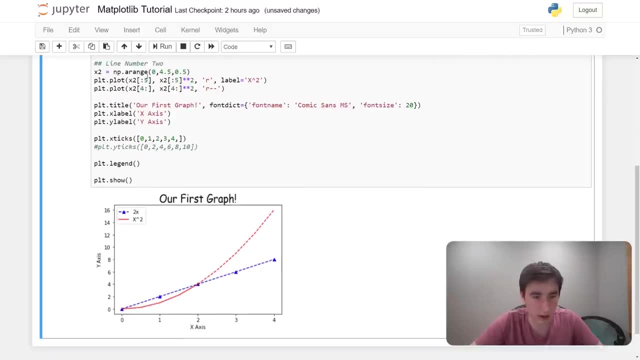 Four dash. We'll make this still the same function, but this time we're going to make it a dashed line. So there you see, and I'm going to actually make this a little bit different. There you see, like maybe something ended here. 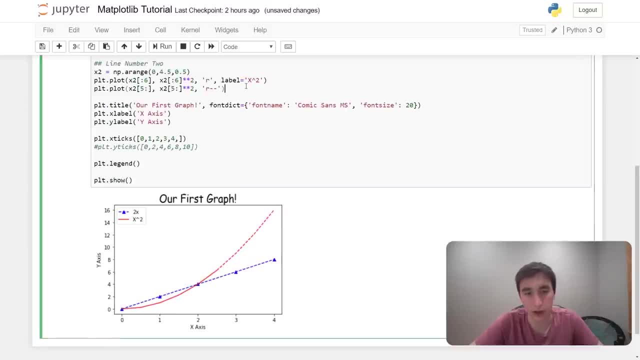 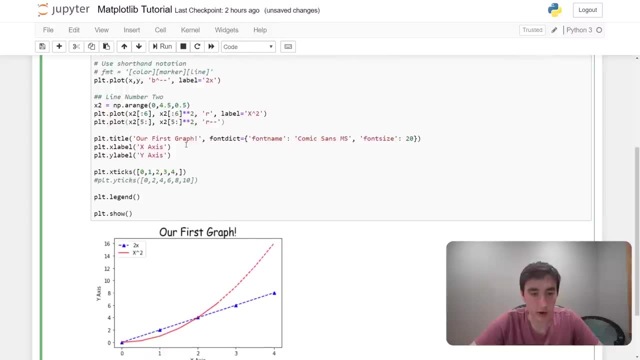 and then you make it dashed the rest of the way You could do something like that using the format I just showed. All right, What else do we have? I'll probably clean this code up a little bit. Another thing that I showed in the original graph: 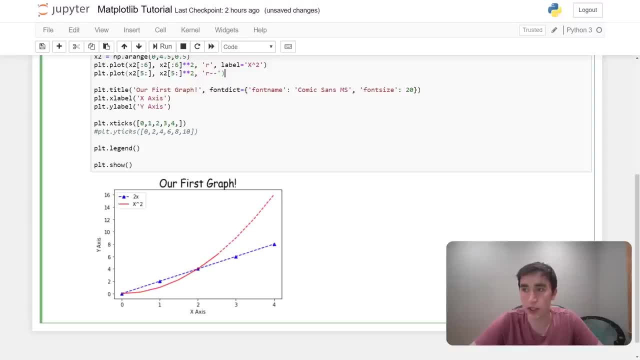 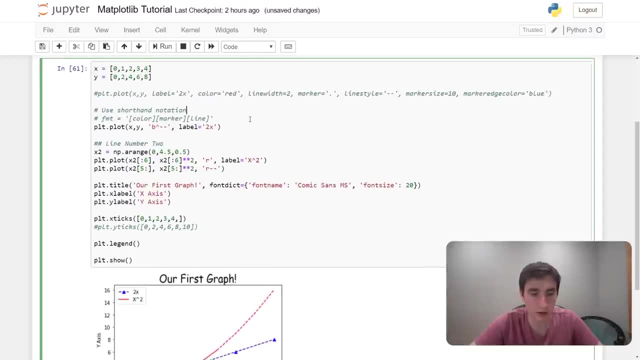 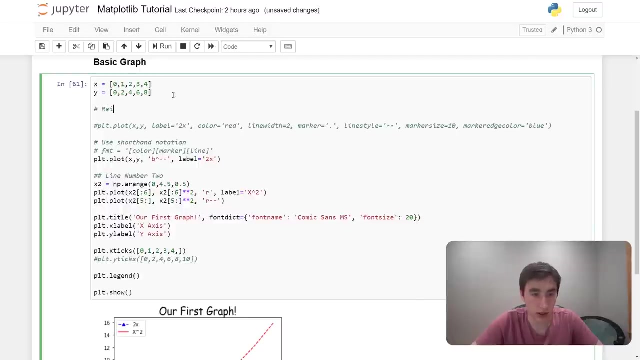 that I showed when I was introducing this video was a resize. So let's say we wanted to resize our graph. Well, we should do that, probably near the top of our graph. So I'm going to go ahead and do resize your graph. 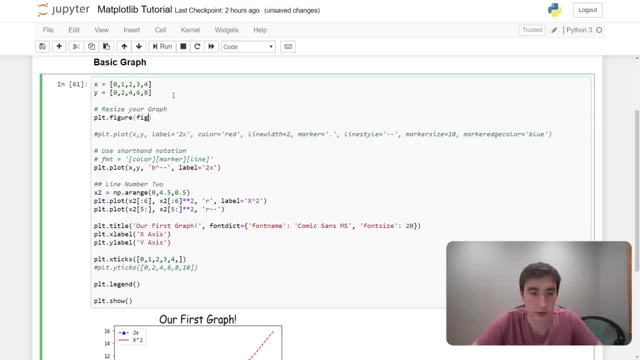 I'm going to go ahead and do plot dot, figure Pass in fig size And we're going to say let's make the dimensions five by three. It's kind of an arbitrary five by three That will give you kind of the ratio of your X to your Y. 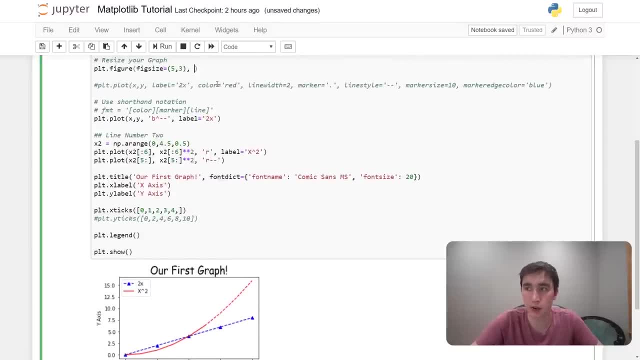 But to specify how many pixels it is, you're going to want to pass in a second parameter, which is DPI, which basically is pixels per inch. So I recommend using a value of around 300 here. If you do smaller values, you'll have more pixelated graphs. 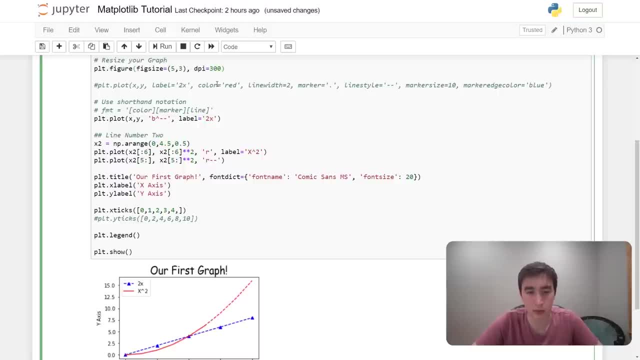 So if you can afford having a bigger image, having a bigger DPI is often nice. So in this case we have pixels per inch of 300.. So this is going to actually be five inches by three inches, So the total pixels will be 1500 by 900 here in this graph. 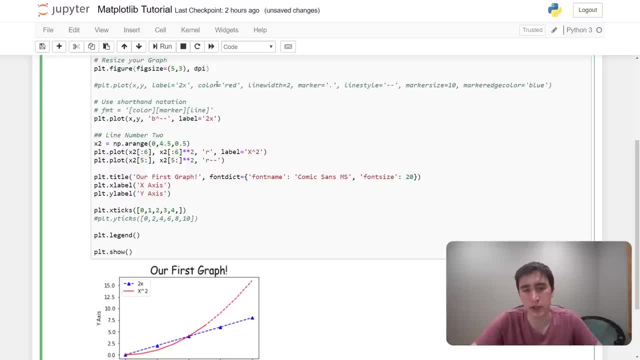 want to riding ziemlich dsright. so for our large size, we want to come back and go ahead and and pass in a second parameter, which is dpi, which basically is pixels per inch. so i recommend using a value of around 300 here. if you do smaller values, you'll have more pixelated graphs. 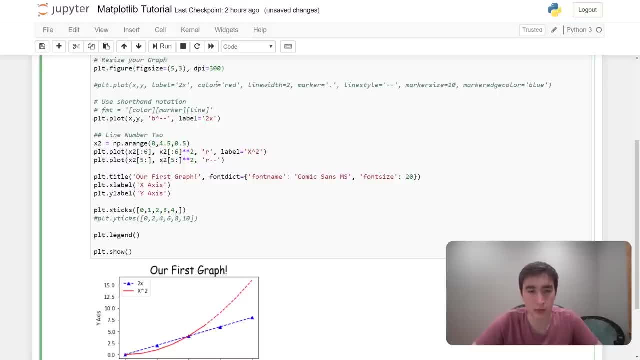 so if you can afford having a bigger image, having a bigger dpi is often nice. so in this case we have pixels per inch of 300, so this is going to actually be five inches by three inches, so the total pixels will be 1500 by 900 here in this graph. so now it's much, much bigger. maybe it's a. 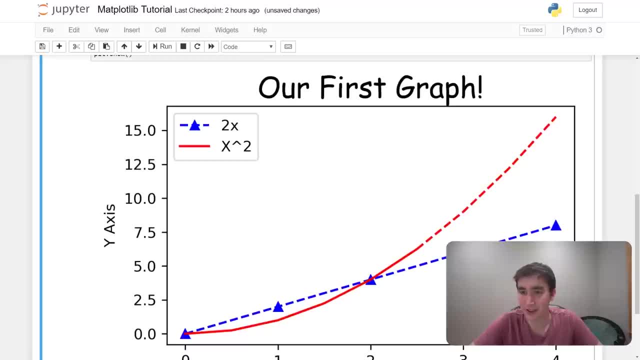 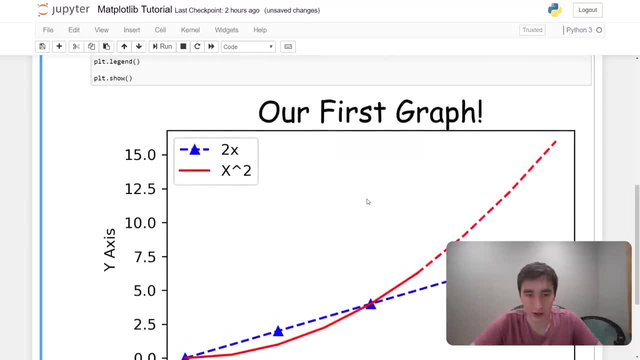 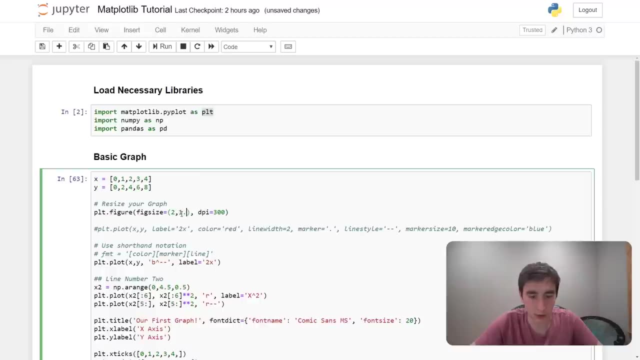 little bit too big. um, i didn't. i'm going to be blocking this graph, so i'm going to make it a little bit smaller. but you get the idea then here, so i'll make it like 2 by 1.5. that's not a good dimensions now, though. 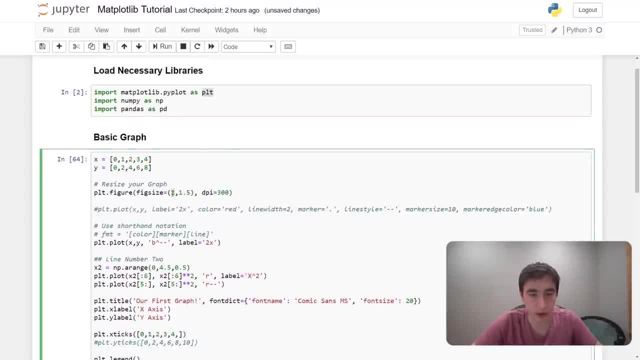 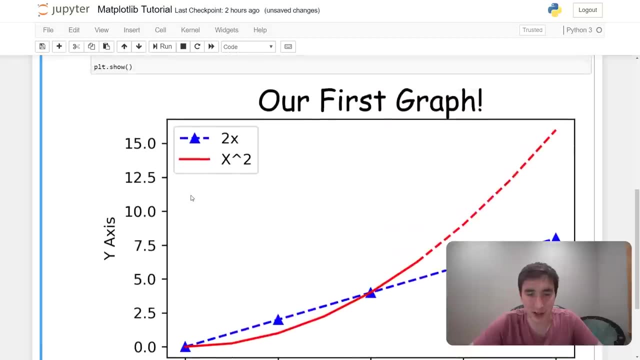 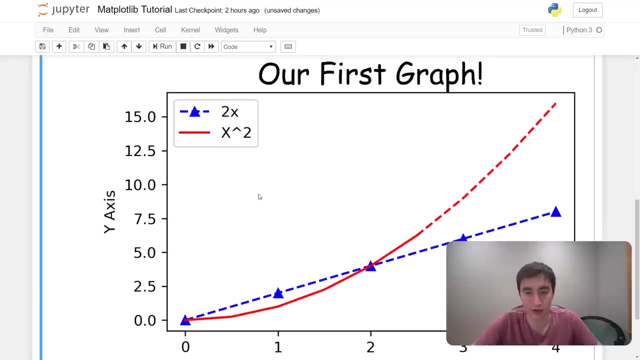 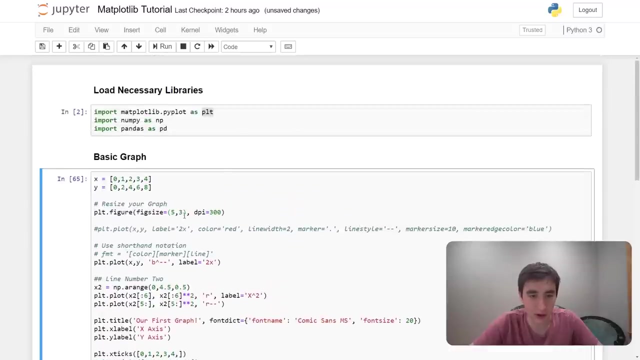 i mean just play around with this. the the biggest issue i have right now is the graph looks so big because, um, i have my screen super high resolution or super. the view is like very up close because i want to make sure you guys can see my code. but yeah, this would be a 1500 by 900 graph. 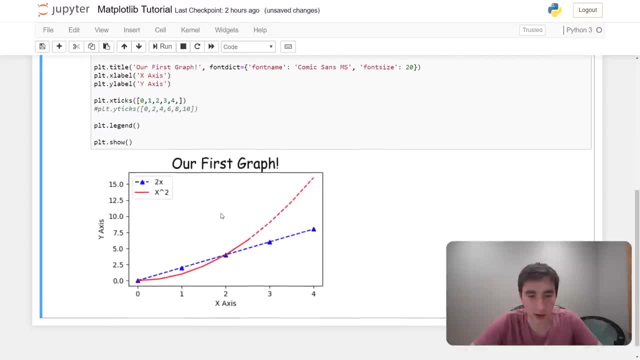 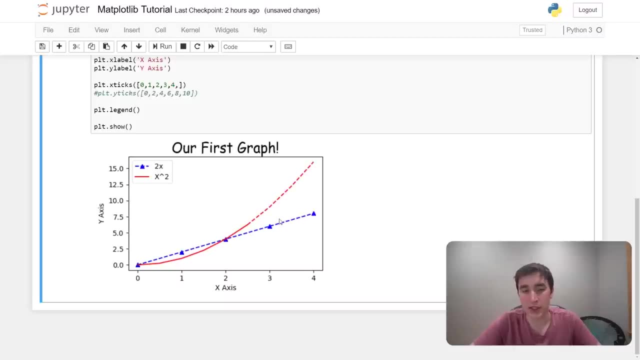 i'm going to, just for the sake of the graph, decrease the dpi and make it more reasonable the the issue. you can't really tell from this image, but if you really zoom into the graph and maybe, if you like, printed the graph out, it would look maybe a little bit pixelated with a dpi of 100. so probably try to keep this value. 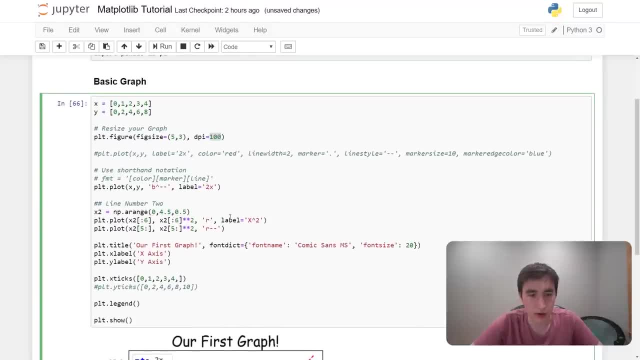 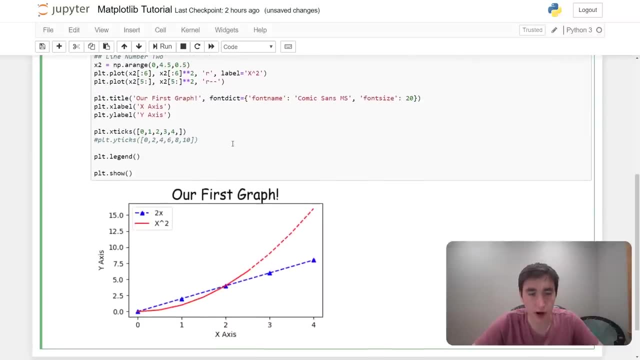 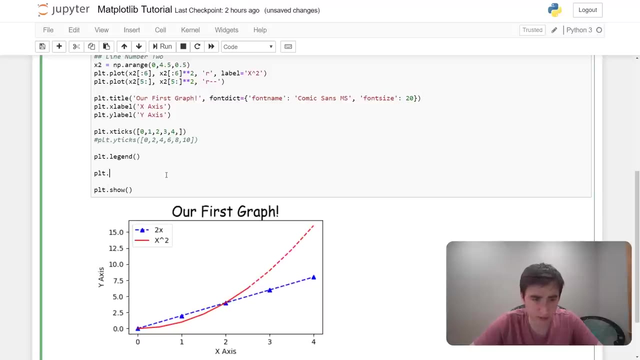 higher if possible. and then another thing you want to do is you'll want to save your graph. so to save, we can do plot dot, save fig, and we can do say my graph dot png. and one thing that's nice too is i could pass in the dpi parameter here as well. so let's say, when i actually saved my graph, i 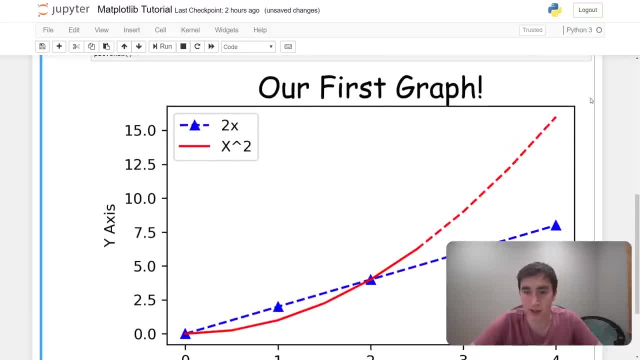 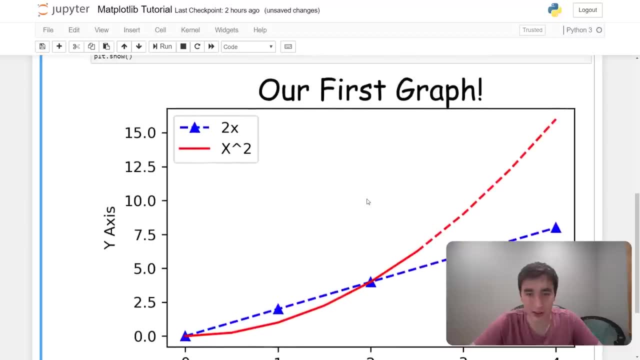 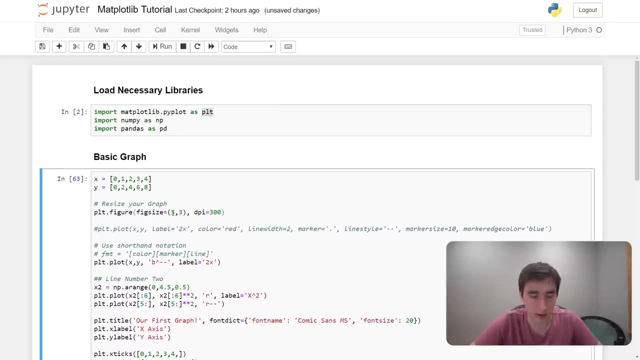 So now it's much, much bigger. Maybe it's a little bit too big. I'm going to be blocking this graph, So I'm going to make it a little bit smaller, But you get the idea then here. So I'll make it like two by 1.5.. 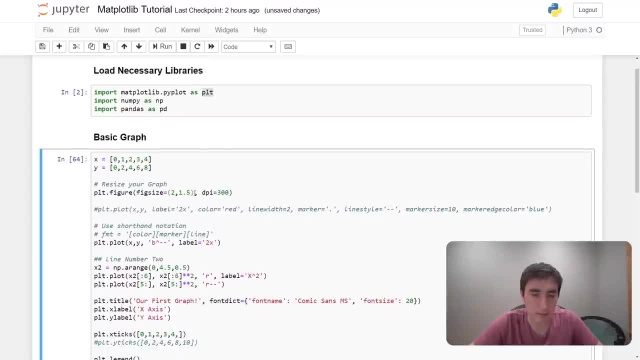 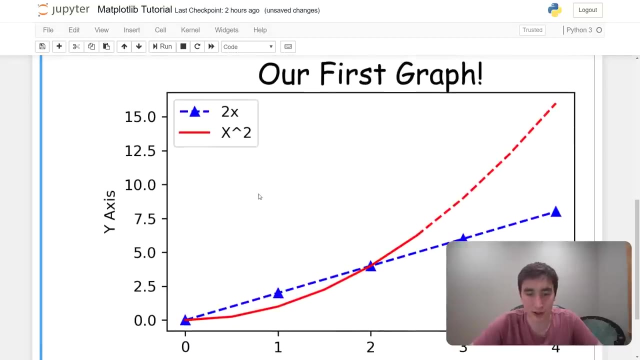 That's not a good dimensions. now, though, I mean just play around with this. The biggest issue I have right now is the graph looks so big because I have my screen super high resolution or super. the view is like very up close because I want to make sure you guys can see my code. 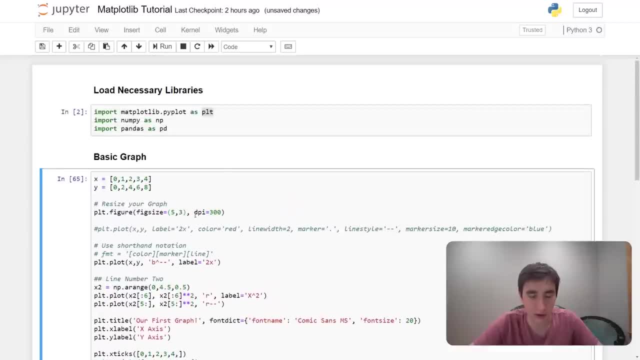 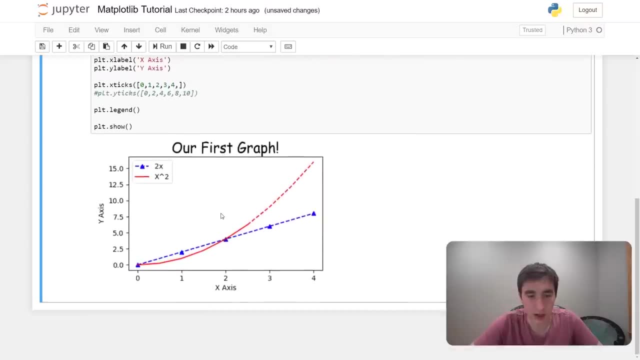 But yeah, this would be a 1500 by 900 graph. I'm going to, just for the sake of the graph, decrease the DPI and make it more reasonable The issue. you can't really tell from this image, but if you really zoom into the graph. 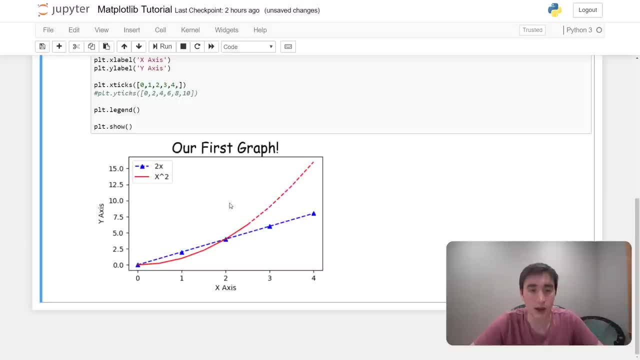 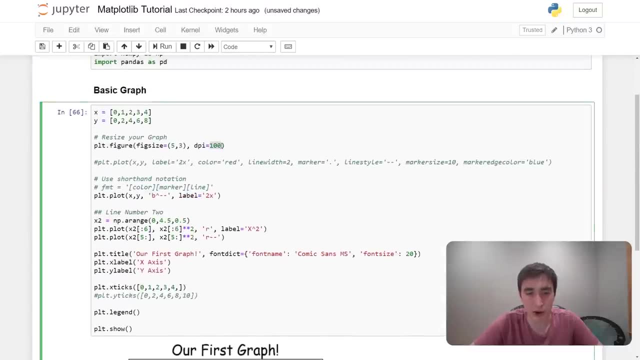 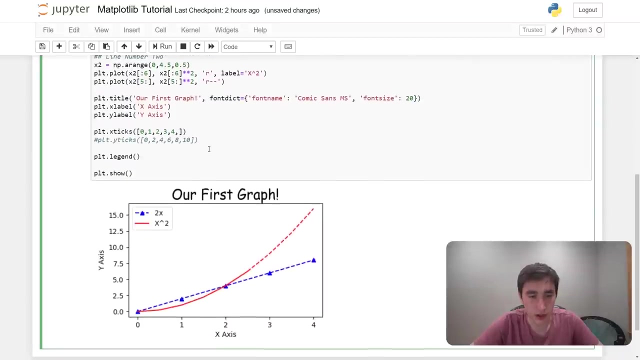 and maybe, if you like, printed the graph out, it would look maybe a little bit pixelated with a DPI of 100.. So probably try to keep this value higher if possible. And then another thing you want to do is you'll want to save your graph. 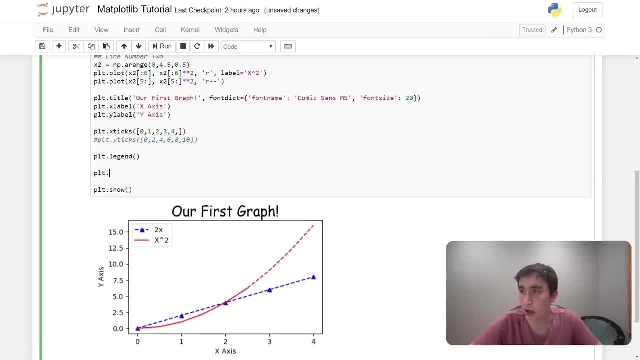 So to save, we can do plot dot, save fig, And we can do, say, by graph dot PNG. And one thing that's nice too is I could pass in the DPI parameter here as well. So let's say, when I actually save my graph, 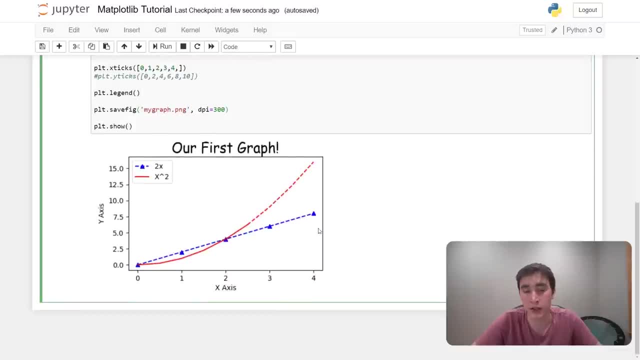 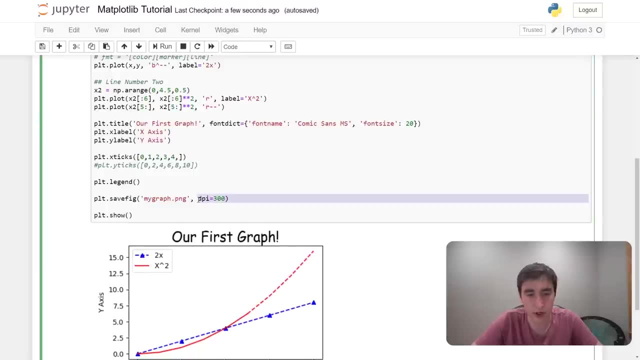 I want it to be bigger, But for the sake of being able to show you guys it in a smaller format, I wanted the 100 above. I can still go ahead and save it with 300 and then kind of solves both my problems. 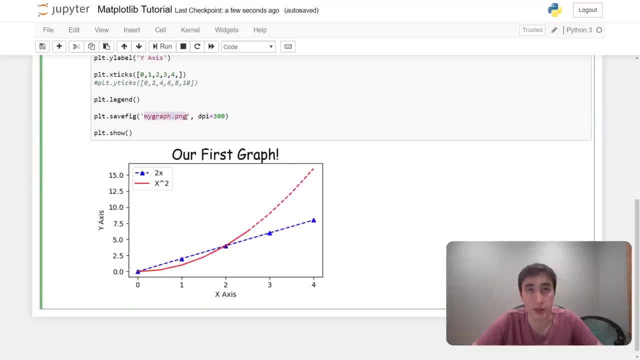 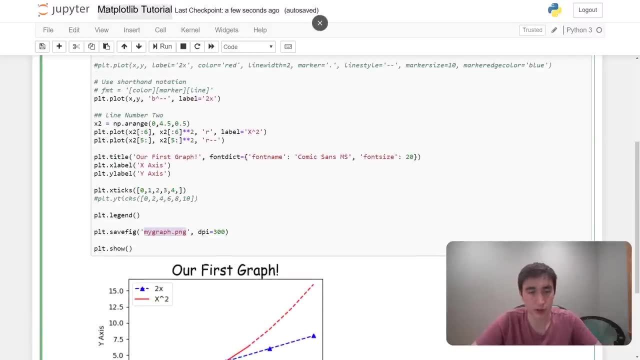 And so this then my graph dot PNG will save in the current directory that this matplotlib tutorial is in. Yeah, it will save in that current directory, The current directory, whatever directory your file matplotlib tutorial is in, this graph will also save there when we run this. 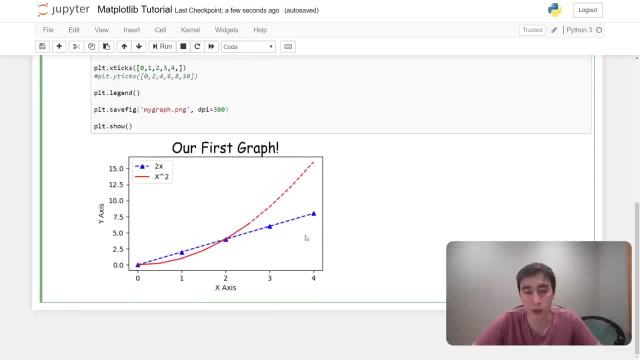 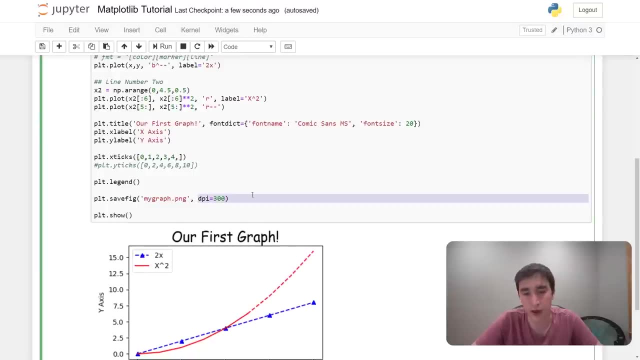 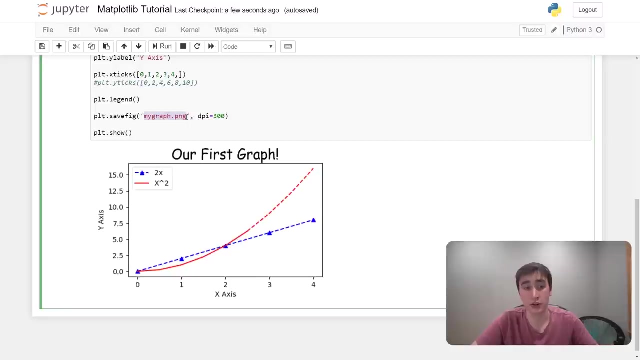 wanted to be bigger but for the sake of being able to show you guys, it's going to be a little bit bigger in a smaller format. i wanted the 100 above. i can still go ahead and save it with 300 and then kind of solves both my problems and so this, then my graphpng will save in the current directory that. 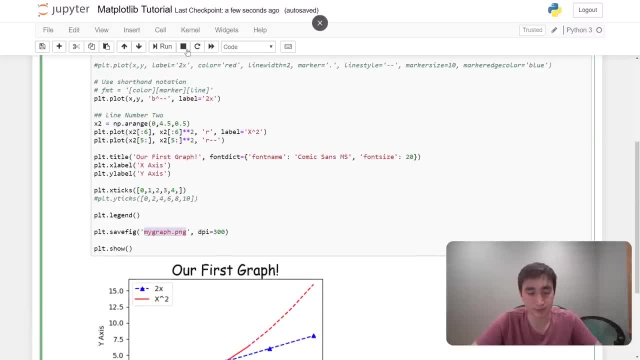 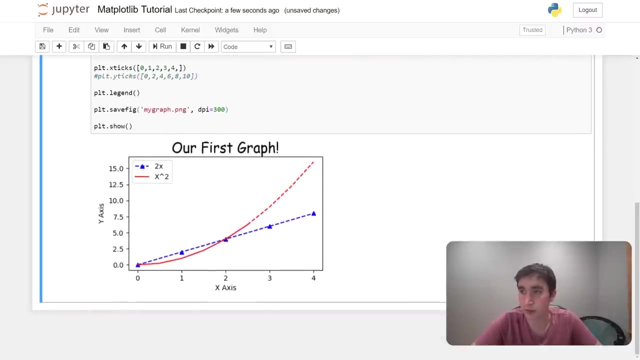 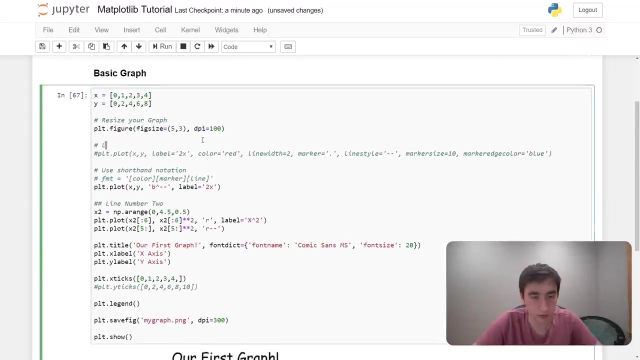 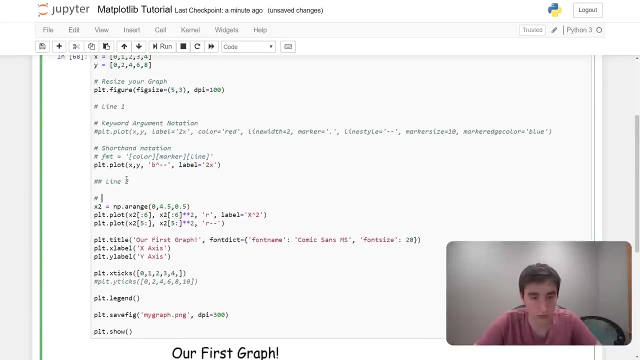 this matlab matplotlib tutorial is in. it was, yeah, saving that current, the current director, whatever, whatever directory your file matplotlib tutorial is in this graph will also save there when we run this. cool, now we have that saved. all right, let me clean this up a little bit and just to note the reason i did this is because this is exclusive, this x here. so when i do the 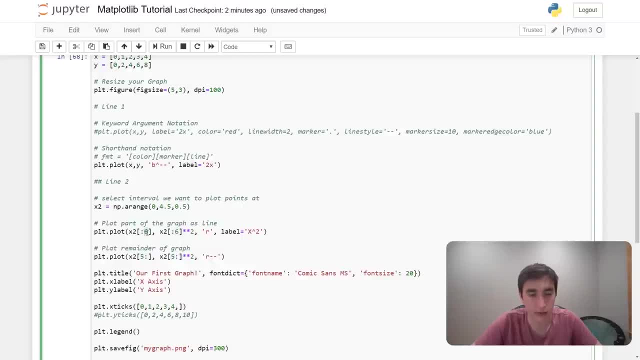 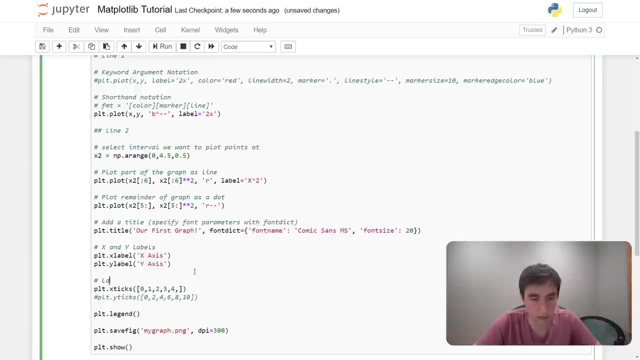 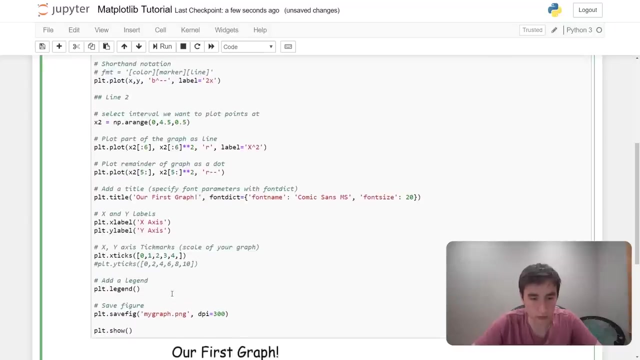 5 onwards. it picks up. this actually ends at 5 because it doesn't include 6, so it actually covers everything here. so I'm just going to go ahead and do a little bit more of that. so i'm just going to go ahead and do a little bit more of that. 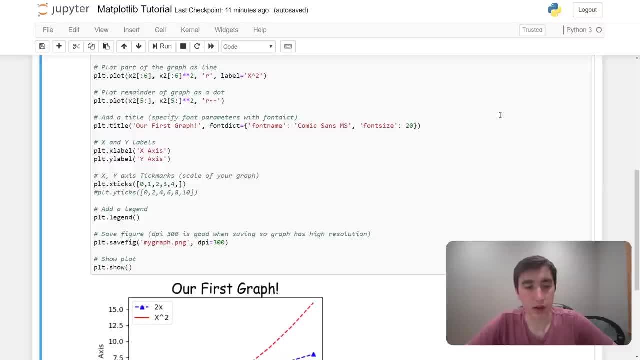 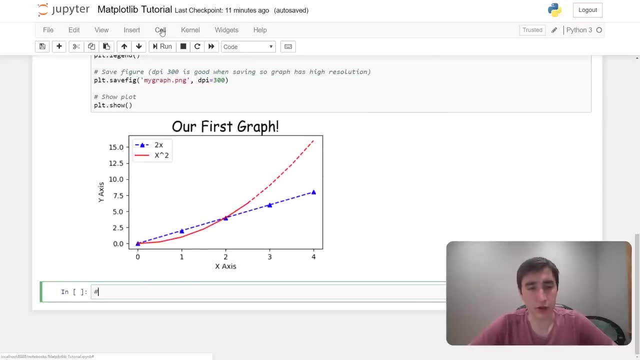 so i'm just going to go ahead and do a little bit more of that. all right, now that we've shown line graphs a bit, let's go and do quickly do bar charts, and after bar charts, i think we're going to just end this video short and i'll do the real world examples in a video that i'll post next week. i just think. 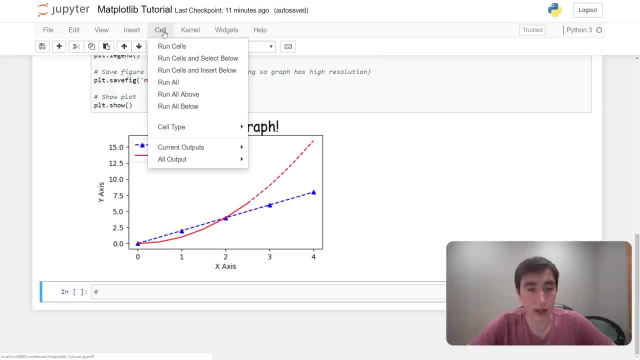 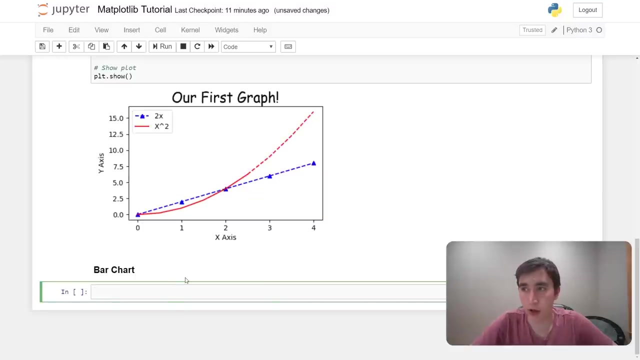 this video might get a bit too long if i include everything in just one video. so all right, so i want to do bar chart, okay, so bar charts are pretty straightforward as well. let's say we had some labels- a, a, b and c- and some values. let's say 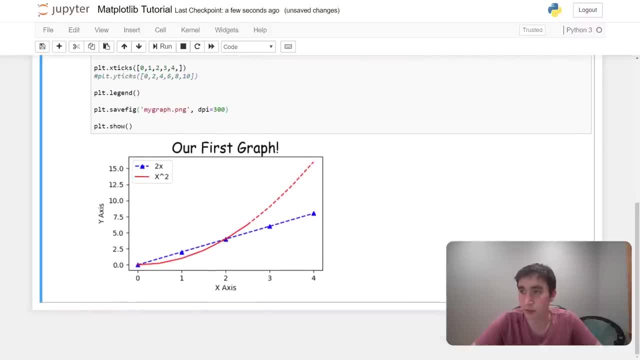 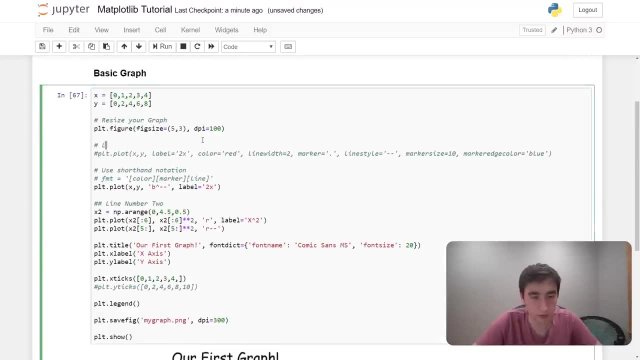 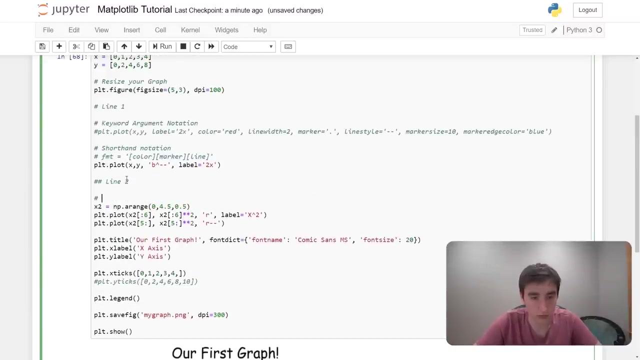 Cool, Now we have that saved. All right, let me clean this up a little bit. And just to note: the reason I did this is because this is exclusive to six here, So when I do five onwards, it picks up. this actually ends at five. 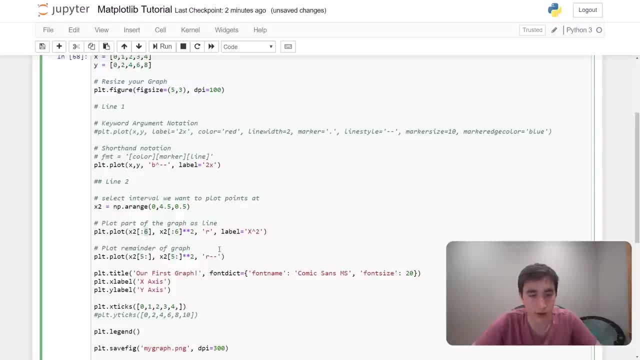 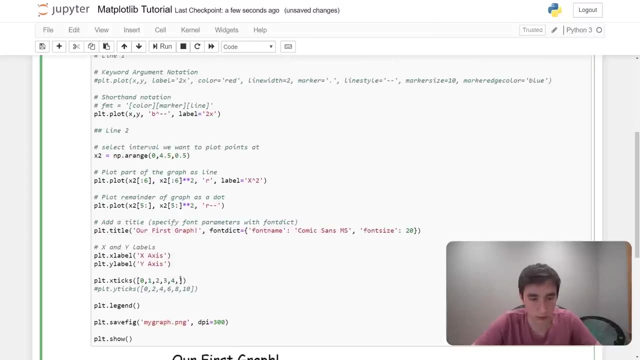 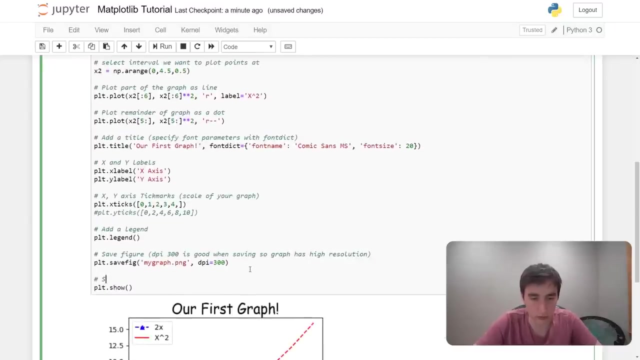 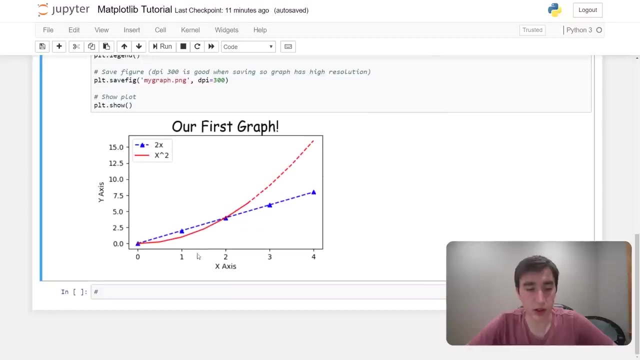 because it doesn't include six. So it actually covers everything here. All right, Now that we've shown line graphs a bit, let's go and do quickly do bar charts, And after bar charts, I think we're going to just end this video short. 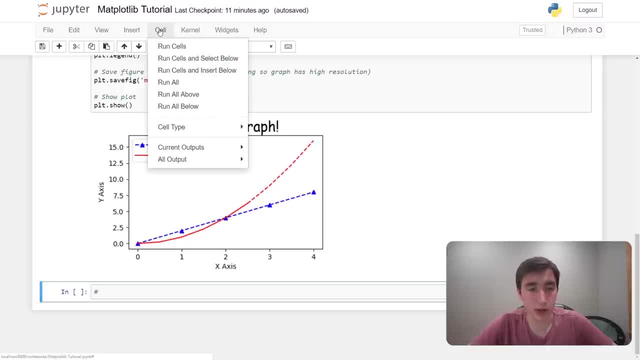 and I'll do the real world examples in a video that I'll post next week. I just think this video might get a bit too long if I include everything in just one video. So all right, So I want to do bar chart. 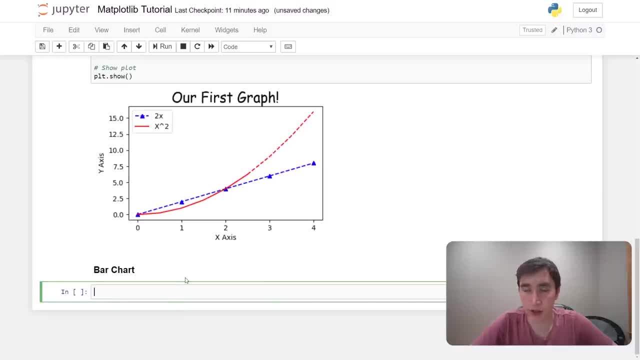 Okay, So bar charts are pretty straightforward as well. Let's say we had some labels- A, A, B and C- And some values, let's say one, four and two. Well, if we wanted to do a bar chart, 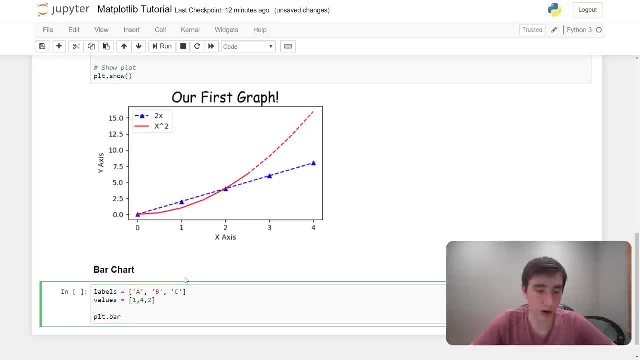 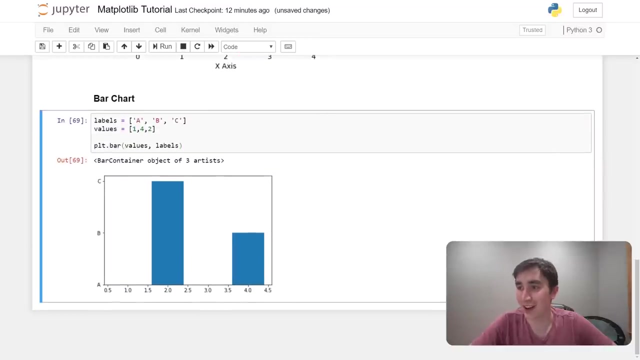 we could just do plotbar of labels, comma values. I probably did that wrong. It's values, comma labels, And we get not what I was looking for. Okay, Let's see, It is actually labels first. 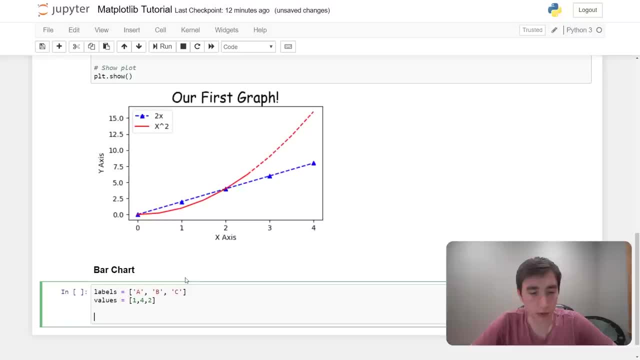 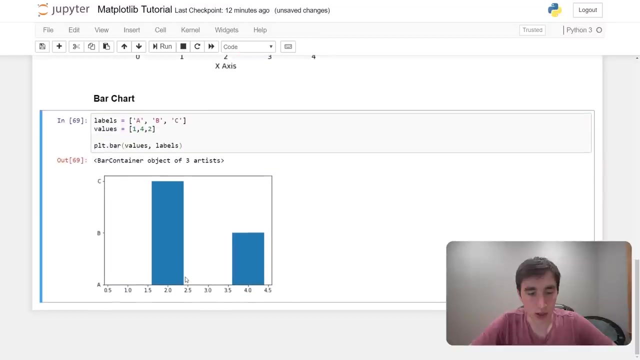 one, four and two. well, if we wanted to do a bar chart, we could just do plot dot bar of labels, comma values. i probably did that wrong. it's values, comma labels, and we get not what i was looking for. uh, okay, let's see. um, it is actually. 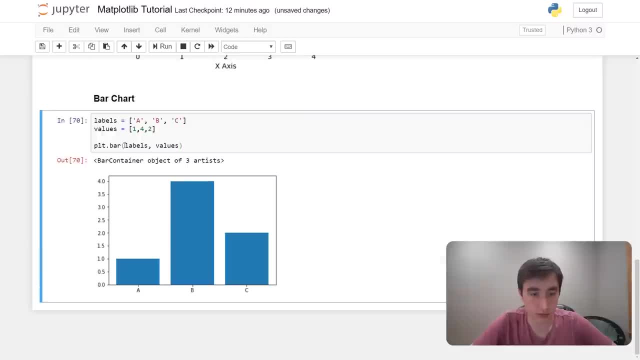 labels first, then values a, b, c, cool, so that was pretty straightforward and i can do the plot dot show and a bit smaller and the bar gap becomes smaller now so that you have a log. i can do all the small things that are that. are you really want to get there all sudeck matrix? so you have it now. 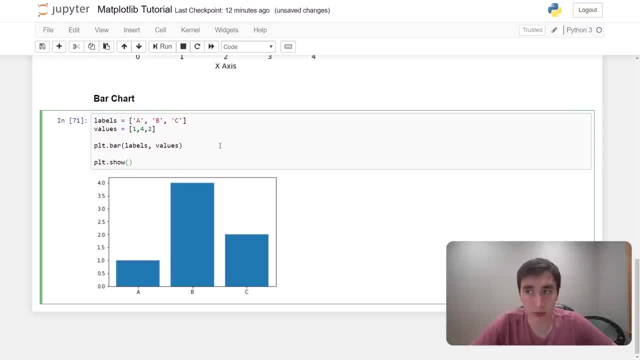 i can shift up five. it doesn't matter, it doesn't have to be several. all changes up is a little bit up to you, so let's save that up. we can do all the adding of titles and whatnot the same way as before in the line graph example. 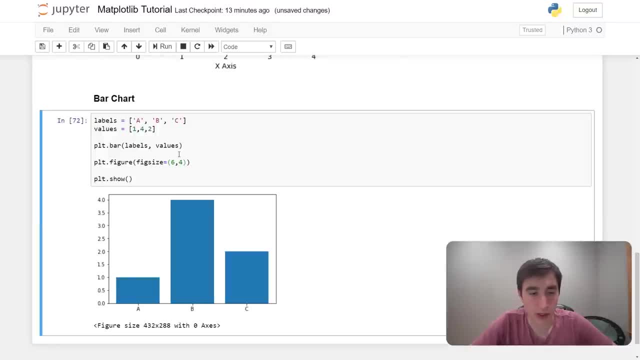 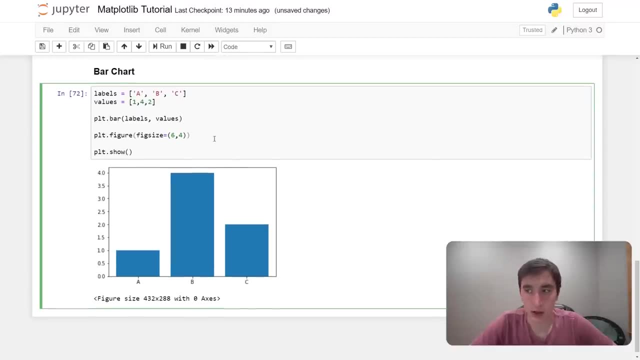 it's going to use, whatever the default DPI is. and then one thing that's cool that you can do with bar charts is you could add different patterns to these. so to do that- and you can, you can really play around with the documentation, do all sorts of different things. I do some kind of following the graphs that I was. 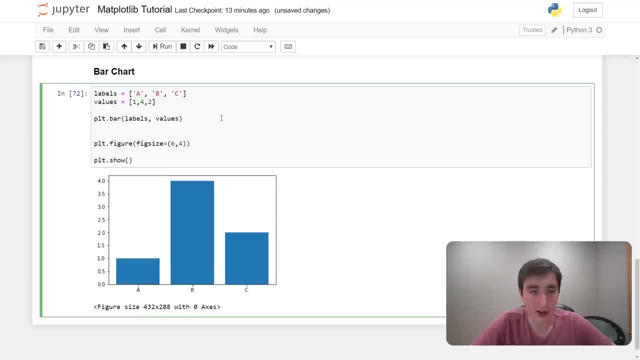 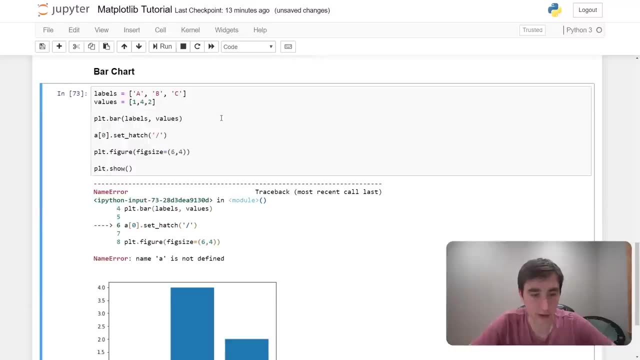 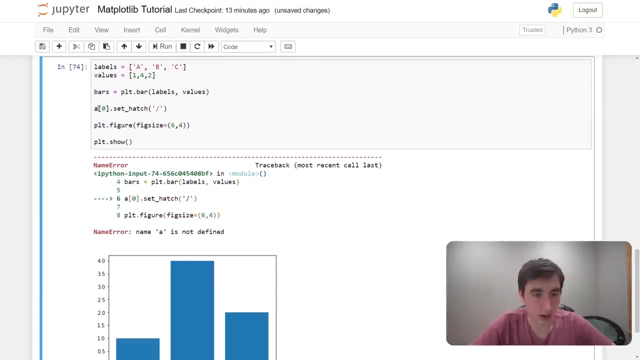 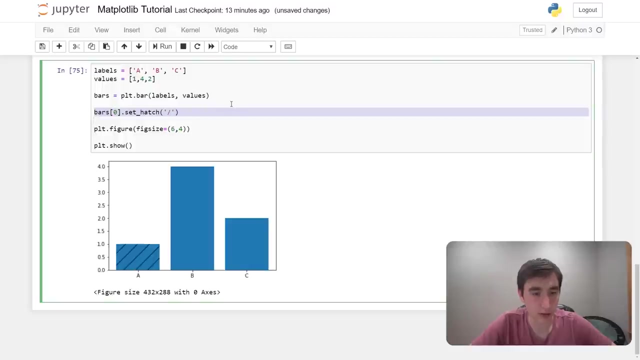 showing the inner intro of my video. so I wanted to just show kind of what different hatch values look like. so I can make the first one have, I'm gonna say, bars, equal plot of ours. there we go. now I do bars, zero, set hatch. that's gonna give me the lines that you see down here. I can do the same thing with. 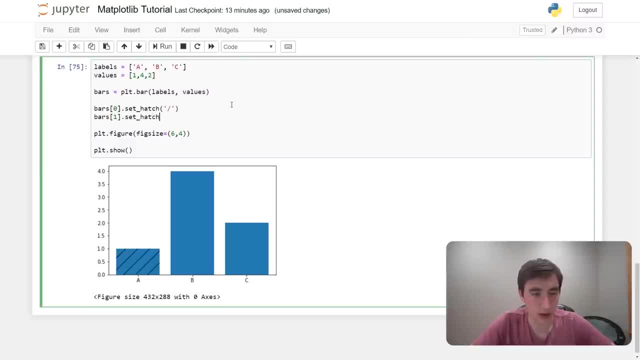 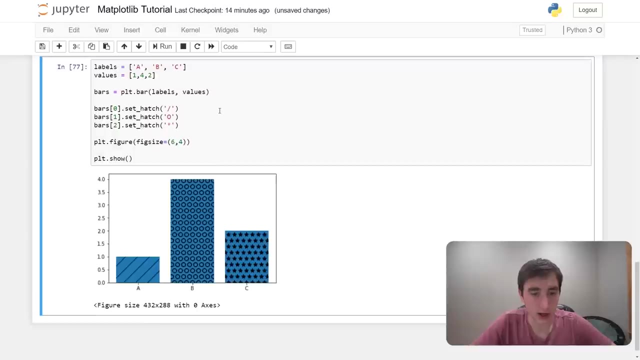 the second value. let's make this circles, and you can find all the hatch values in the documentation as well. let's do the third value. we'll do stars. so now you get kind of a cool little bar chart. I can also add a legend to this very easily, and this will tell me right away. 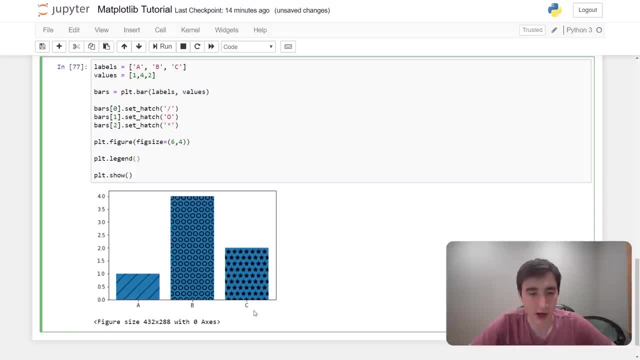 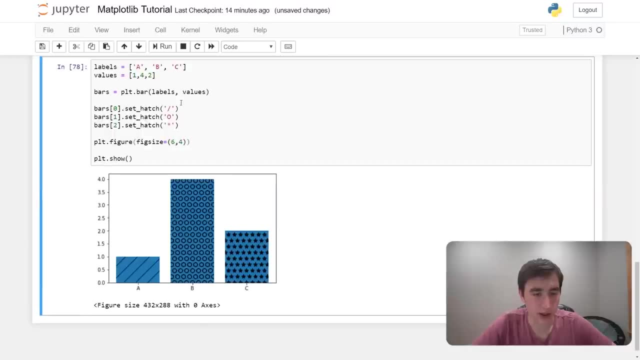 we have a, B and C, but I mean they're labeled right here, so legends probably not necessary in this case. all right, let's see what else did I want to do with this. and then, if you wanted to make this a little bit neater, if you had like. 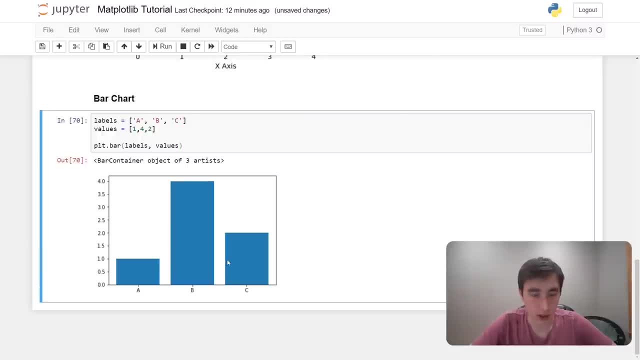 then values A, B, C, Cool. So that was pretty straightforward And I can do the plotshow. We can do all of the adding of titles and whatnot the same way as before in the line graph example. Let's skip over that for now. 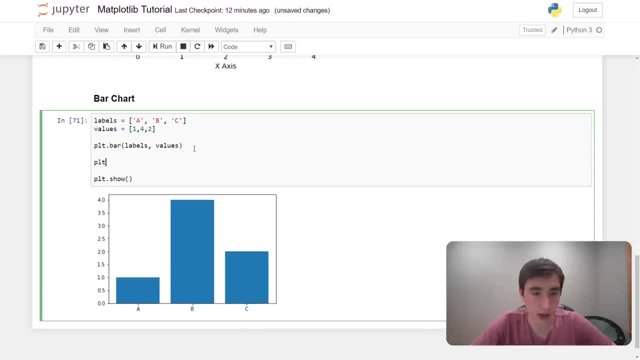 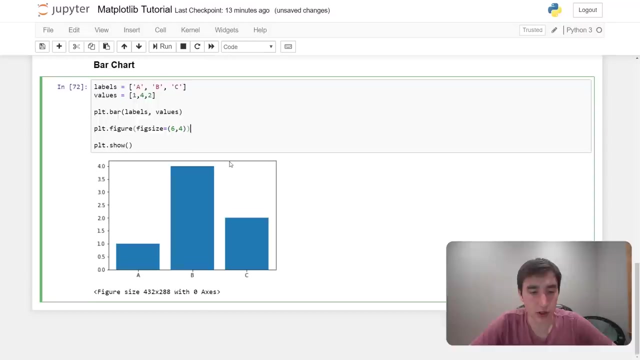 I could also resize it, let's say So I could do plotfigure fig size equals, let's say, six by four. It's going to use whatever the default DPI is. And then one thing that's cool that you can do with bar charts. 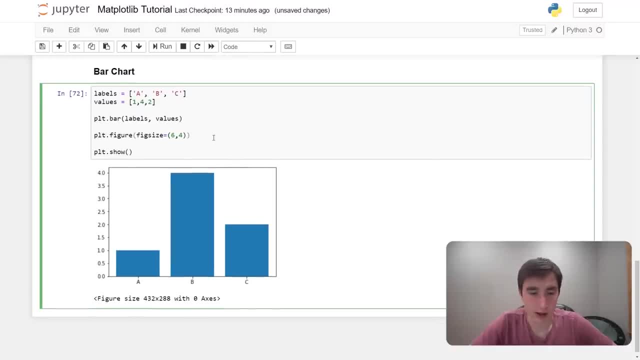 is, you could add different patterns to these. So to do that- and you can really play around with the documentation, do all sorts of different things. I just am kind of following the graphs that I was showing, showing the intro of my video. 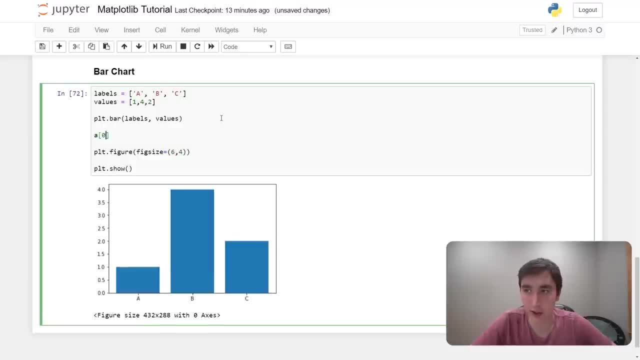 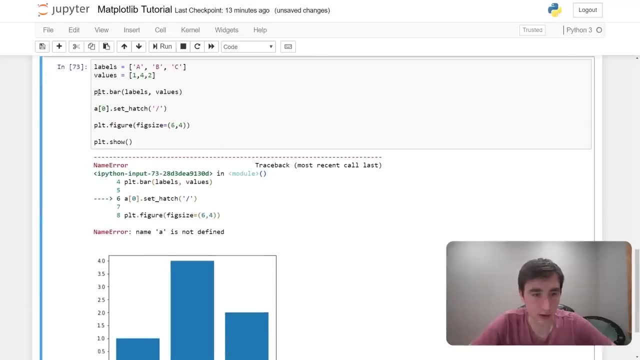 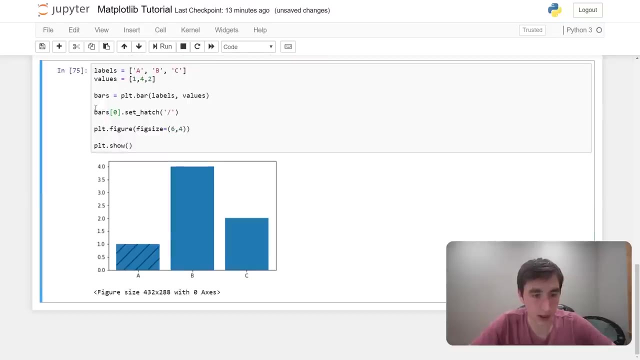 So I wanted to just show kind of what different hatch values look like. So I can make the first one have, I'm going to say, bars equal plotbars. There we go. Now I do bars zero set hatch. That's going to give me. 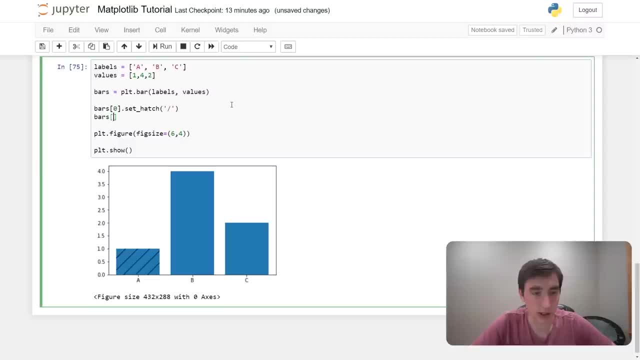 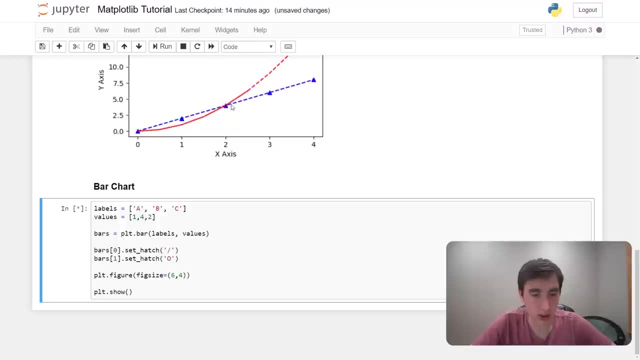 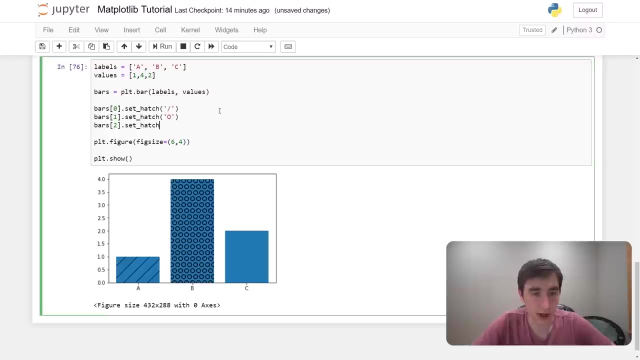 the lines that you see down here. I can do the same thing with the second value. Let's make this circles, And you can find all the hatch values in the documentation as well. Let's do the third value. We'll do stars. 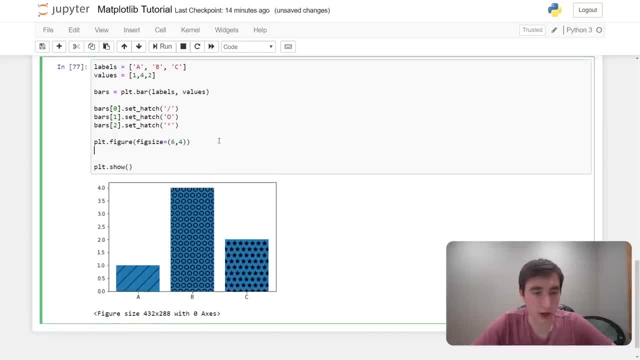 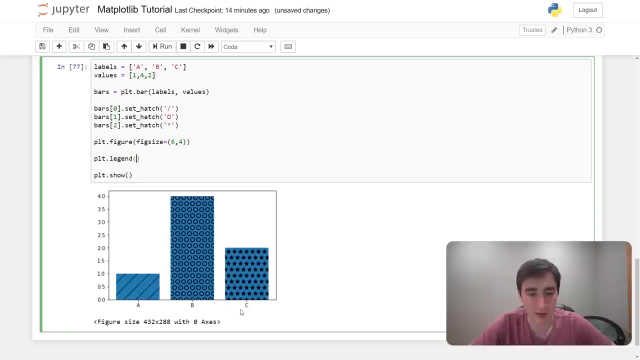 So now you get kind of a cool little bar chart. I can also add a legend to this very easily And this will tell me right away that we have A, B and C. But I mean, they're labeled right here, So legend is probably not necessary in this case. 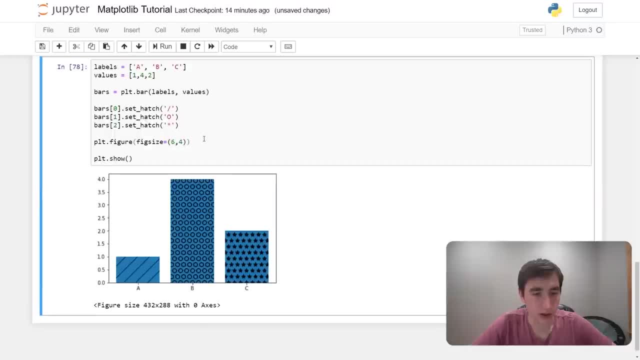 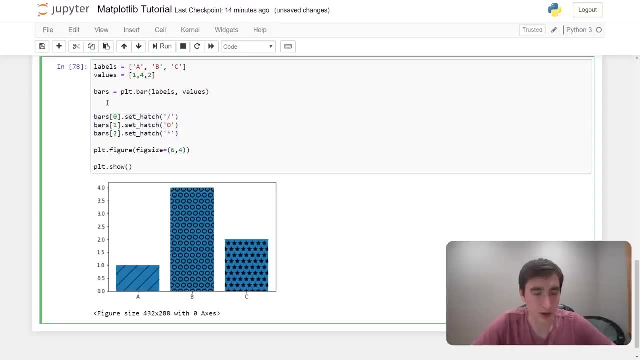 All right, Let's see What else did I want to do with this. And then, if you wanted to make this a little bit neater, if you had like many more, it might get tiring to do this. So you could do something like: